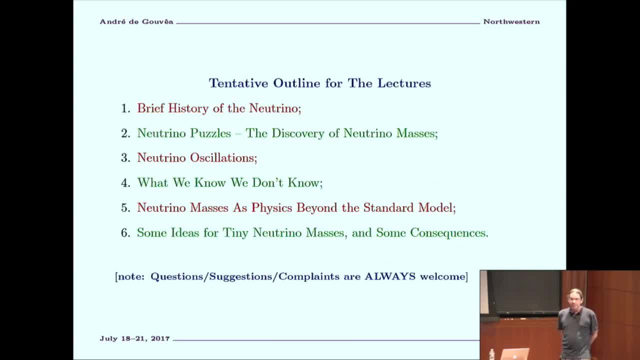 puzzles that plagued particle physics for the last 50 years or so, and they were eventually resolved at the turn of the century. And then, of course, the physics that's responsible for resolving this is the fact that neutrinos have non-zero masses, and they undergo this. 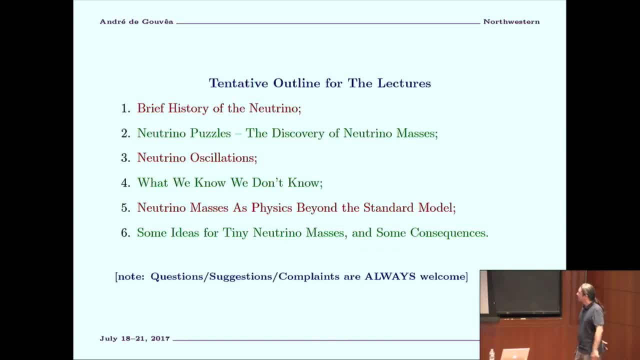 phenomenon called neutrino oscillation. so I will talk about that a little bit, And then I'll give you a snapshot of where we are as far as understanding this phenomenon as concerned, and I will try to convince you that that's what drives a lot of the experimental. 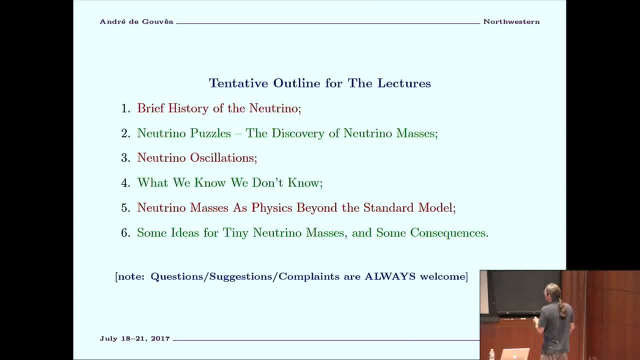 efforts that are going on today. Then I will move towards more theoretical things, towards the end and trying to convince you that neutrino physics are an interest- I mean, non-zero neutrino masses are an interesting discovery because they force us to revisit the physical world which, to be honest, is 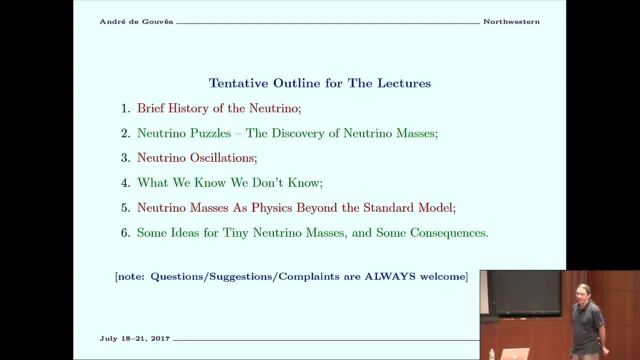 revisit some of the things in the standard model that we thought were correct and asking ourselves: how are we supposed to be modifying this model in a way to accommodate non-zero neutrino masses? and then I'll try to discuss some of the model building that comes along. 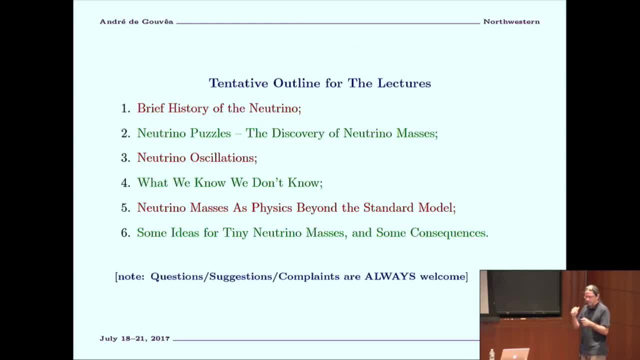 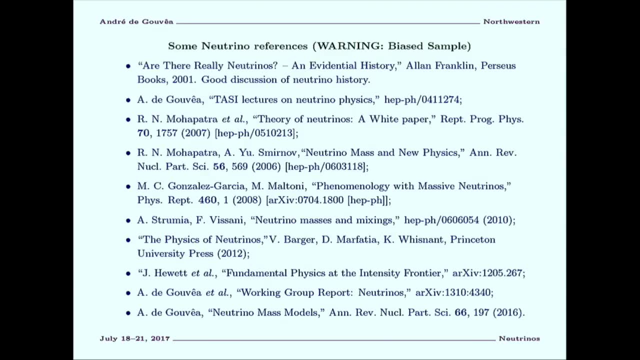 with that and hopefully just to give you a sense of what it is that people who do a lot of research on neutrinos concentrate on. So, because this is going to be available to you, I try to come up with a very biased list of reviews that people have worked on to give you a sense of neutrino physics during the 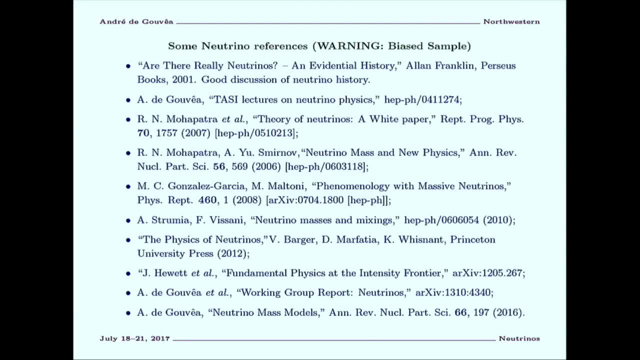 last. I guess this is getting old now, so this is about, say, 15 years or so, and it does give you a sense of how quickly this field has been changing. And one thing which I hope to convince you of is that if you follow the history of the 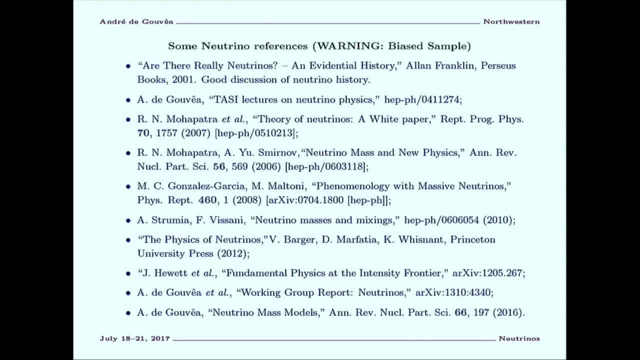 neutrino things usually change very, very, very slowly. So progress comes every other decade or so and somehow we're entering, or we've entered, this era. This is no longer the case, which makes a neutrino physics particularly exciting today. 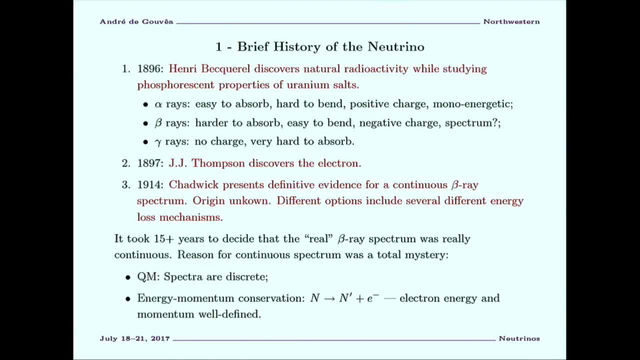 So let me get started by reminding you of the history of particle physics in the 20th century. A couple of warnings: This is a highly selective list of topics. There are lots and lots and lots of important historical facts that I will omit. 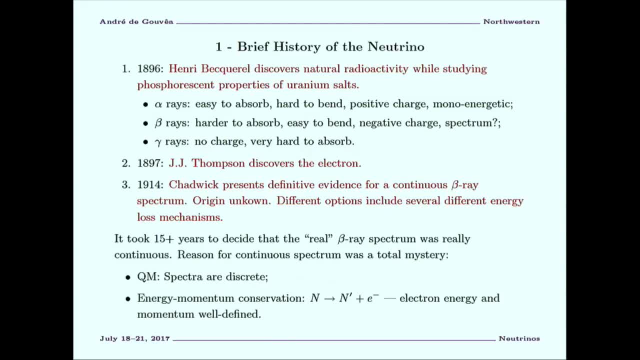 I am quite sure that there'll be lots of things which I'll say which are wrong, but they are correct in spirit, so hopefully that will be good enough. And again, you know this is a very biased list of history, but let's start out. 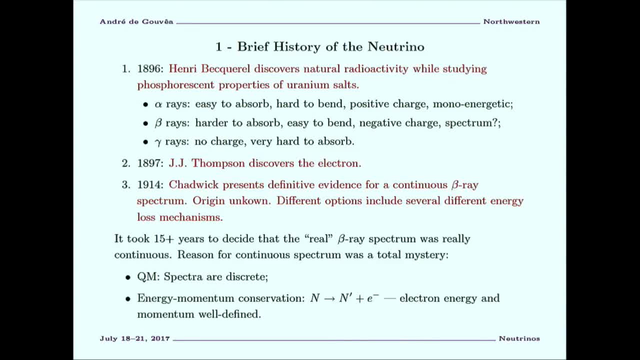 For neutrino physics, the most important thing that happened in prehistory was in 1896, when a natural radioactivity was discovered. This is one of these great stories in physics, which may or may not be true, but I'll tell you anyway. 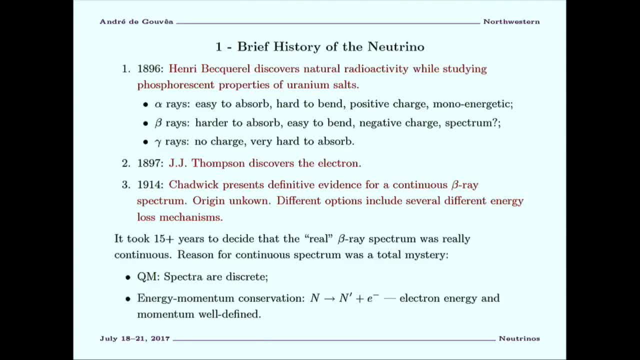 And so natural radioactivity was discovered by Henri Becquerel, who was doing studies in phosphorescence in uranium salts, And the idea is pretty simple, especially if you're a theorist: You take this uranium salt, you expose it to light and then you figure out that it. 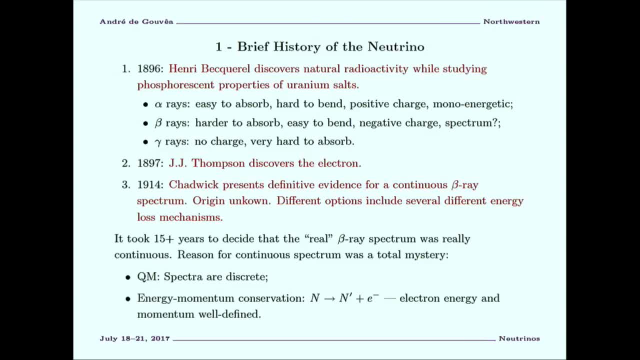 shines light after you've done that. So people were intrigued about how that happened, so they were making measurements of that And the story goes- and this is the part which may or may not be true, but it doesn't matter- that he was doing these experiments and at one point you know he had to do some experiments. 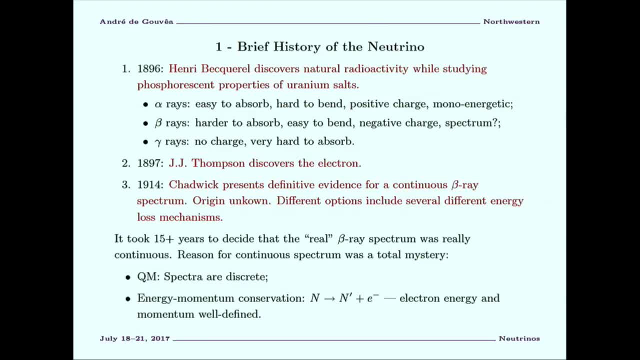 of phosphorescence. I think he lived in Paris. The weather in Paris is horrible, as many of you might know, So he couldn't do the experiment on a particular day, So he took his samples, he put the samples away in a drawer and he had to go on a trip. 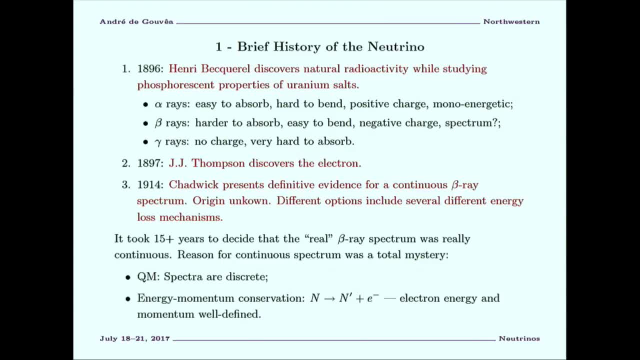 So he came back from the trip and a long time later he remembered that, hey, I have this sample that I put in a drawer. I don't know if it's any good or not. So he opened the drawer and the way that they did experiments back in those days was: 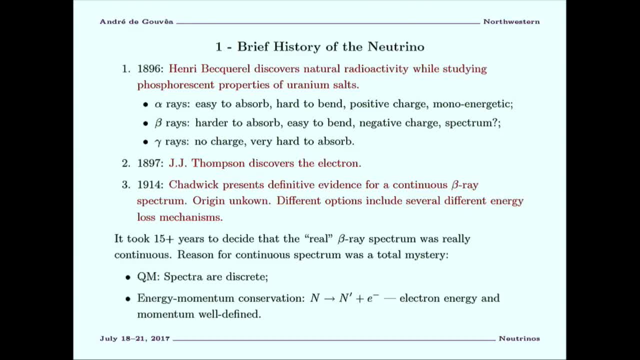 with photographic plates And basically what he did is he had this photographic film and he put the uranium salts on top of that And so he opened the drawer. Everything was kind of old, So he had this photographic plate and he decided to develop that. 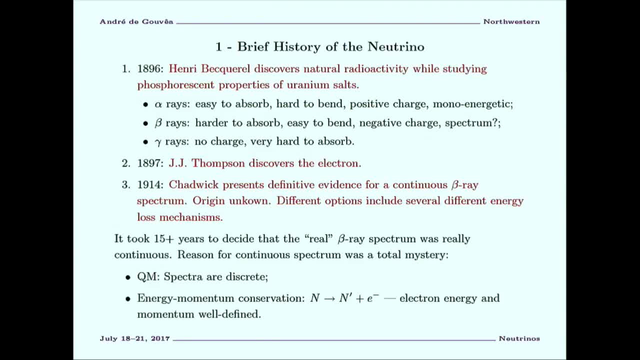 This is actually. that part is true. There's pictures of this. So if you take the photographic plate and you develop that, he noticed that where the little box with uranium salts was sitting on actually had left an imprint in the photographic plate. So that was odd because it wasn't supposed to do that. 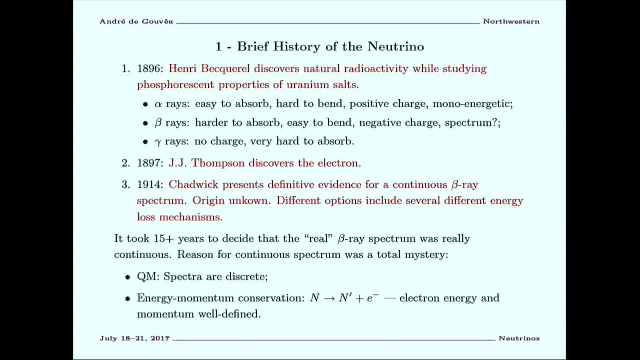 So of course he repeated the experiment, this time on purpose. so he put the little piece of uranium, You know, on top of this photographic plate. He left it there for some time. He developed the plate and he found out that for some reason uranium was emitting this. 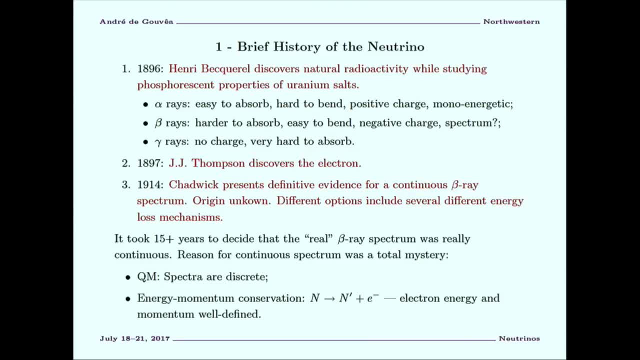 magic thing that was leaving an imprint in the photographic plate. So this is a discovery of natural radioactivity And, of course, immediately after that, people started doing lots and lots of experiments just to figure out what was going on. So what is this radioactivity? 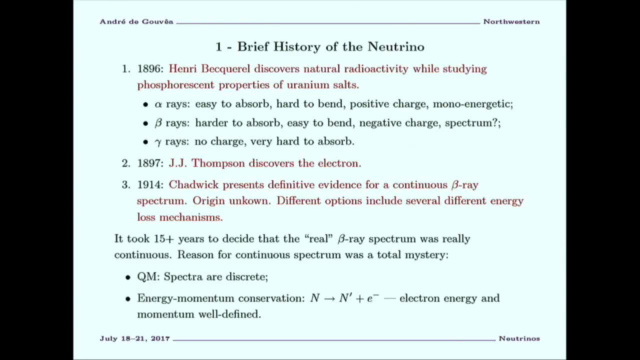 What does it look like? And if you're doing an experiment, you know and you found something. You found some new form of energy that's being emitted from a piece of material. You start asking questions about that energy, And that's exactly what these people were doing at the turn of the 1800s to the 1900s. 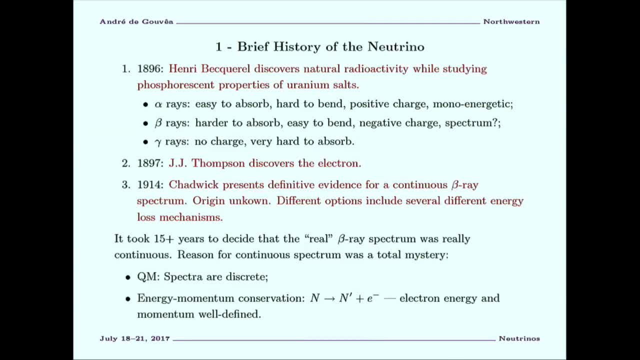 And they could ask very simple questions of the radioactivity. So that's what they did. So one thing you can ask is: does the radioactivity that comes out of this piece of material have a sign, as you know, related to charge? 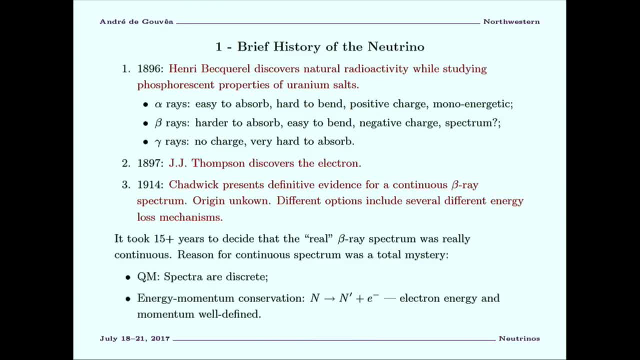 So is it charged, And that's easy to test. You make a sample where you can emit the radioactivity in a particular direction. You place that in a magnetic field and you see if it bends, for example. So that's one thing you can try to measure. 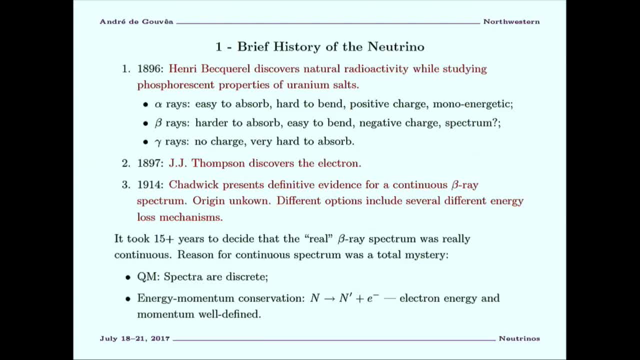 The other thing you can try to measure is you can measure the properties of the radioactivity by asking: how hard is it to contain the radioactivity? And that was actually the first zero-torder thing that they did And they found out by doing these experiments. 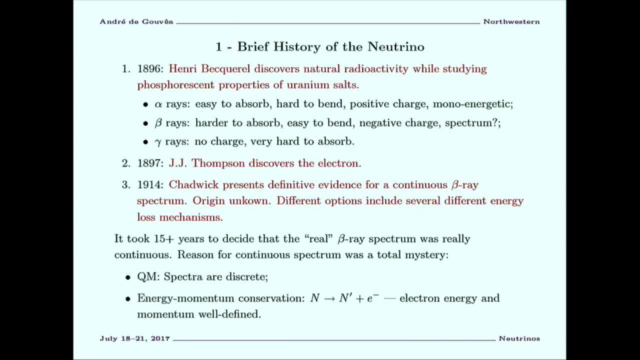 They did experiments with lots of different materials, that there are three kinds of radioactivity if you classify them by how hard it is to contain the radioactivity. And of course they gave these things names alpha, beta and gamma, for completely obvious reasons. 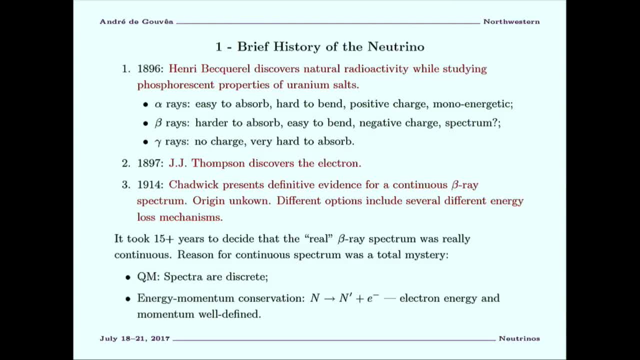 So there's no mystery between these names. There are three kinds. You know it's A, B and C. But you don't want to use A, B, C because that's boring, So you use alpha, beta and gamma. 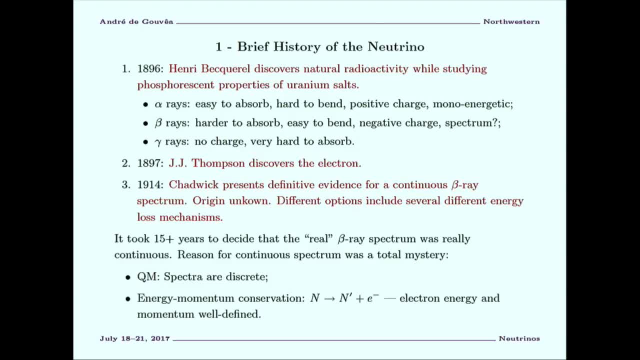 And of course, alpha radiation, as people know very well, is very easy to absorb, And people also figured out that alpha radiation actually has positive charge. Beta radiation, on the other hand, is a little bit harder to absorb. That means it's harder to contain. 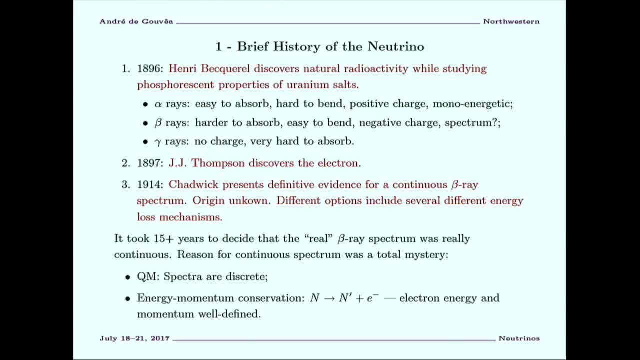 So again, the idea is you do the experiment, You put the piece of material here, You put a detector here And then you put a barrier in the middle And if it's easy to make the radioactivity not get to the detector, that's easy to absorb. 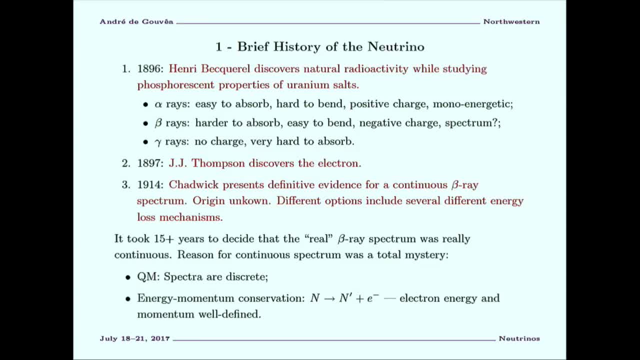 If it's a little bit harder, it's a little bit harder, And if it's really hard, it's really hard. So that's the idea. And you know alpha radiation, as you might know or you should know, you can kind of 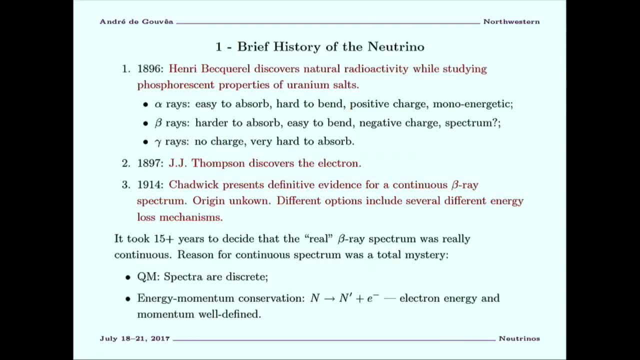 stop it with a piece of paper. You cannot do that with beta radiation. You need a little bit more material for that, And gamma radiation is even harder to stop. So that's how they were originally classified. People then also figured out that beta radiation had negative charge for all of the stuff that 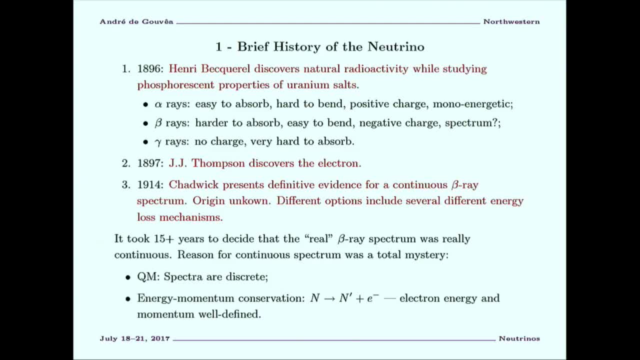 they managed to study at the time And gamma radiation did not have any charge and it was the thing that was hardest to stop. This is kind of step zero of studying this natural phenomenon of a natural radioactivity. You can do more sophisticated experiments by asking. 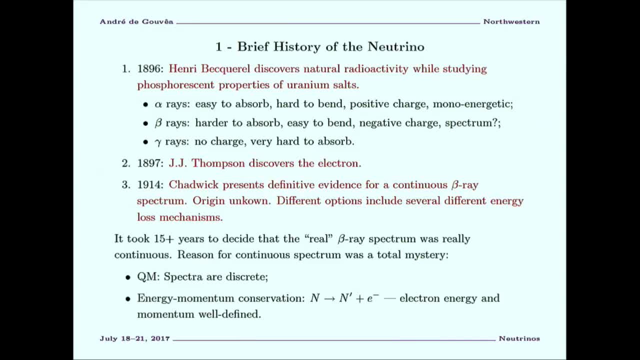 And before I talk about that, let me remind you that this is in 1896. At this time we did not know of any fundamental particles. That took one year. In 1987, the electron was identified as a thing, as a particle, by studying a cathode. 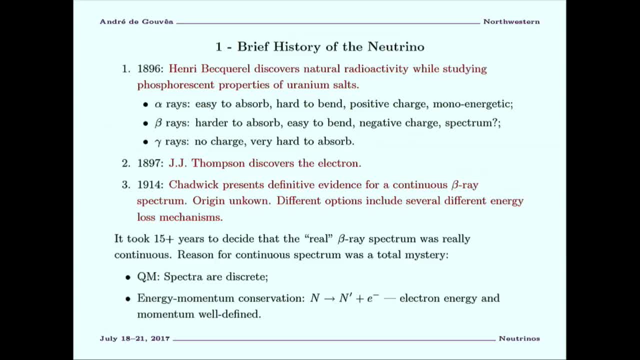 rays And these are tubes that people put an electric field on And you saw stuff moving one way or the other And you could see the electron moving one way or the other. So the electron was discovered here. But going back to the radiation, people could also study the energy of the radiation. that 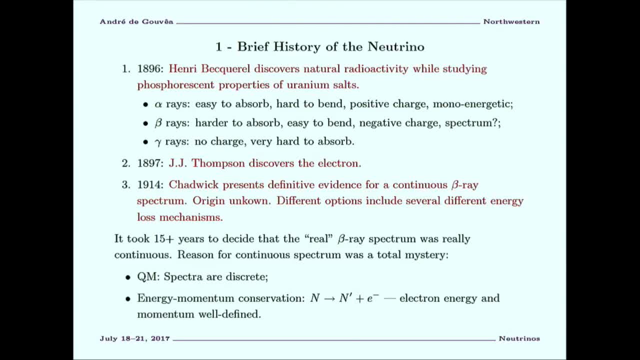 comes out And you can kind of understand how you would do that, certainly for alpha and beta radiation, Because you can take the radiation, you can place it in a magnetic field and the bending in the magnetic field will give you some information on the momentum of the thing that's coming. 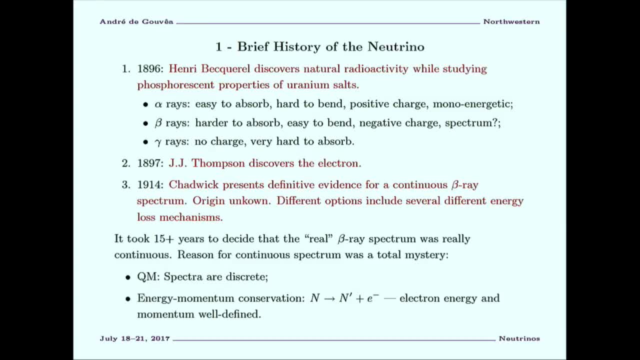 out. So by studying that people figured out a couple of interesting things. For example, alpha radiation usually comes out more or less monochromatically. Beta radiation will come back to, And then alpha radiation was harder to measure the spectrum, But people figured out how to do that later. 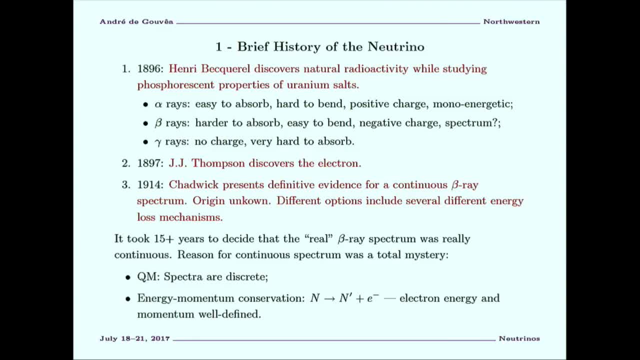 OK, So our job is to talk a little bit more about beta radiation And again, it's important to keep in mind what was going on at the time. In the 1900s, we didn't know quantum mechanics existed By 1910, we had learned a little bit about quantum mechanics and we were very, very 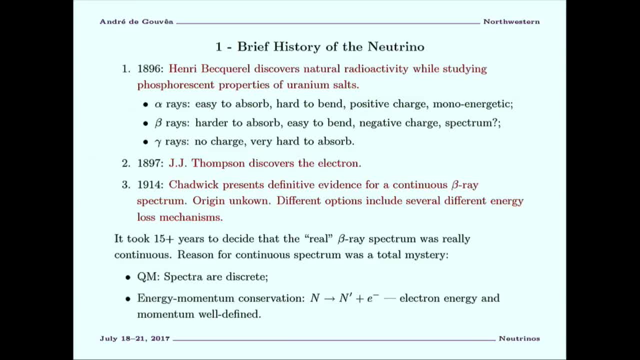 confused. OK, So that's sort of where we are, And one thing that was going on with beta radiation is people were trying really hard to measure the spectrum of beta radiation. If you read the histories associated to that, this is a very, very confusing time in our 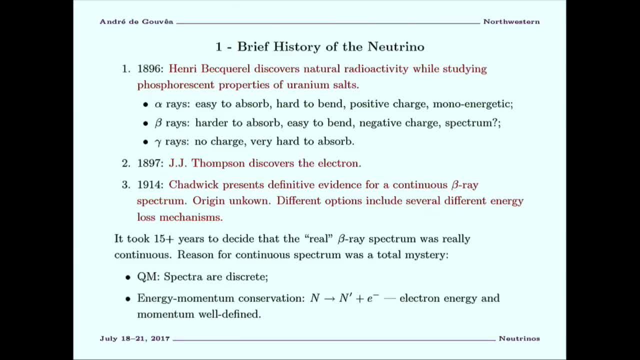 understanding of radiation And you probably know a lot about beta radiation And you know that the end result is beta. OK to the discussion is that the spectrum of the radiation that comes out is continuous, So a beta radiation happens. you get this beta ray, which now we know is an electron. 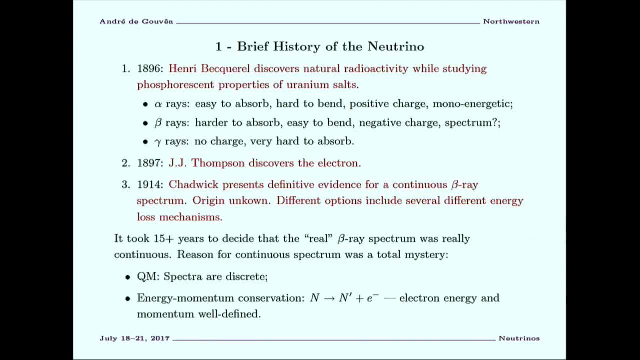 and that electron has a continuum of energies. People did not know that for a very long time. So it's only in 1914, so about almost 20 years after radiation was discovered to begin with- that somebody did a set of experiments that established beyond reasonable doubt that 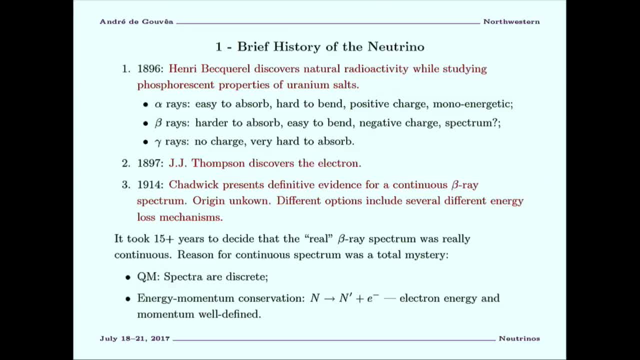 the spectrum was continuous. Okay, so that was a fact, and it took a long time to establish that fact. Now, this was very, very confusing. When they figured out that the spectrum of beta radiation is exactly continuous, they were surprised, and that's why it took people. 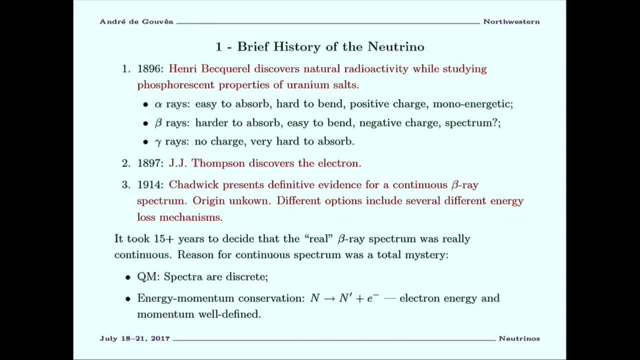 a long time to convince themselves that this was actually correct. And there are lots of reasons to be surprised, and I will mention the two obvious ones. The first one is the following. One is that this was clearly a quantum mechanics phenomenon and if you remember the old history, 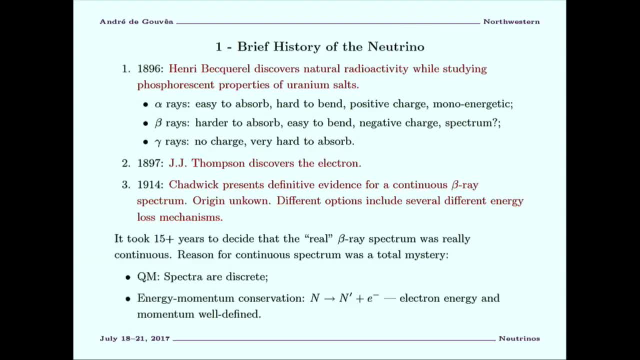 of quantum mechanics. usually, when you have spectra of radiation coming out from some physics process, like say atomic lines, you get these discrete spectra. Actually that's where the word quantum comes from. So this one looked different. so people were: 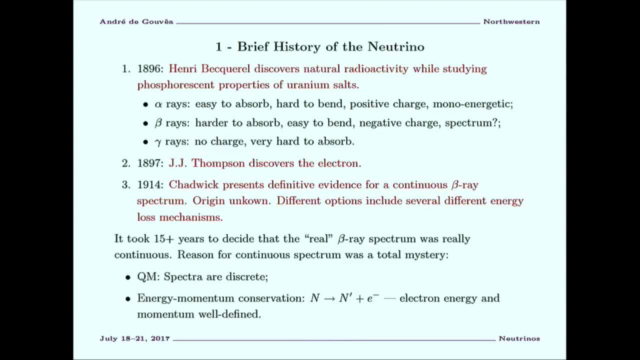 puzzled by that. A more serious concern, of course, was energy momentum conservation. So you probably know the story. You know after we learned a little bit more. you know before we knew that this process could be properly defined as some atom that was converting. 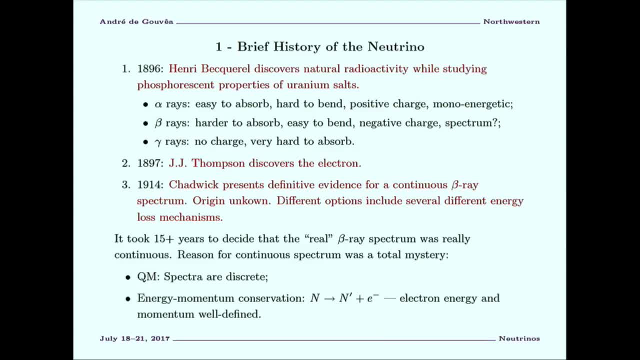 into another atom, usually an ion, because you lost charge and then an electron was emitted. So, regardless of what's going on over here, you can appeal to the conservation of energy and momentum to make a prediction, and the prediction is that this electron, that 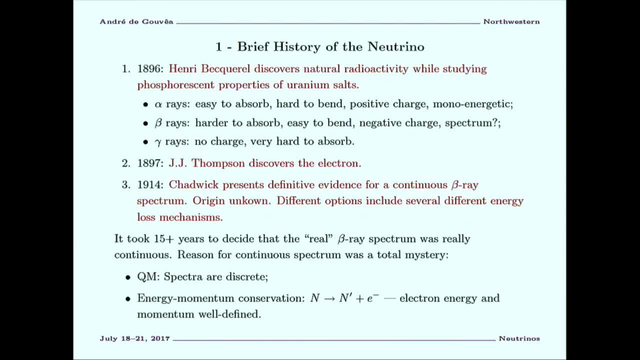 comes out. you know the beta radiation that comes out has a very well-defined energy and momentum. You can calculate it. You don't have to know anything about the interactions or what's going on in order to predict very, very strictly that this electron has to come out with a 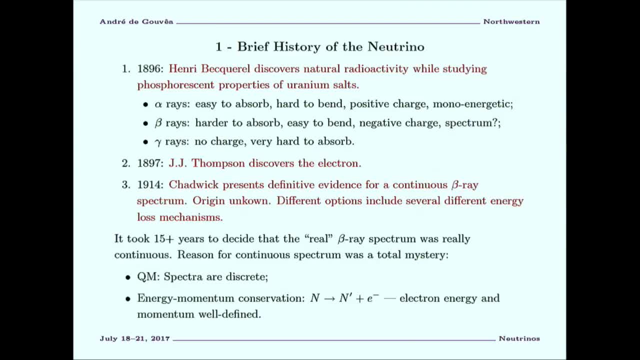 well-defined energy and momentum and you could calculate that. And just to give you a sense, right over here I will draw a beta spectrum And keep in mind this is similar to the, you know, rotation curves of galaxies. So here's the beta spectrum that you predict. 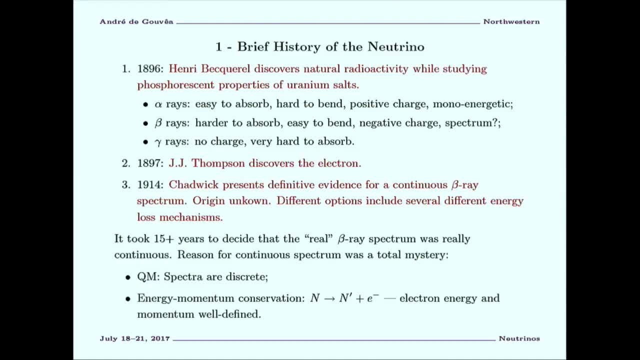 It's a delta function over here. Here's the beta spectrum that you measure And here's the beta spectrum that you measure. It looks like that Completely different. So that's bad. So, of course, very, very smart people spend a very, very long time thinking about. 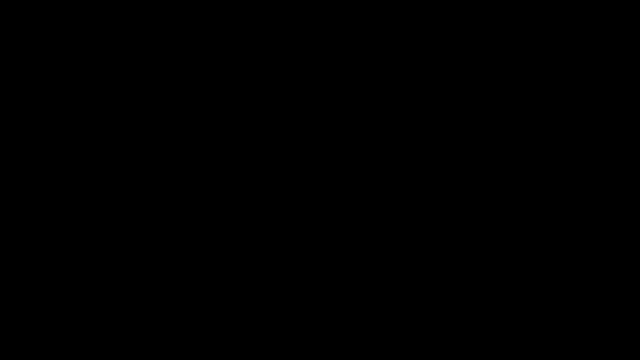 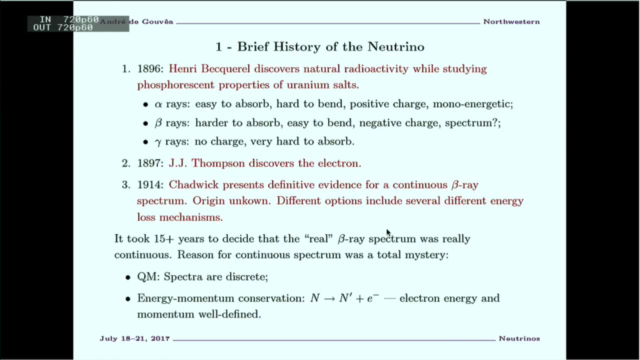 this. There are lots of – did I do that? Did I do something weird? I probably did So, let's see. Ah, thank you. So if this is what's going on, then the first thing that you think about is that somehow there's an energy loss mechanism in the system, Right? 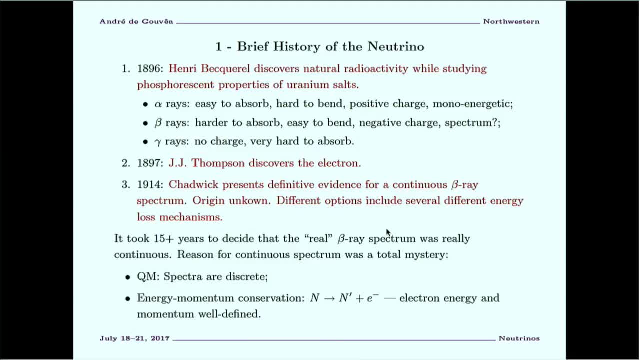 You've produced an electron, It has to come out of the material, So somehow it's losing energy as it's trying to do that, And that was one good explanation. Curiously enough, that was refuted as a good explanation by experiment. Don't ask me how they did that. 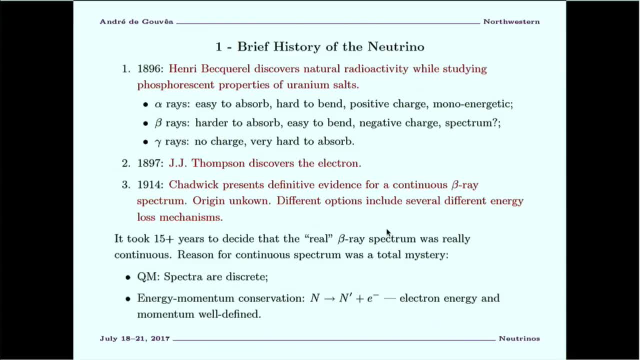 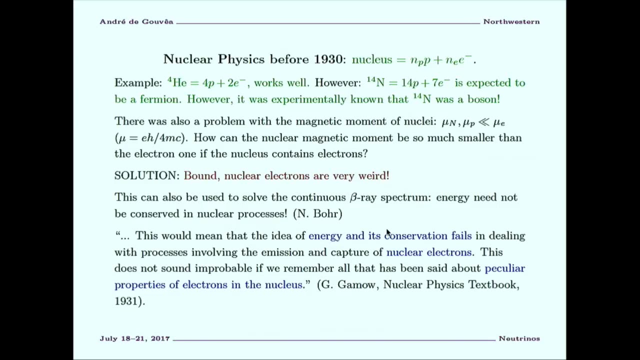 It's not very easy. It has to do with you being able to measure whether the material, as the beta radiation, is coming out, And that was not being observed. So let me make a brief pause to tell you of what was going on, say in the 1920s as far. 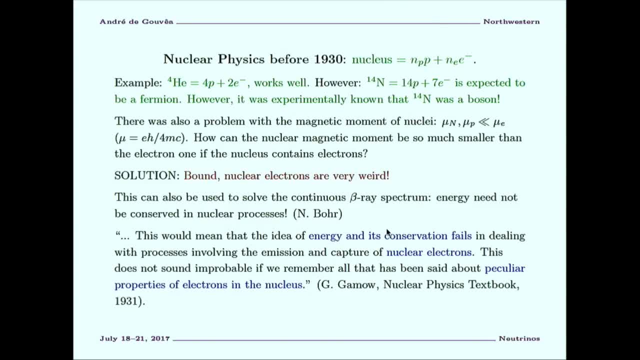 as understanding nuclear physics. So first of all, let me remind you that nuclei were discovered And we had this- quote unquote- planetary model for atoms, which is very successful. So now the next job was to figure out how nuclei are formed, And here's the model of: 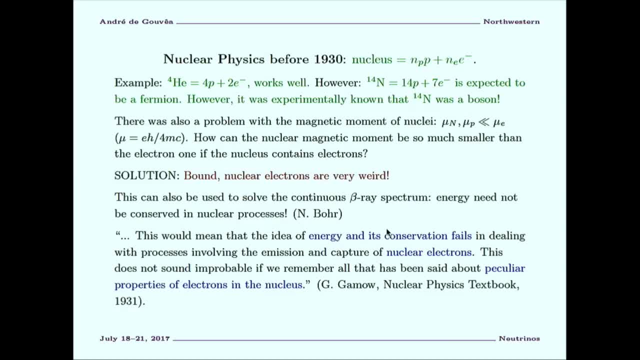 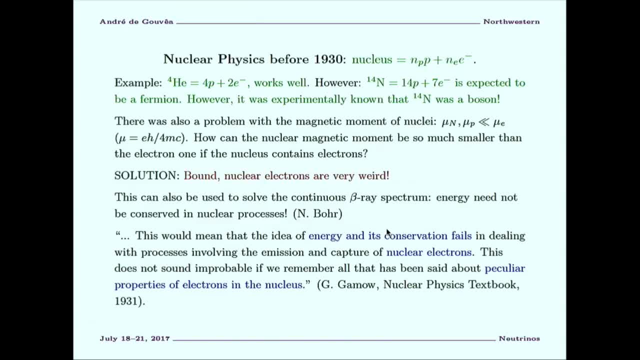 protons and electrons. Most of the mass comes from the protons and the electrons are there to make the charge work out. So this is the model And with this model you can make a lot of predictions. So, for example, helium-4 is four protons and two electrons. That works. 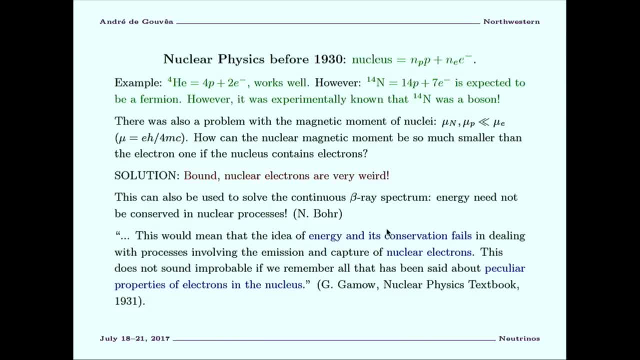 ridiculously well. But then people started running into other problems. One problem is very simple to understand. Here's nitrogen-14, which, according to this model, is made out of 14 protons and 7 electrons. Again, it's a good prediction: You get the. 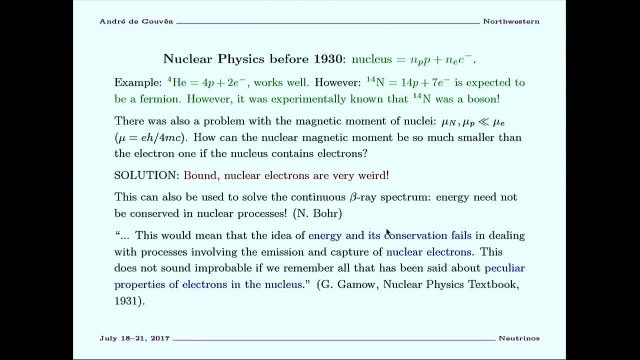 mass right, But there's a big problem. It turns out that nitrogen-14 is experimentally determined to be a boson. This thing, whatever it is, is a fermion. It's not the same thing. So clearly there's something going on, because you made a prediction that nitrogen-14 is 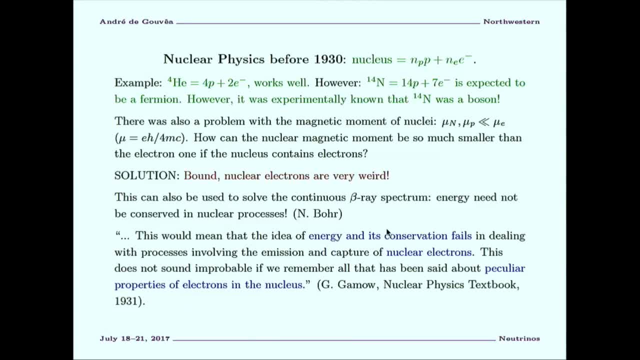 a fermion and you do experiments and it's a boson. That's a very big difference. There's actually another funny problem with this model, which is it has to do with magnetic moments, And people have started measuring magnetic moments and they figured out that 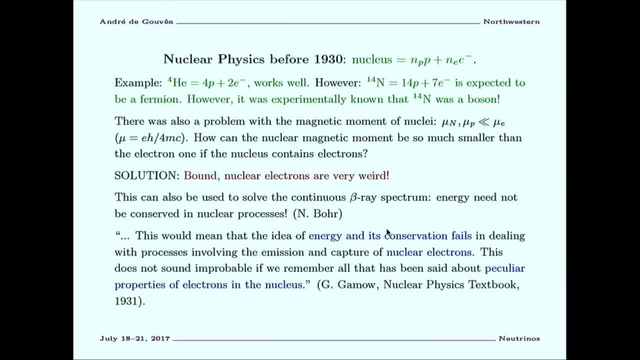 nuclei have magnetic moments as well, And you can quickly convince yourself, with everything that you know about magnetic moments today, that the electrons in the nucleus are the most important elements in the system, And so you can clearly see that the electrons electromagnetic moment is actually much bigger than the magnetic moment of nuclei. 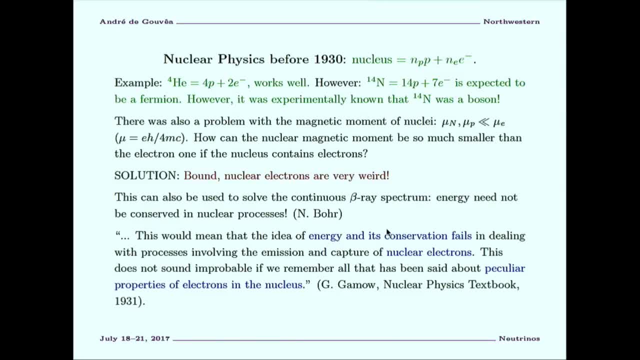 That sounds very puzzling, because you're postulating that your nucleus is made out of a lot of electrons and somehow the contribution of these electrons to your magnetic moment cancels out, because otherwise you would expect the magnetic moment of your nucleus to be. 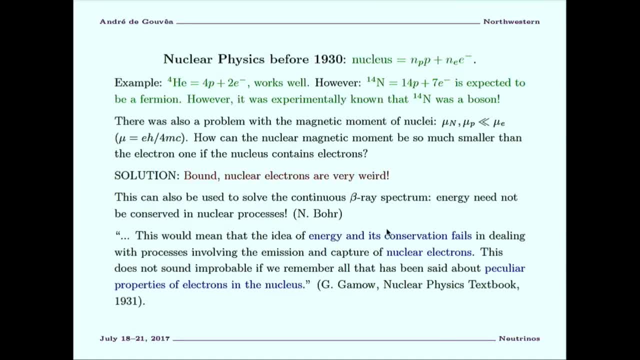 mostly of order, the electron magnetic moment, and that turns out to be wrong. So these are all these problems that people were running into with our understanding of nuclear physics in the 1920s and the solution to this, and this is the best thing, people, 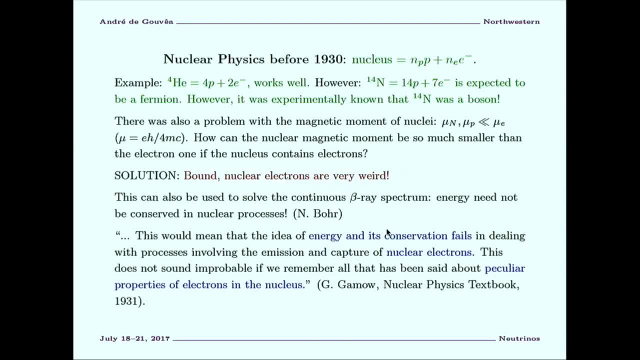 could come up with is summarized here, is that people figured out, or they postulated, that these electrons that live inside of nuclei are just very, very weird And you can say no, nobody would say that. but of course the smart people said that. 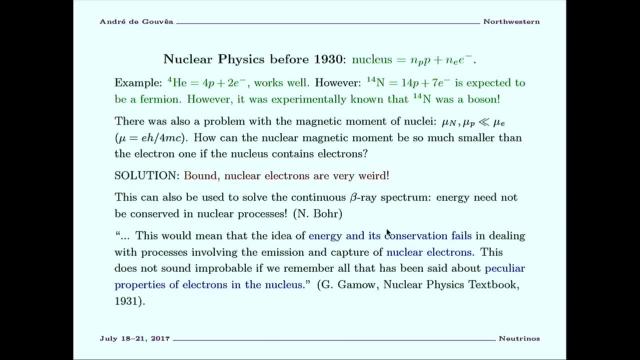 and they took advantage of this. they say: hey, nuclear electrons are weird and maybe that explains the beta radiation. Maybe they're so weird that they don't have to conserve energy and momentum, for example. This is a quote from Niels Bohr and it says that, you know, maybe energy is not conserved. 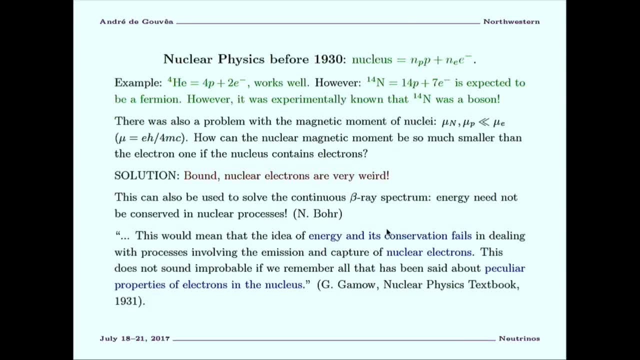 in the nuclear physics processes. And again, another thing which is important to keep in mind in this historical context is that this is a textbook on nuclear physics written by George Gamow in 1931, and it contains this sentence here. Gamow, by the way, was sort of a funny guy, so this is consistent. 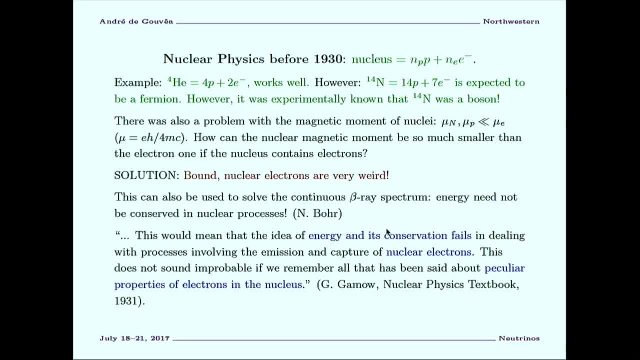 But he says, you know, blah, blah blah. this would mean that the idea, the idea of energy and its conservation, fails in dealing with processes involving the emission and capture of nuclear electrons. This does not sound improbable if we remember all that has been said about the 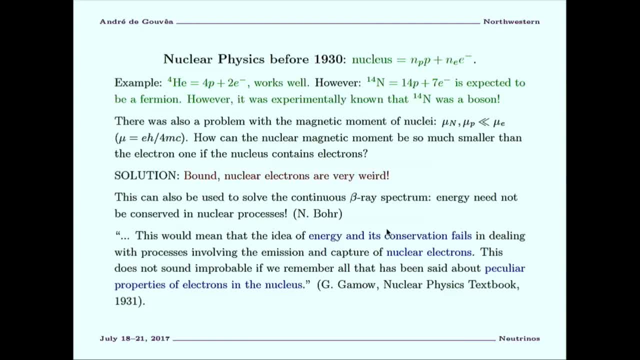 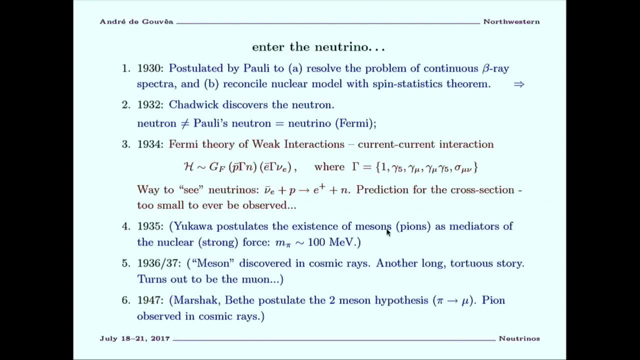 peculiar properties of electrons and nuclei. So it was an interesting road that people were going down through, and all of that changed in 1930. And, of course, this is a story that I assume 100% of you have heard before, at least once. 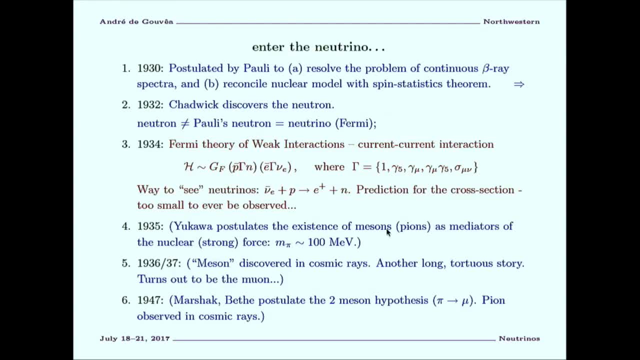 But I will tell you the story anyway, because it's a great story. So the idea is that in 1930, Pauli postulated a different solution to all of these problems, And it was a very simple solution. So basically what he said was he had a solution that solved both a lot of the nuclear physics, 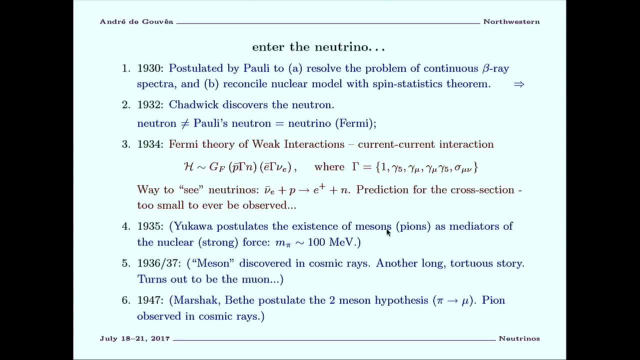 issues that people were concerned about. but it also solved this continuous beta-ray spectra, And you know the story that's very well known is that this was actually not published as a paper. It wasn't even published as a proceedings in a conference, because this is a conference. 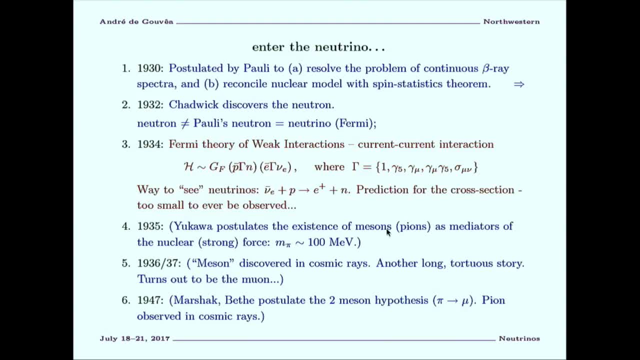 that Pauli didn't attend because he couldn't make it. It was a paper, He couldn't make it, But he actually sent a letter to the participants in the conference with his new idea And he asked his friend to go to the conference and read it for him in the conference, which 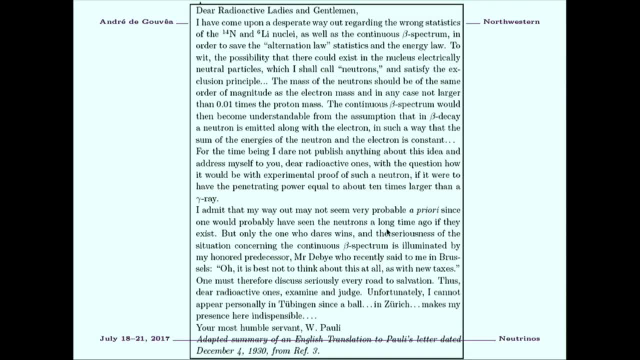 apparently is how it worked out back then, And this is a translation of Pauli's letter. It's a very short letter so his friend didn't have to be embarrassed for very long, But this is a really interesting letter that has lots of interesting features to it. 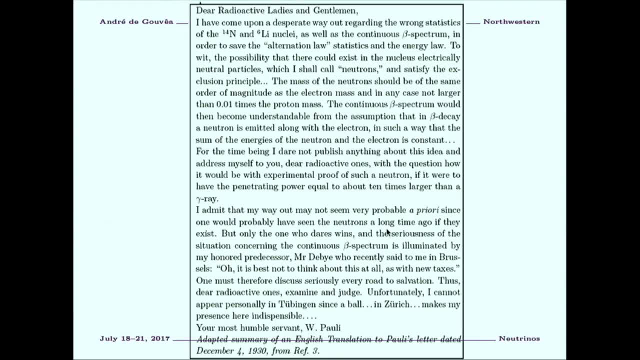 So he starts out by laying out what the problem is. He says: hey, we have this problem with the spin statistics theorem and a couple of nuclei that have been measured very well. Remember, this is Pauli. He invented the spin statistics theorem. 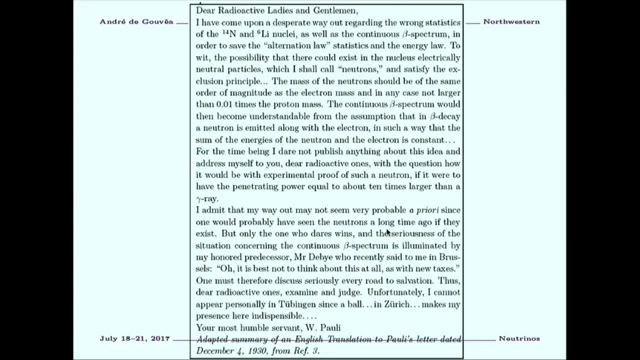 So he cared about it very much, I suspect, And also this continuous beta spectra. So blah, blah, blah. Lots of things are going on And he says, in order to solve all of these problems, I'm going to invent a new particle. 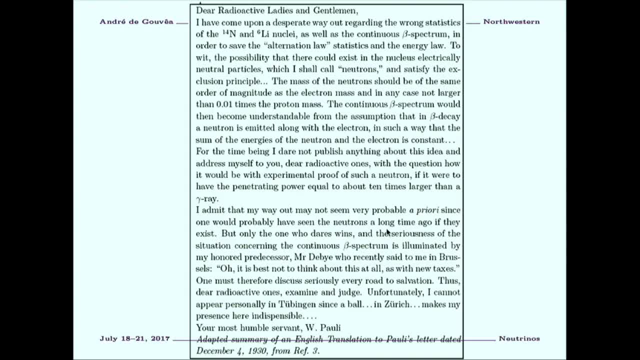 So he invents a new particle Which he says also lives inside of the nucleus And that particle better not have any charge because those properties of nuclei were working very well. So we don't want to screw that up. So he called that particle a neutron. 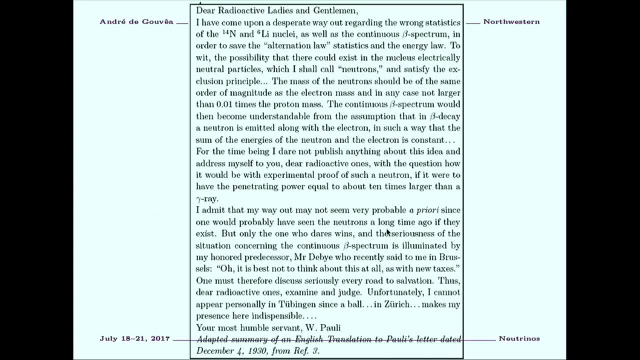 Now he also said so. he did some phenomenology, So I'm inventing a new particle. What properties must this particle have so that it fixes the problems that I'm trying to fix and hasn't been discovered yet? So that we do that all the time? 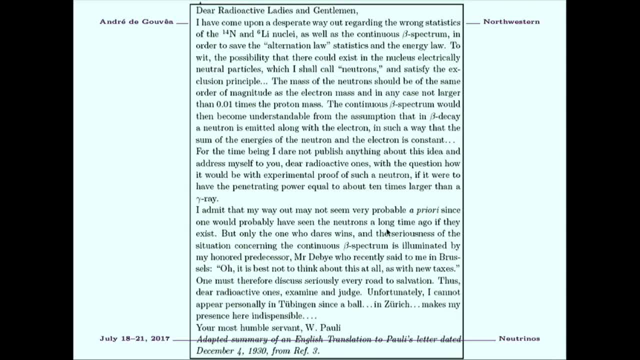 That's sort of how we make a list. That's what I'm living nowadays. And so he said: you know, so it has to be a spin, a half particle, So it satisfies the exclusion principle. So if you add enough of these particles, you can choose whether things are going to be. 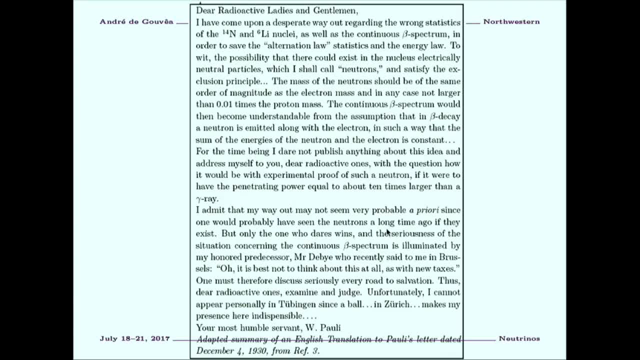 bosons or fermions. So that solves that problem. And you can solve the beta spectra in a very simple way If you say that the beta decay process is a three-body final state process. So the nucleus decays into another nucleus, an electron, and this neutron that comes out. 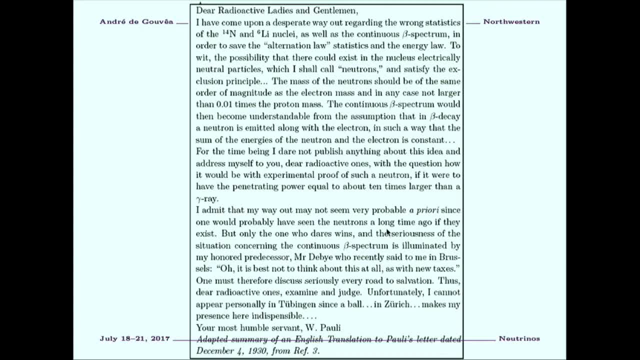 and that explains why you have this continuum spectrum, because the electron is sharing all of this energy with this other particle that's coming out. And then he did a little bit of numerics to figure out how heavy must this thing be, so that we've never seen it before. 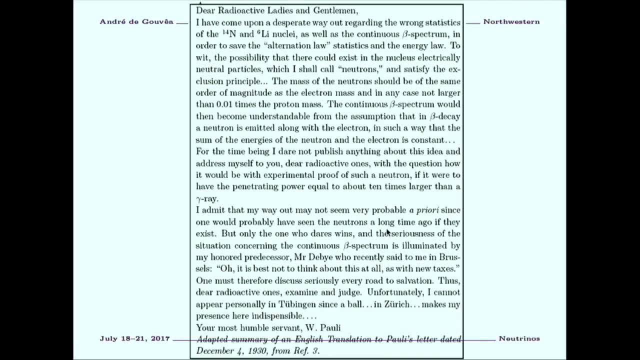 So he places an upper bound on the mass of this object, And then he also has to make some calculations about how come we've never seen this before, And that means that the penetrating particle, I mean the penetrating properties of this object, Have to be very good. 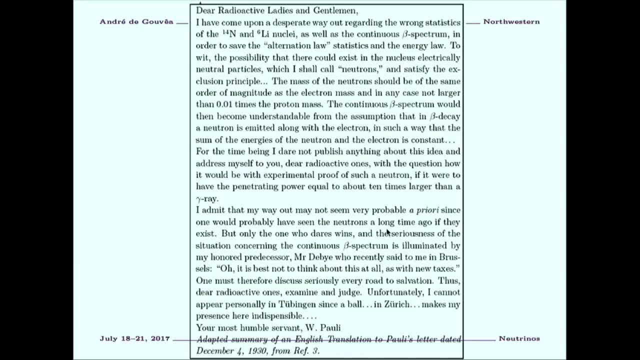 It has to be a very hard to measure particle. So that's basically all that he's doing over here in this first paragraph is laying out the properties that this particle must have in order to solve all the problems and not be observed experimentally. 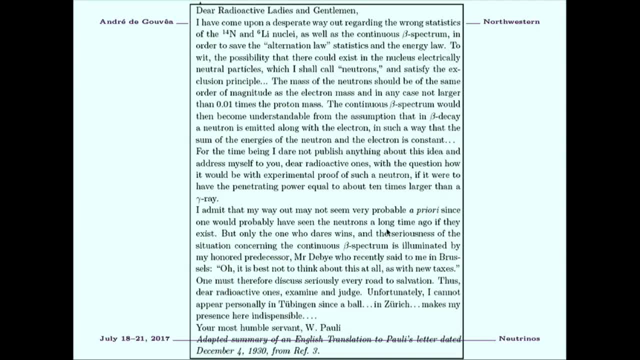 Then here he has some concerns. So basically what he says is he's sort of ashamed that he's invented a particle that nobody could detect and he doesn't like that. We've gotten past that. We can invent lots of particles that we can't detect and we don't have any qualms about. 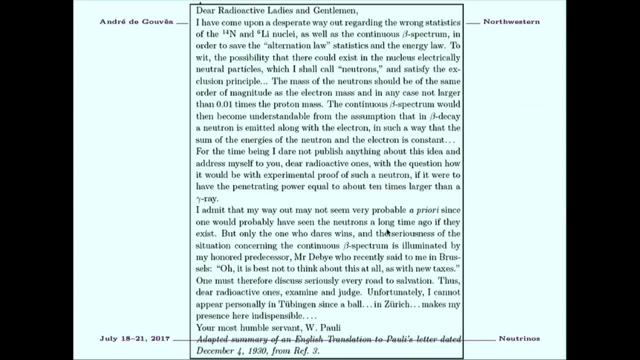 that. But then he has some funny sentences here about whether that's a good idea And he's saying it's a good bet to take, and so on. And finally he also explains why he can't go to the conference, because he had to go. 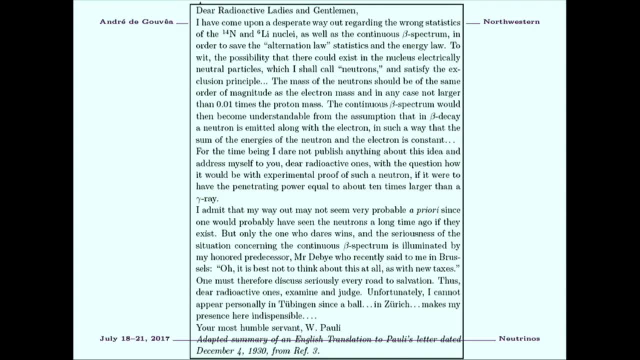 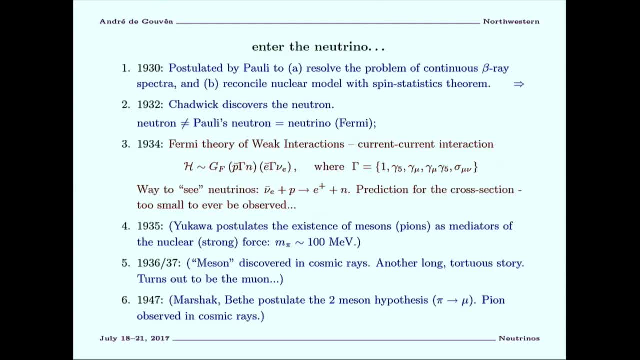 And lots of things happened right after that which are very interesting. I'm sorry this is in 1930.. In 1932, in England, Chadwick- who was one of these renowned experimentalists who had done a lot of work, he actually discovered a new particle that was neutral. 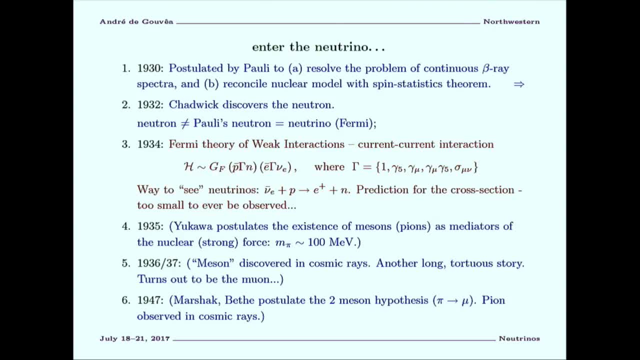 And he discovered it, It doesn't matter how. And he discovered this thing called the neutron, and that was a really big deal because it changed the way that we do nuclear physics, for example. So right away, the information percolates throughout. 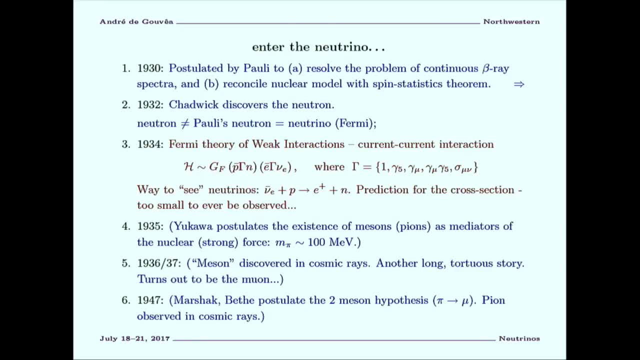 It's a very big discovery And I probably won't tell the story exactly right, but the idea is, then this got to Italy and Fermi was talking to some people about the discovery of the neutron And then somebody asked Fermi, hey, Chadwick just discovered this neutron. 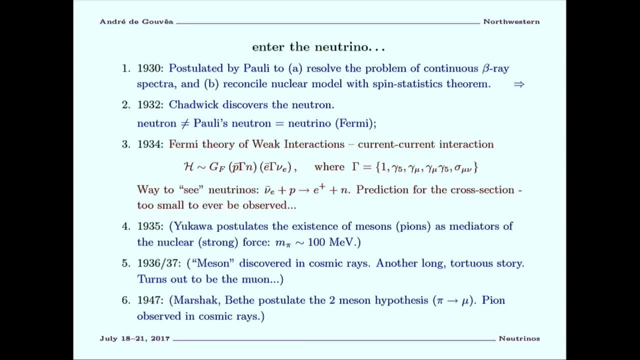 Is that the same particle that Pauli proposed? And then Fermi said: no, no, no, that has to be a totally different particle, because the particle that Pauli proposed is much, much lighter. So it's not a neutron. 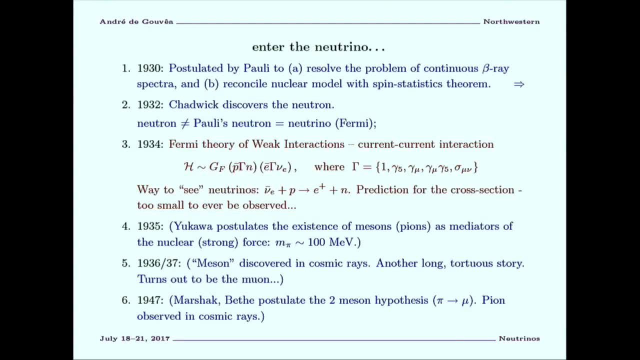 It's a small neutron, which in Italian is a neutrino. So Fermi did that and that's the name that the particle that Pauli invented got. And if you know Italian, eno means small. It's a suffix that makes things small. 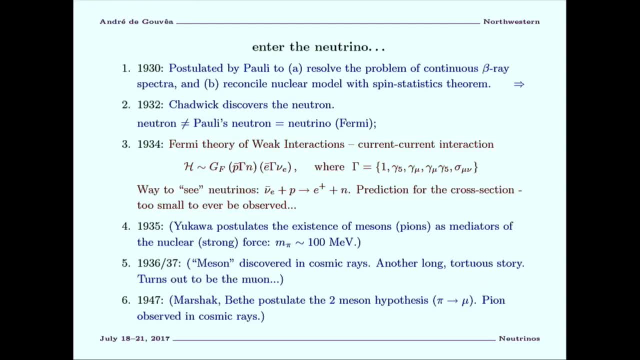 So this is a small neutron. To differentiate it from the big neutron, the name stuck, which is kind of interesting. It's also peculiar, But this Italian suffix eno was hijacked by the Susi people to indicate fermions. 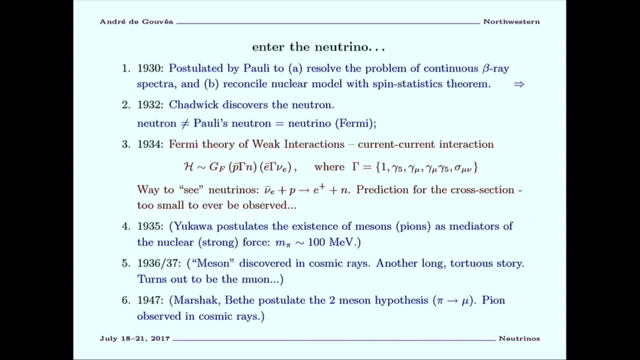 So you have hexenos and charginos and gravitinos and all these particles are in quotes, little gravitons and little charged particles and so on, except that they could be very heavy. Anyway, I'm sure the Italians were not amused, but they've gotten used to it by now. 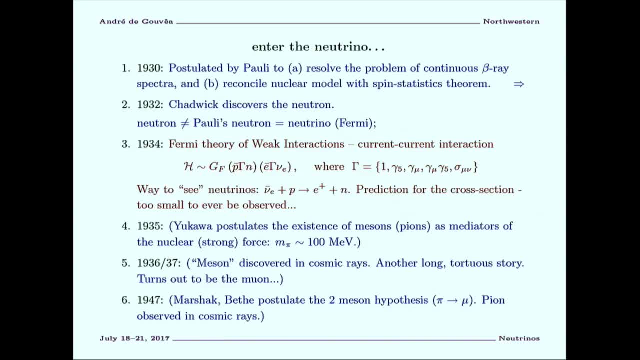 So this is in 1932.. In 1934, something much different, Something much more important happened. I mean again, when the neutron was discovered, the nuclear model started to be revised. It became much more sane to say that nuclei were made out of protons and neutrons. 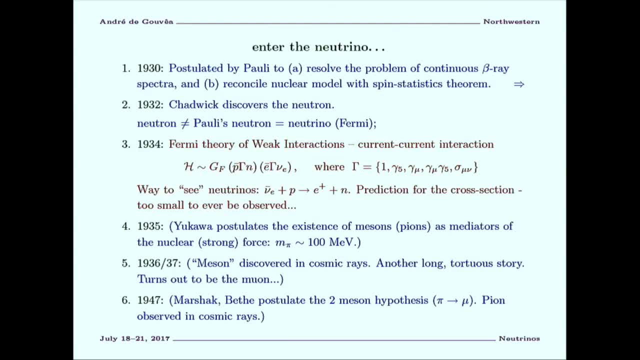 So you didn't have to have any electrons or neutrinos inside of the nucleus. But then what Fermi did is he wrote down the Fermi theory. And the Fermi theory is an amazing idea that uses information that people had from other descriptions of physical phenomena. 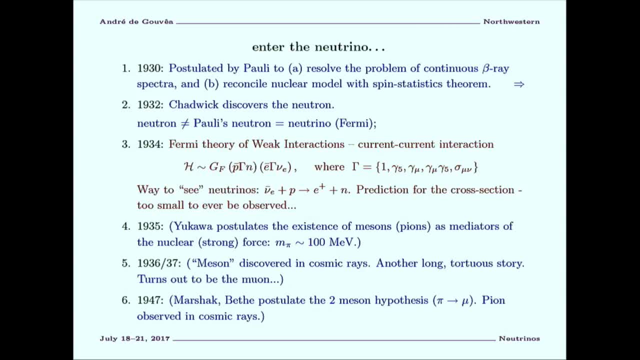 And basically what Fermi postulated was this: He wrote down the Fermi theory, He wrote down a theory for beta decay And he said: you know, we know how electromagnetism works. It's a current-current interaction. So if you want to do, say, electron-electron scattering, that's described as a current-current. 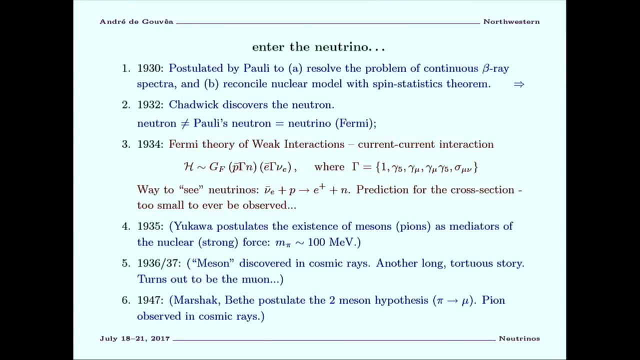 interaction. So I want to describe beta decay in the same way, except that I want to have some funny currents And I want to postulate that you can have a proton-neutron current and I can have an electron-neutrino current as well. 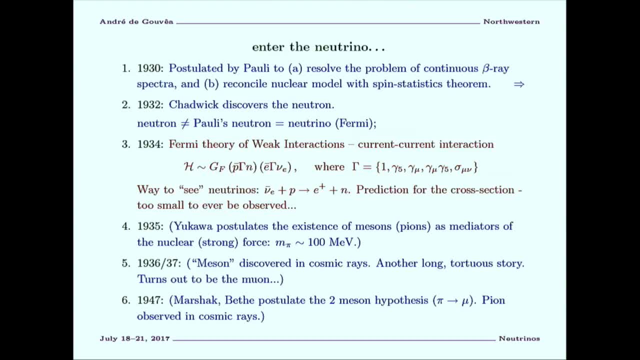 And I don't know the nature of this current. It doesn't have to be a vector current. It could be an axial vector current, a pseudo-scalar current, a scalar current, and so on. But he wrote down this theory here. 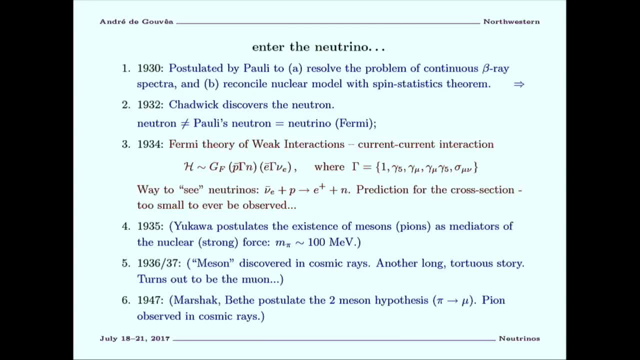 And of course, this is proportional to some unknown constant which is called a G, which we of course call the G-Fermi. There's also a funny story here- if you've ever done calculations using Fermi theory, is that there are always some annoying factors of a square root of 2 or 2 floating around. 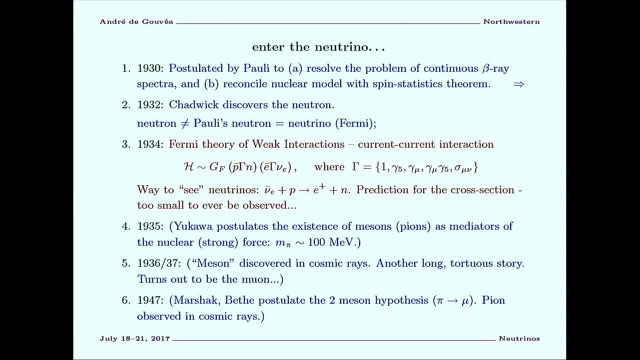 I think that has to do with Fermi's definition of the constant, which is not optimal for doing calculations. Anyway, so he wrote down this theory And this is an amazing idea that has lots of interesting consequences. Probably the most interesting consequence of this is that he allowed for the possibility. 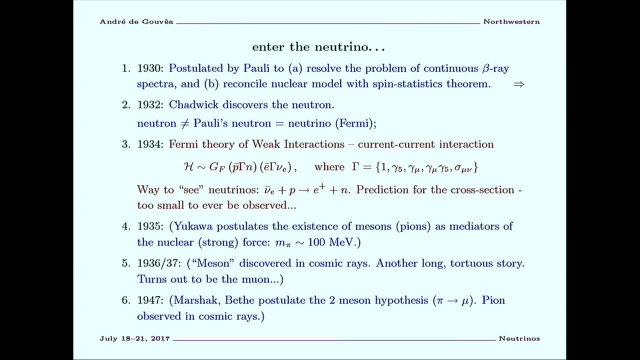 of particles turning into other particles. We already knew about the fact that you could create, say, photons out of nothing, which is a really weird idea, but we got accustomed to that. This is the first time where you could have one kind of particle turning into another. 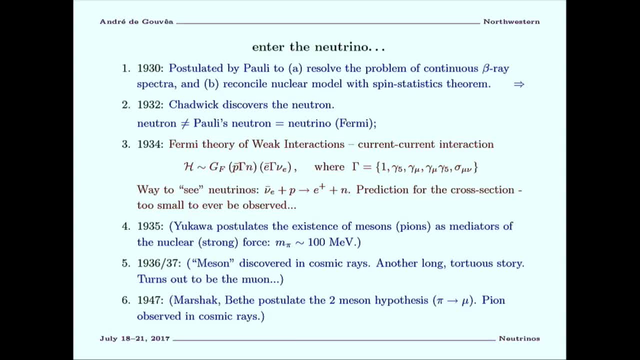 particle, So you could have a neutron turning into a proton and then having an electron and a neutrino pair appear out of nowhere, And that was OK. So this was first written down here And people again have grown accustomed to this. We of course don't even worry about that. 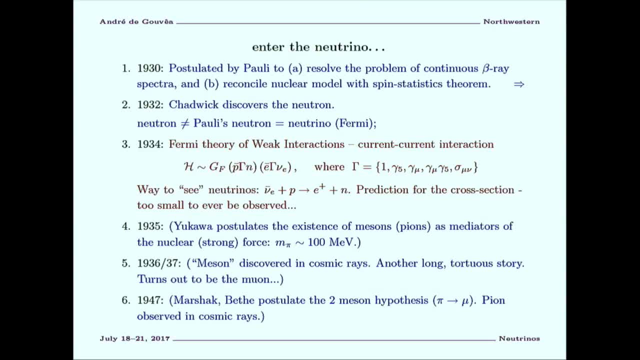 But this is probably really really weird, Because this makes very little sense from the point of view of what does a particle look like? What does a particle mean? Let's see. But the other thing that's very important is once you write down a theory that describes. 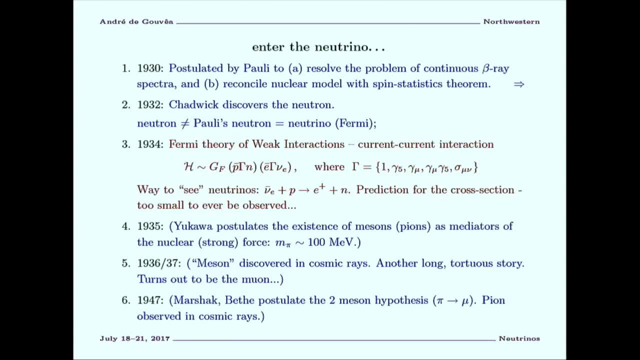 beta decay pretty well. you can fit the model to the. then you can actually calculate stuff. And one thing you could calculate was: so can we ever observe these neutrinos that come out? Because, again, they do have some interaction. So it must be possible in principle to have these neutrinos come in and hit something. 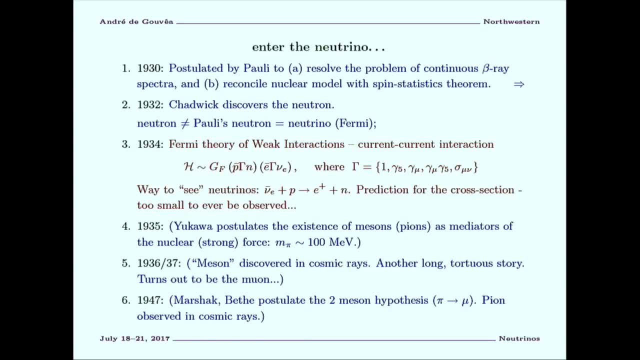 So you could calculate that. You could calculate the cross-section for that. And, for example, using a modern language, you could have the neutrino hit a proton, produce a positron and a neutron. That's possible, Of course. you calculated the cross-section. 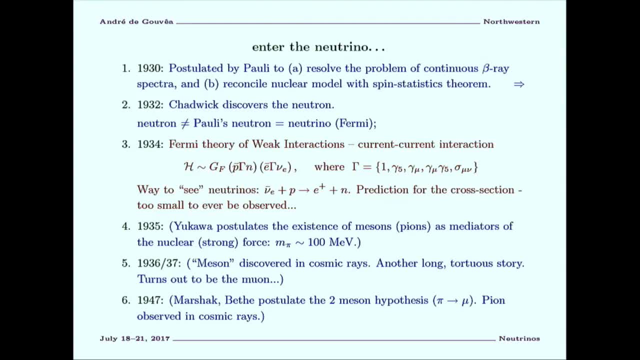 And the cross-section was just ridiculously small. By the way, one thing that Pauli had said was that it was never going to happen that this neutrino would be discovered. He actually had some bets on that, which he lost after about 20 years. 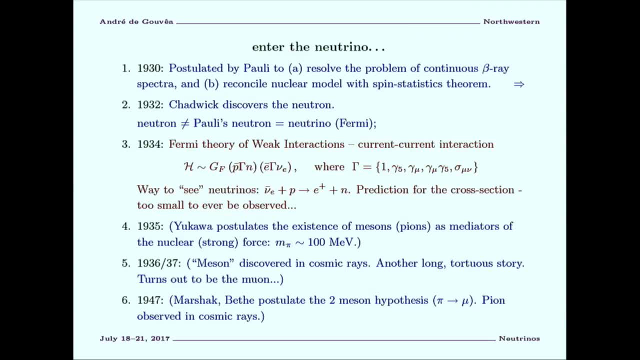 But nonetheless it was possible. He was probably very happy about that, Anyway. so now we had a model that told us how the neutrinos interact And that allowed us to contemplate doing experiments Again. in 1934, when this theory was written down, the safe conclusion was that it was. 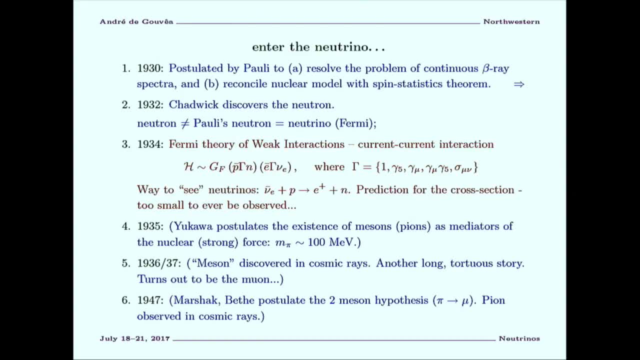 not going to be possible to do an experiment ever to see a neutrino. That was a good assessment at the time. So let me pause here for a second and tell you about other stuff that was going on Again. particle physics is a really exciting field in the 20th century. 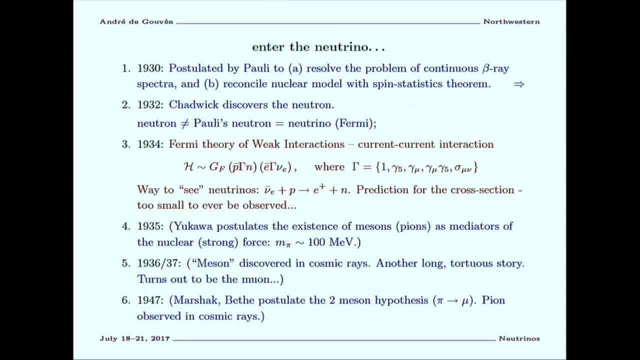 It's a very interesting field. It's a very interesting field Because we knew very little when we were discovering all these funny things. By the way, there's one thing which I won't talk about, which is this interaction. here is the interaction that we write down today as an effective theory for describing neutron. 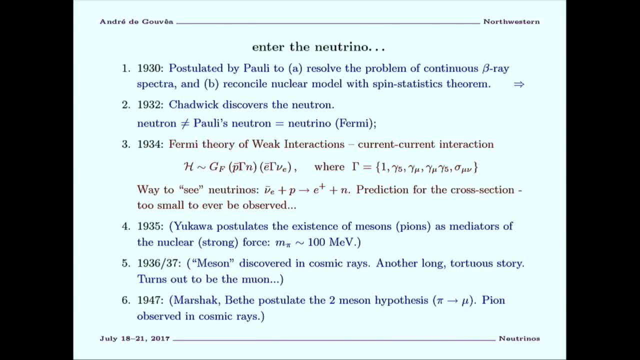 decay. It works pretty well. This current here, certainly written out in this electron neutrino part, that's the V-A current. That's characteristic of the weak interaction that violates parity maximally. We've all heard about this. So this theory is written down in 1934. 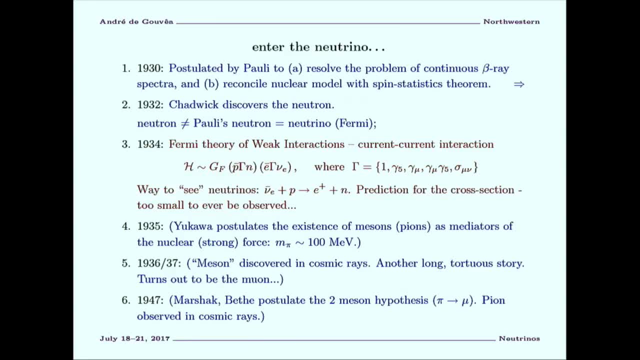 It took until the late 50s for people to figure out experimentally what this current was. There's lots of debates, lots of fights. Every once in a while the data looked like it was. I can't remember scalar and tensor. 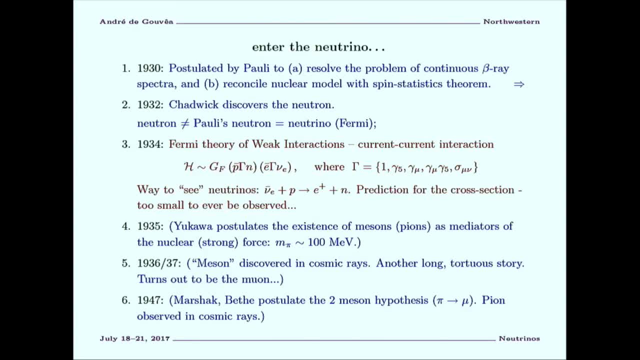 theory. Half the time it looked like a V-A theory or a vector theory or an axial theory. There's a lot of fun history that's going on over here And ultimately this was resolved by better experimental data. But then there are also some very famous people who wrote theory papers addressing the nature. 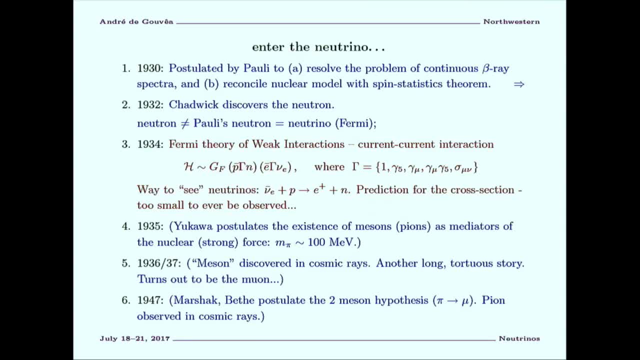 of this current And eventually it was established that it's a V-A current. One of these papers is by Feynman and Gelman. I think that's the only paper that they wrote together And the story is that they actually did separate papers. 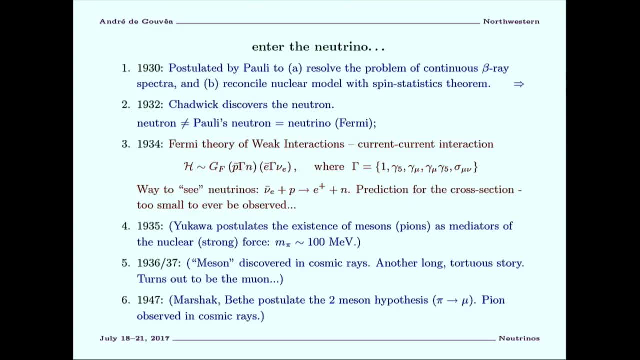 And somebody in their department convinced them or made them actually write just one paper. That story might be false as well, but it sounds like it's a good story. I've heard this more than once, so it must be true. Okay, so what else is going on? 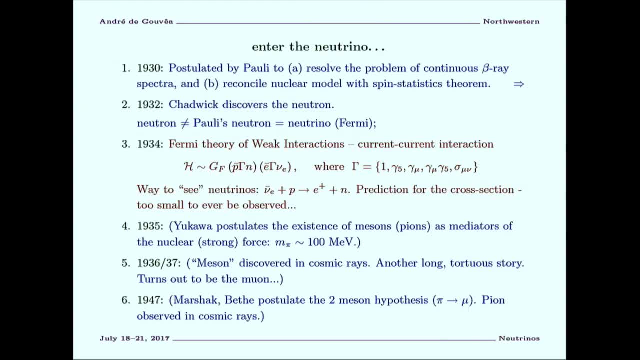 People were trying to understand how neutrons and protons stick together. The most successful model for that at the time was postulated by Yukawa. This is the Yukawa model that postulated the existence of a new particle, which is called a meson. 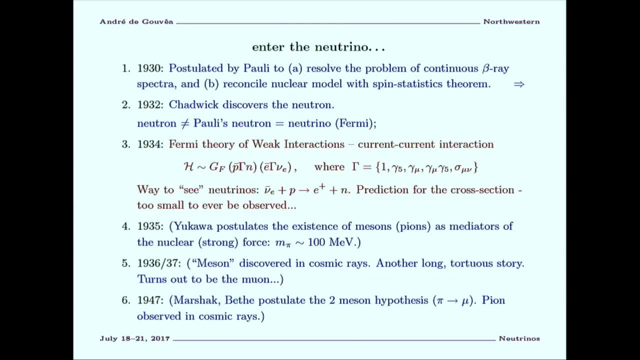 I don't know what name he gave it at the time. I think it was the meson, but that doesn't sound right. Maybe that's it. Maybe that's right. Okay, I think it's the meson And I'll come back and I'll remind you what that name means. 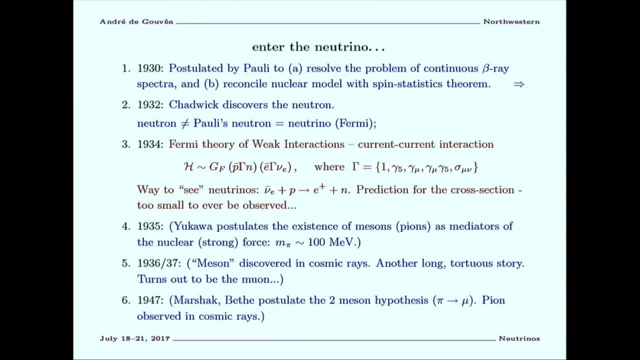 So people know why it's called a meson, right? What's that? Yeah, so the mass is somewhere in between the electron mass and the proton mass, which of course makes no sense for B mesons. but that's a different story. 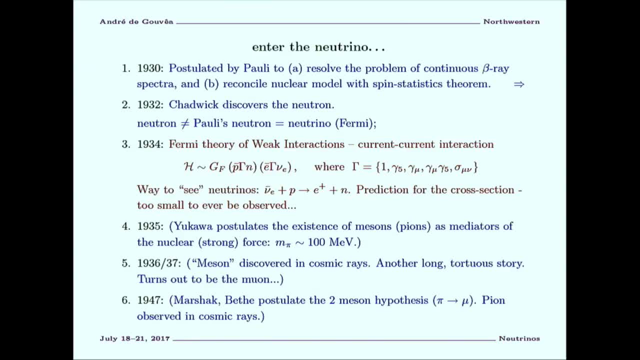 But that's where this name comes from. And what's interesting is he wrote down in 1935. And he mentioned it. He wrote it down And he made a calculation for the mass of that particle, which is about 100 MeV. 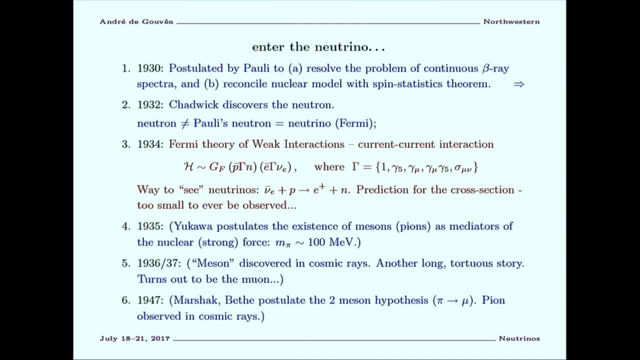 This is in 1935.. One year after that they discovered a new particle doing cosmic ray experiments in 1936. And that particle had a mass of about 100 MeV And people got really excited about that because they had just discovered Yukawa's meson, which 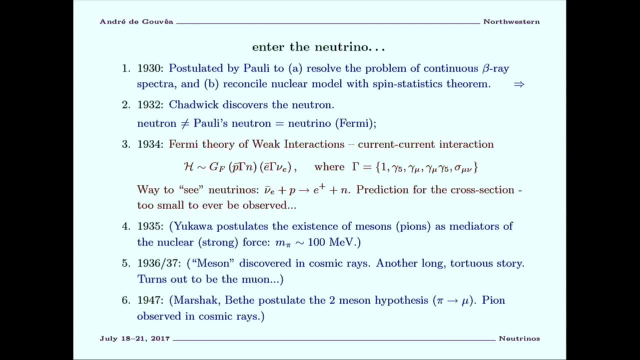 is great, except that it was wrong, And people figured out that it was wrong. And people figured out that it was wrong Because the properties of this particle had absolutely nothing to do with the properties of the meson that Yukawa had postulated. 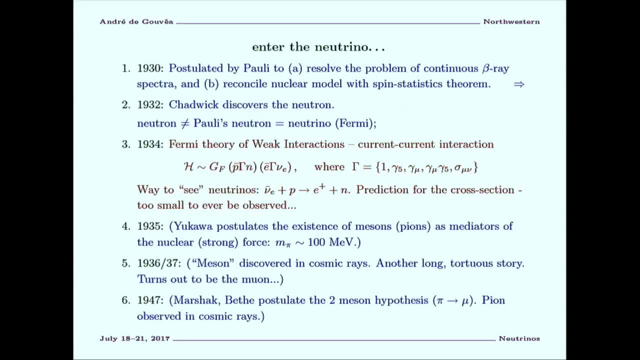 But it was very, very confusing And it took about a decade for somebody to figure out or to postulate that actually what happened was these experiments were happening in a way that the Yukawa particle was being produced. This is happening in cosmic ray experiments. 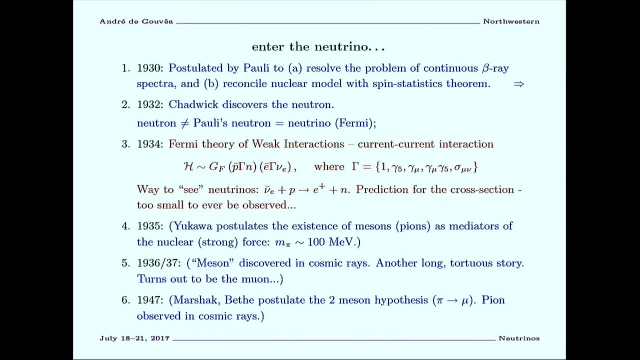 But then that particle was decaying into some other particle, And using modern language, the Yukawa meson is called the pion, and that's the pion that we know about, And the thing that it decays into is a muon. 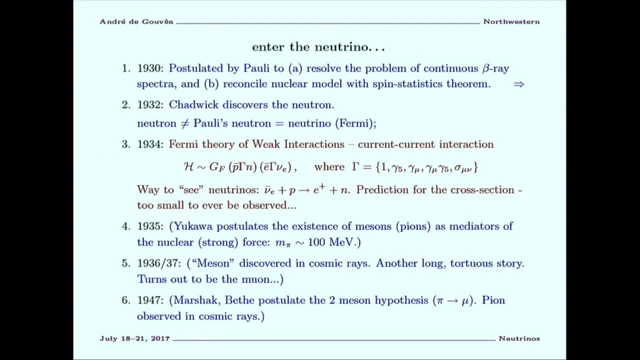 And the muon is the thing that you actually detect in the experiments. This was actually confirmed later on, both in cosmic ray experiments, when people decided to put cosmic ray experiments way up high in the atmosphere, So they did experiments high in mountains and things like that. 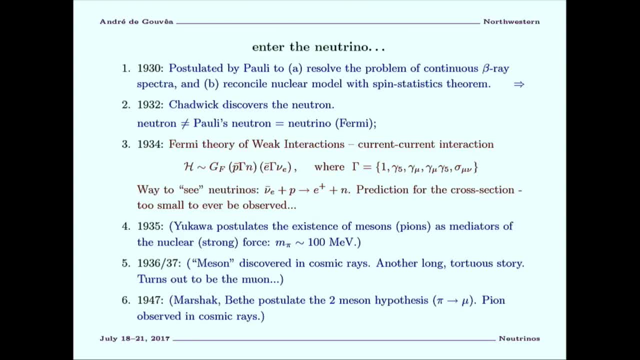 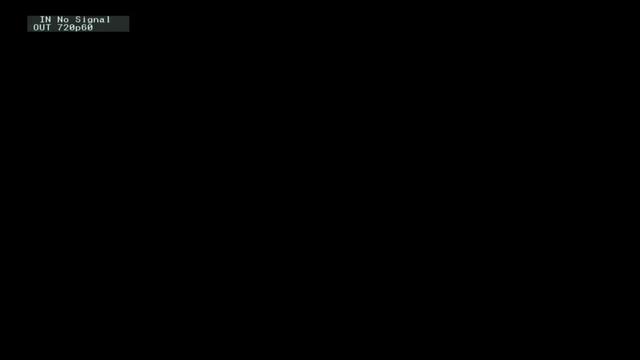 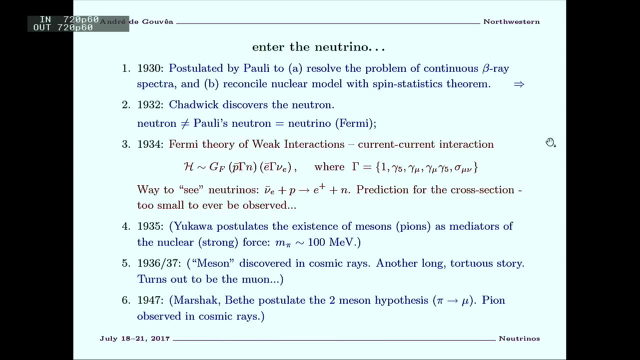 And also when people started inventing particle accelerators And they could produce pions directly in the laboratory And they got very good at detecting them. So there's a lot of history there as well. So this particle that was discovered in the 1930s was the muon. 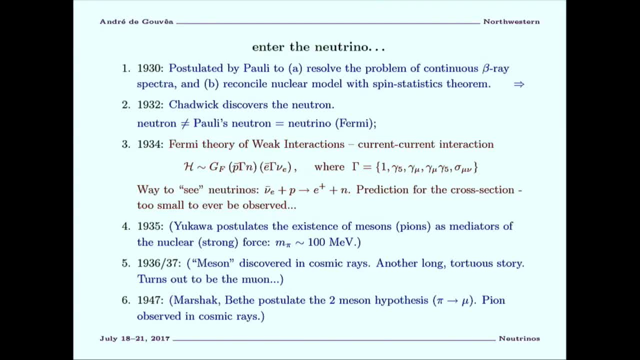 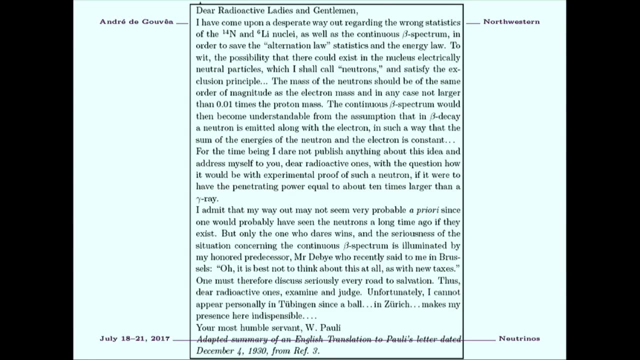 The muon is a very weird particle. The muon is the particle that, after it was established what the muon was, that invited the question: who ordered that? Right, And that was the first to second generation particle that we ever discovered, So we've talked about that. 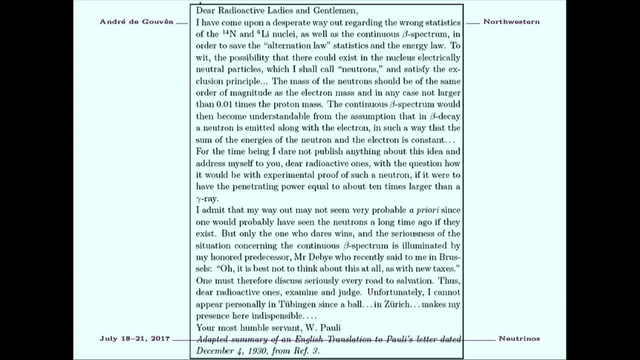 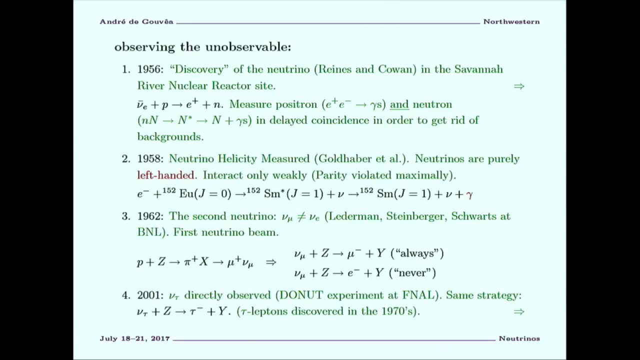 So now that we know where we are, so we've discovered muons And now we want to talk about how did people actually measure the neutrino? So remember, in the 1930s people did a calculation to figure out what the cross section for detecting. 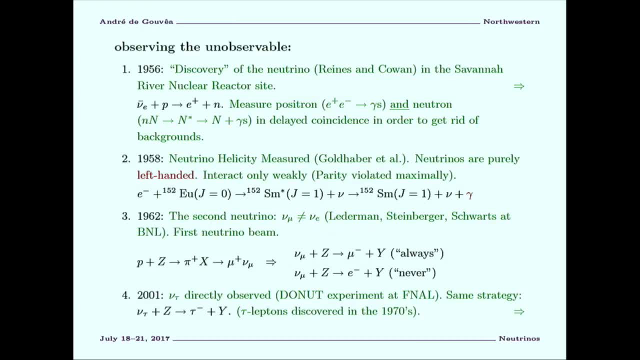 a neutrino was, And they concluded correctly that it was impossible to do an experiment that would actually allow you to observe a neutrino. And between the 1930s and the 1950s, something very important happened, Actually lots of very important things happened. 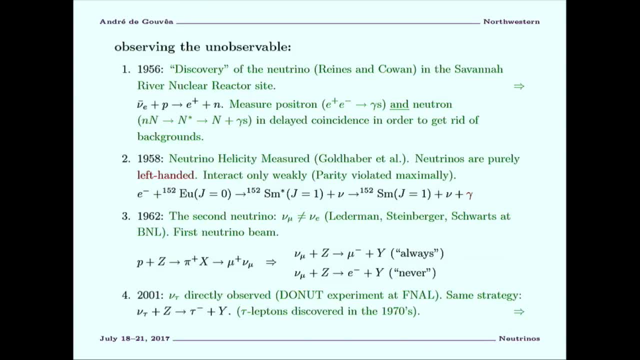 There was a big war And people invented nuclear weapons, And they also invented nuclear reactors For the same reason. by the way, Those three things are highly correlated, And the neutrino was actually discovered in an experiment by Reines and Kao. taking advantage, 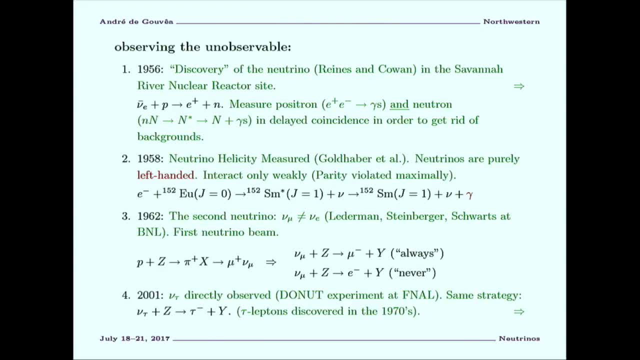 of nuclear reactors. Now, nuclear reactors are very important because they happen to be. you're basically taking a beta decaying nucleus and you're collecting lots and lots and lots of them in one place, So you get a very strong source of neutrinos. 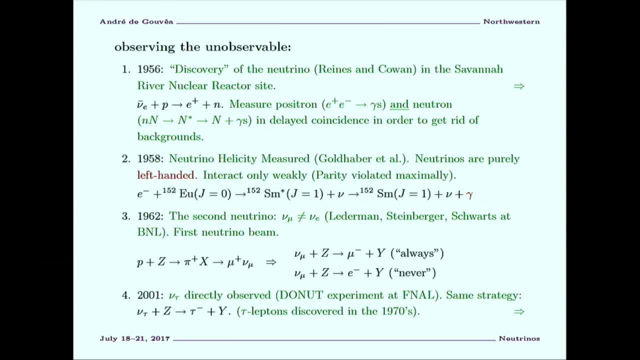 So, even though the cross section didn't change, what changed was the fact that you could now get a lot of these neutrinos to actually do the experiment. One thing which I always like to point out is that this was not Reines and Kao original. 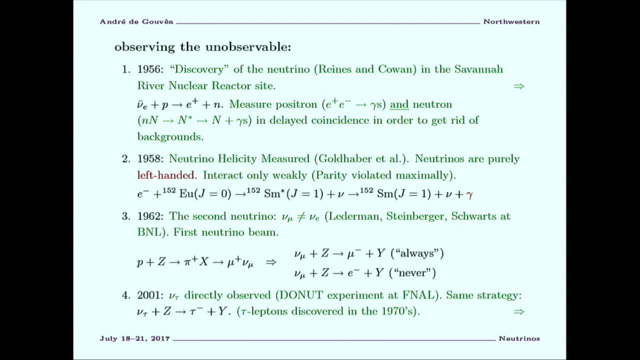 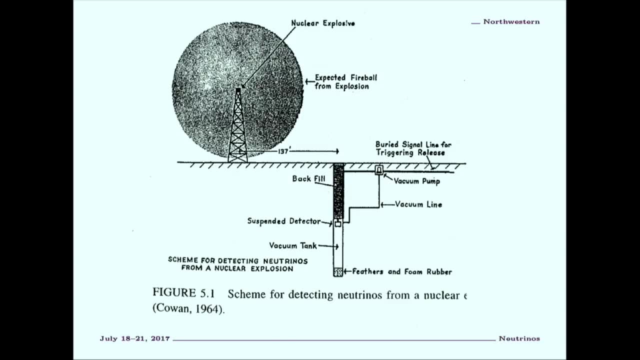 idea. They actually had a different idea. They wanted to detect the neutrinos first, which was not funded. This is a great idea. So this is their neutrino experiment, And there's another physics process that releases a lot of neutrinos at the same time. 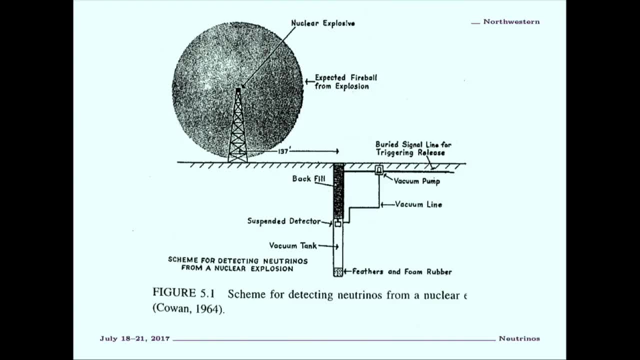 And that's a nuclear explosion. People knew how to do that And they also had lots of those going on in tests of nuclear weapons, So it wasn't totally crazy because this was going to happen. So this is the proposed experiment. Your bomb is exploding over here. 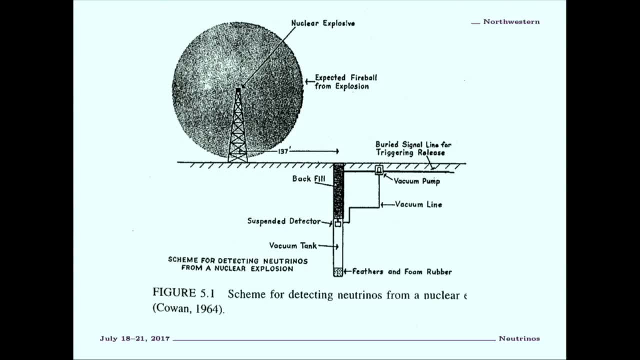 And then you put your detector over here And then you try to detect the neutrinos, And I'll talk about how you do that Now. there's some technical difficulties. The biggest one is that you will have your detector here And you want to turn on your detector while a bomb is going off right next to it. 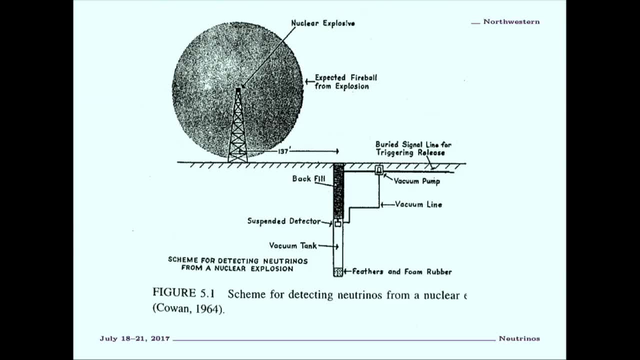 That's a very difficult experiment. Their solution- that's presented here- this is from their proposal- is what they were going to do is, When the bomb gets off, they were going to say: you know where's the gueule at. 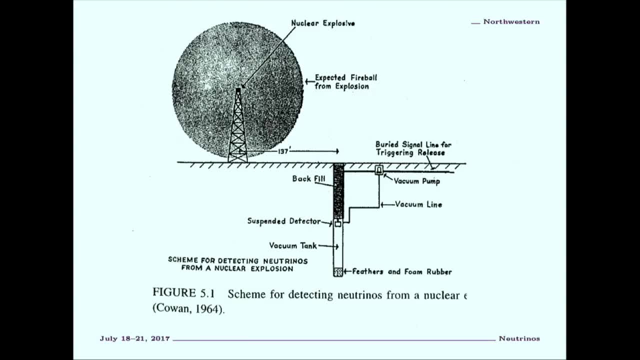 bomb went off, they would let the detector fall, and that's a great idea, because then when the ground is shaking, the detectors, just fine, it's falling, but it's, it's fine. and then they have here feathers and foam rubber which hopefully will hold the detector and everything will be fine, and so this is a great. 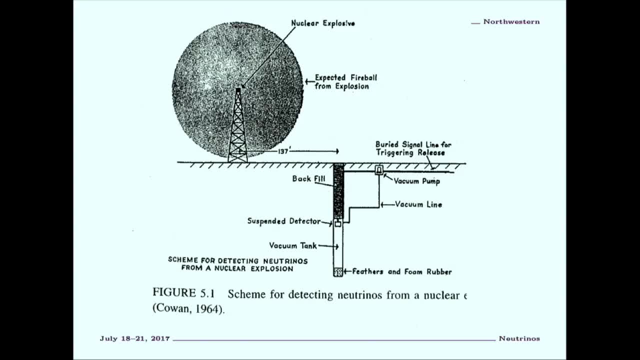 proposal. it was encouraged, but it was not funded in the end. by the way, the flux of nutrients that comes out is quite large. the experiment in principle could have worked. the only other fun thing is that there's a. the distance between the explosion and the tank is a hundred and thirty seven feet, and that's. 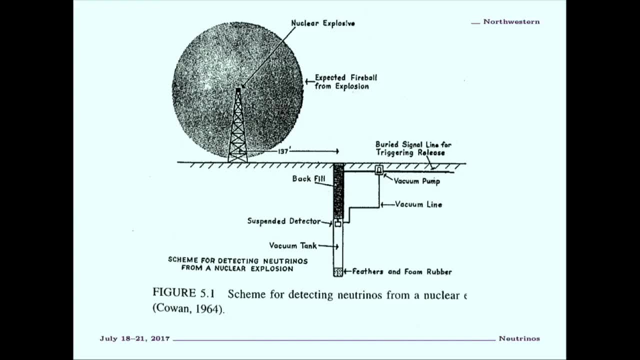 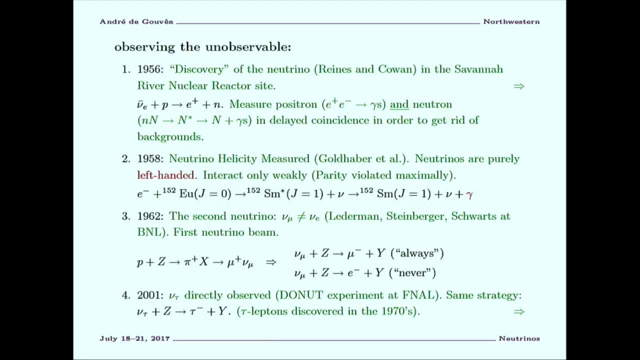 either a joke or it's just an amazing coincidence, but anyway, so that's, that's that proposal. what's that? oh, maybe, I mean, uh, I, I think we still propose a very amazing, amazing experiments, I think I, I would like to argue with that, not that amazing? 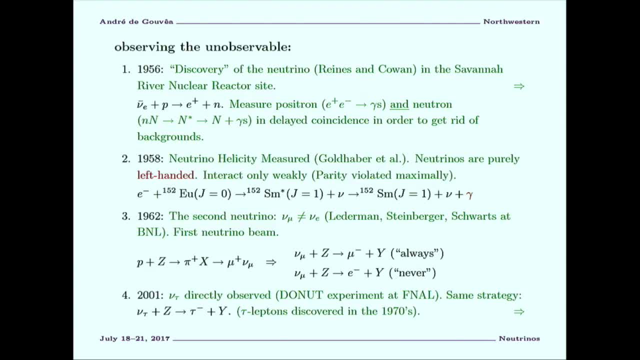 yeah, I don't know if anybody ever measured the neutrino flux from a nuclear explosion- ever something to be a thought about, okay, so this is a really cool experiment and we still do the experiment exactly the same way for neutrinos that come from nuclear reactors. the idea is very simple. you're 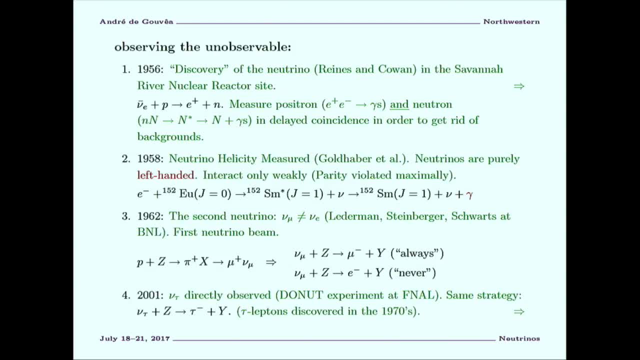 looking for this reaction that you could calculate with Fermi theory. so it's a. it's a neutrino comes in, hits a proton, produces a positron and a neutron, and what people figured out was so if you build a big experiment, this positron that comes out. 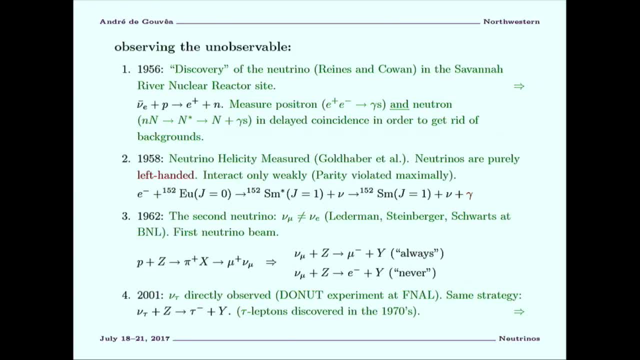 will annihilate with some electron in the material and will give you a gamma ray signature, you know so. you see photons out of that, so that's great. that's one thing that you look for is photons in your detector. the problem is, there are lots of other junk that will do exactly the same thing. 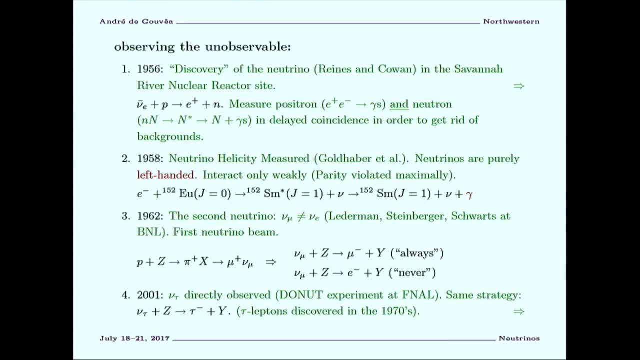 will produce photons in your detector. so what they figured out was: hey, there's also this neutron that comes out. so if I could tag the neutron, because the neutron it random, walks around until it gets captured by a nucleus and then the nucleus DExites. so if you have a large 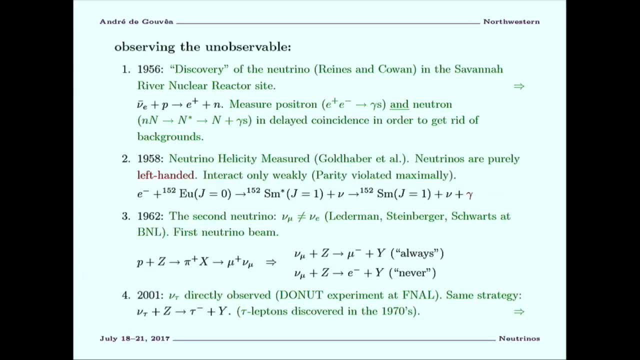 cross-section for nuclear, nuclear nuclei being absorb, I mean neutrons being absorbed. you could see photons coming from this DExitation of whatever absorbed the neutron. and if you do that, then And then you can first see a big burst from the positron and then some calculable amount. 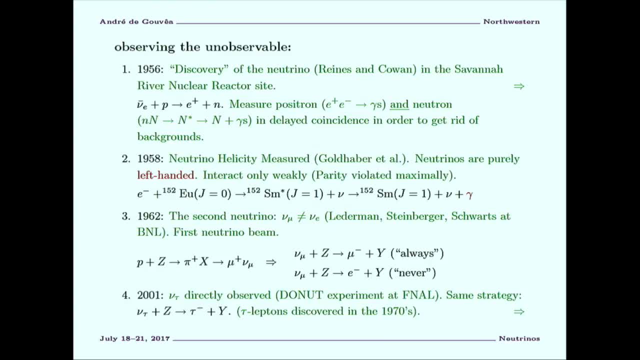 of time. later you see another burst of photons coming from the neutron capture And that was a great way of getting rid of backgrounds and it's still a great way of doing these types of experiments. So these coincidence measurements are very important for doing reactor neutrino experiments. 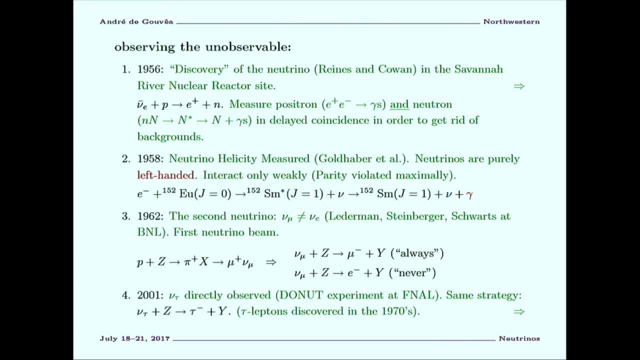 and we still use them today. Okay, so they've discovered the neutrino in 1956, and again, by discover, it means that they managed to see a neutrino hit something. Again, if you're a purist or if you're a theorist, then you can argue that the neutrino was discovered. 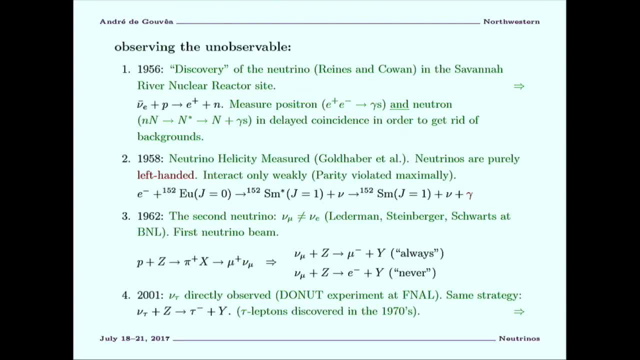 by Pauli in 1930 to explain beta decay. but that's kind of a cheat. We had to see it just to make sure that it was the real particle. Then a lot of progress happens after that. In 1958, we figured out that neutrinos are close. 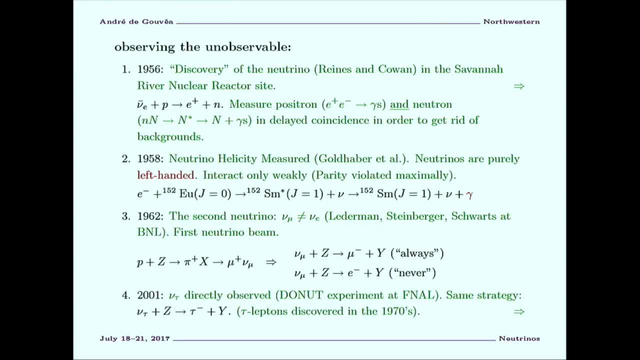 They're completely left-handed. The helicity of the neutrino was measured, So neutrinos are left-handed, antineutrinos are right-handed. This is a really nice experiment done by Goldhaber et al, where they figured out that, even though 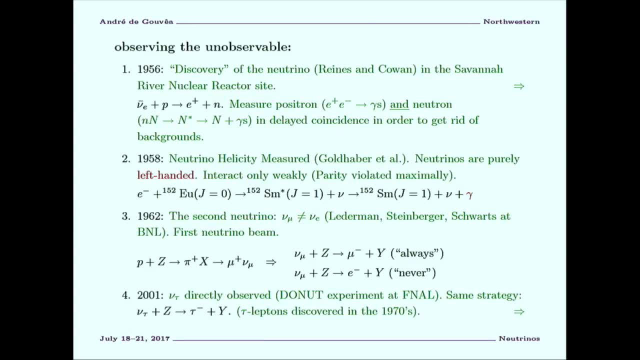 you can't see the neutrino, you can still infer from angular momentum conservation of a complicated nuclear physics process what the helicity of the neutrino is. And of course it's a maximally parity-violating interaction. Okay, so we're here in 1958.. 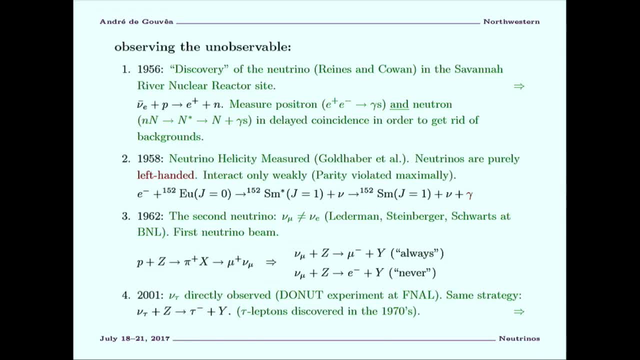 And I don't have a lot of this story written down, so I'll tell you about it in words. Remember, we discovered this thing called the muon, And the muon is an interesting particle. We figured out that it decays into an electron and two neutrinos. 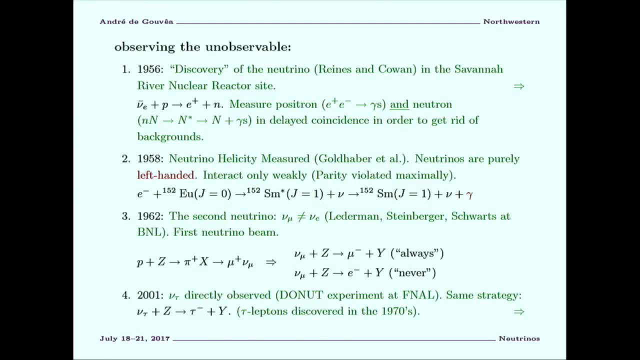 That's by far the dominant decay mode of the muon. Otherwise, the properties of the muons are very electron-like. That's why it's called a second-generation particle. It's a partner of the electron. Then people started asking questions about the muon. 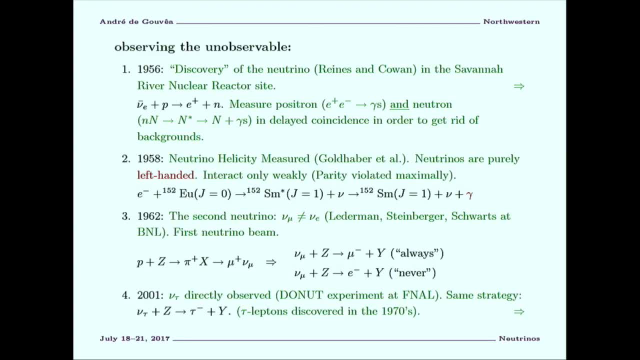 And one really good question you can ask- and they asked that question at lots of different levels. If the muon looks like an electron, it's very similar to what happens with radioactive nuclei, in the sense that we can take a nucleus and we can convert it into- in quotes- a heavier 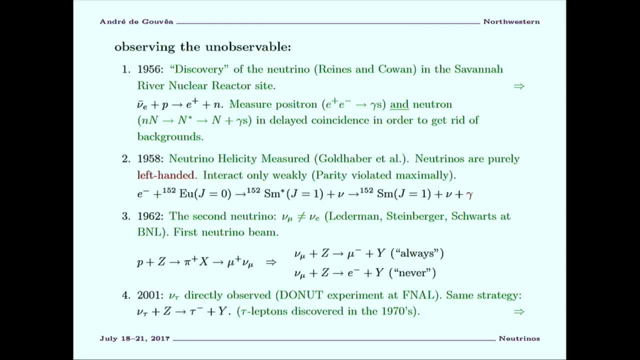 version of the same nucleus by exciting it, and then those nuclei tend to de-excite by emitting gamma radiation. So people are starting asking the question: maybe the muon is an excited state of the electron. It's a very great, very good hypothesis. 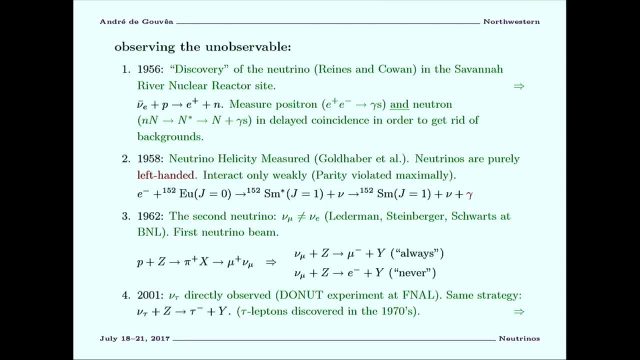 So that means we should be able to observe this excited electron de-exciting into an electron and a photon. So people asked: does this thing happen? And they started doing experiments And it turns out it doesn't happen at all. It's not. 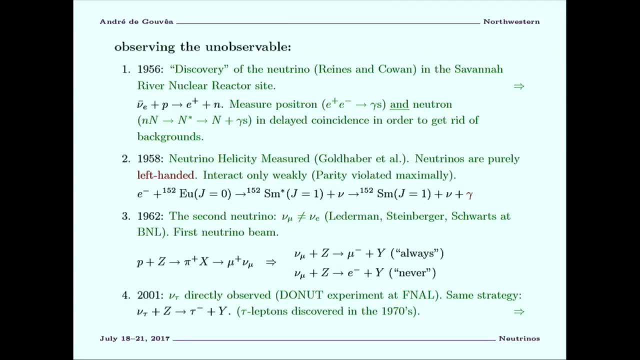 It's not. It's not at the, you know, 10 and minus 1 level. if you talk about branching ratio Doesn't happen at the 10 and minus 2 level. So at some point people said, yeah, this excited electron thing is just wrong. 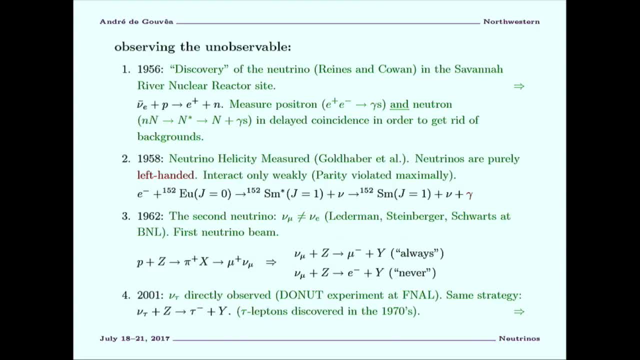 However, they went back to asking this question again because they had another idea, which was: so we know how this muon decays, right, The muon decays. So let me write it down over here. So the muon decays into an electron. 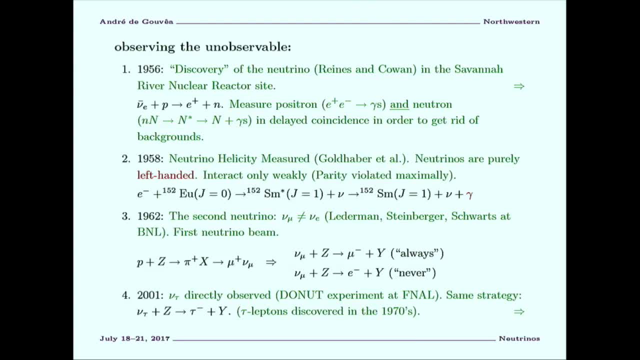 It's a neutrino and an antineutrino, So that's the dominant decay mode of the muon And we know that works really well. It's also described by the Fermi theory, which is a sign that the weak interactions were. 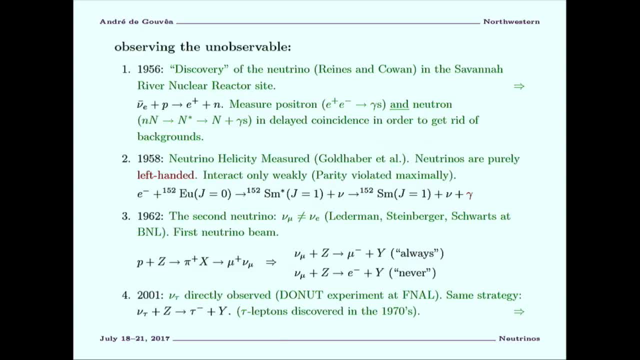 the same that describe muon decay and pion decay and nuclear beta decay. But if this is how the muon decays, people knew enough about perturbation theory back then in the 1940s that you could ask yourself: why don't I close this neutrino loop? 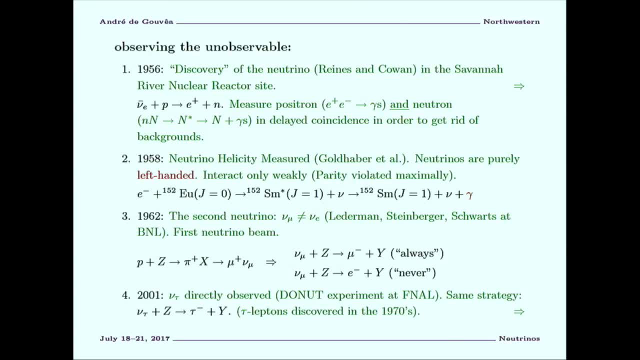 And what happens is you remove a neutrino loop. You have a neutron Spider-T foot. You put it inside a neutrino loop like this and add a photon somewhere, So the muon has to decay into E gamma. It's a simple calculation. 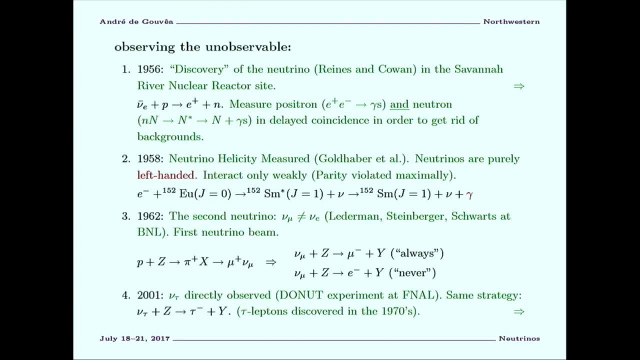 It wasn't simple back then. People made some estimates and the estimate was that the branching ratio was something like 10 and minus 4 or 10 and minus 5.. The error bars were big. So, again, people kept doing experiments. 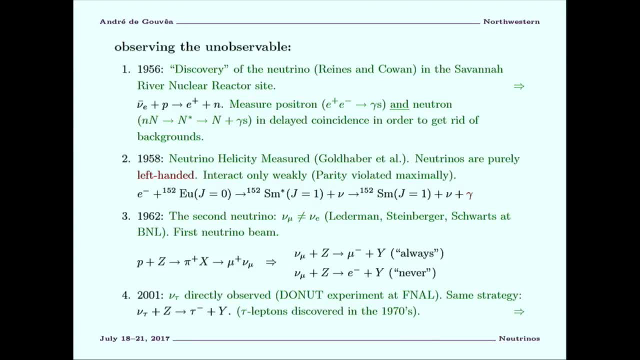 And they got the 10 and minus 4.. 10 and minus 5.. 5, 10 to the minus 6, and the branching ratio was smaller than that. So this is a big puzzle, because the muon definitely can decay into electron, neutrino and anti-neutrino. 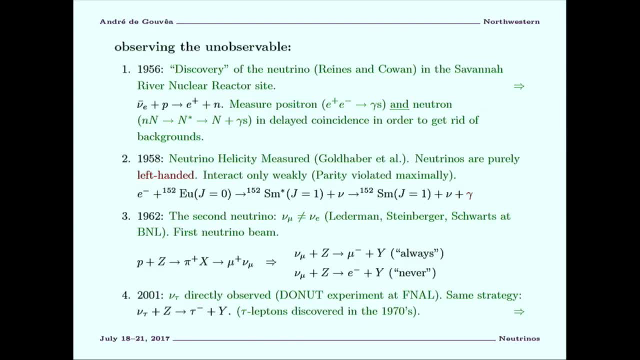 But somehow something is preventing it from decaying into E gamma. This was a big puzzle, and this was actually resolved in a way that's very important. So in the language of the day, the solution to this was called the second neutrino hypothesis. 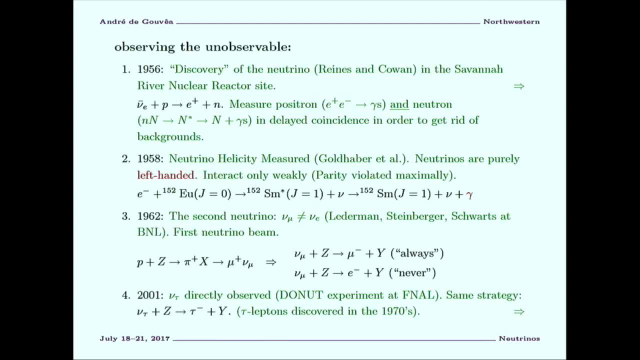 The idea was that when the muon decays into an electron, a neutrino and an anti-neutrino, then the neutrino and anti-neutrino that come out are not a particle-antiparticle pair. They're two different particles. 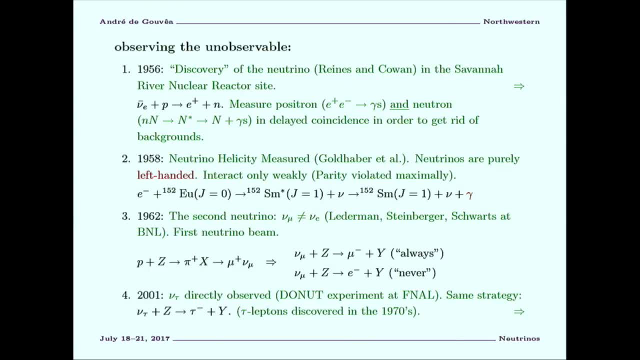 So this is a second neutrino hypothesis, And along with that we could explain using more modern language that the muon doesn't decay to E gamma because it violates a conservation law. So we invent a new quantum number. There's an electron nest and a muon nest. 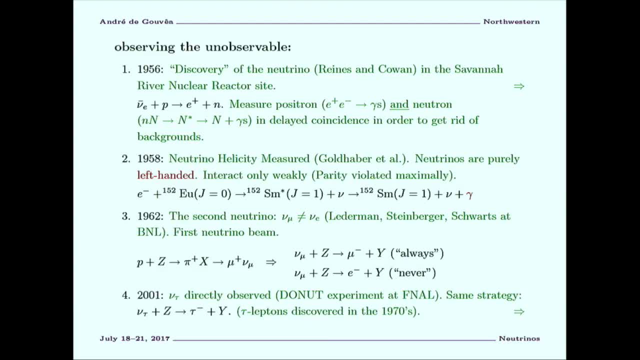 And the electron nest and muon nest are conserved. We call that electron number and muon number, And that explains why mu to E gamma doesn't happen. This is important because this conservation law is actually wrong. We've established that experimentally by now. 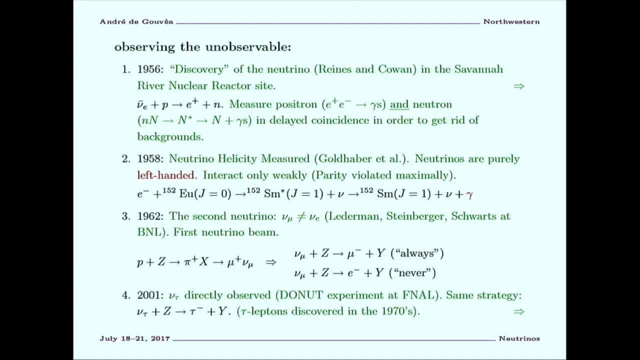 But nonetheless this two neutrino hypothesis came up And the question is: how do you resolve that? experimentally, And people came up with a way And the way of doing that. this is in the 1960s. This is an experiment that discovered the muon neutrino. 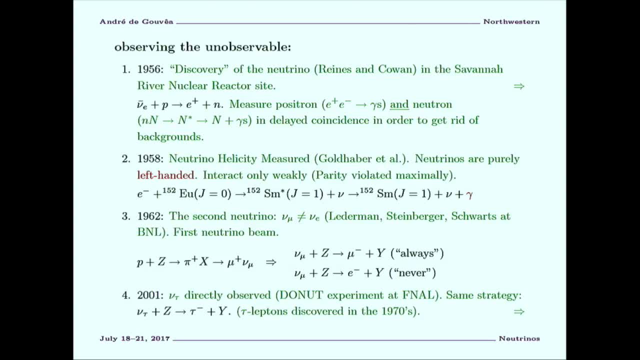 if you want to think about it that way, It's a very important experiment. It's actually peculiar that the discovery of the second neutrino got the Nobel Prize before the discovery of the first neutrino, But that's how Nobel Prizes work. 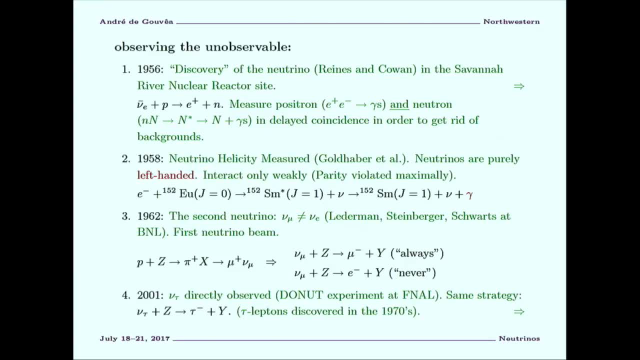 So again there's this very famous experiment, And the biggest contribution of this experiment is that these people- this was led by Letterman, Steinberger and Schwartz- And they actually produced the first neutrino beam. And they actually produced the first neutrino beam. 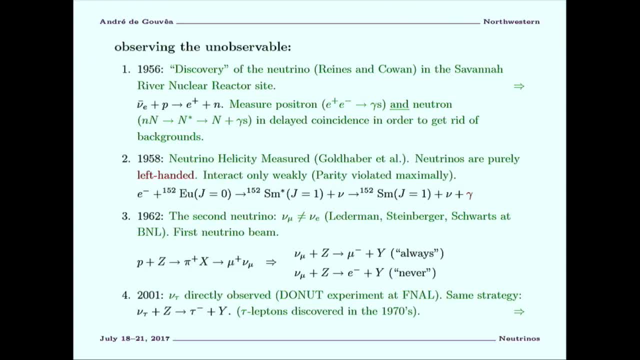 The idea is really simple. So you take protons, You shoot it on a target, A bunch of pions come out. If you wait long enough, the pions decay. Pions decay into muons and neutrinos. If you wait some more and you put a bunch of junk. 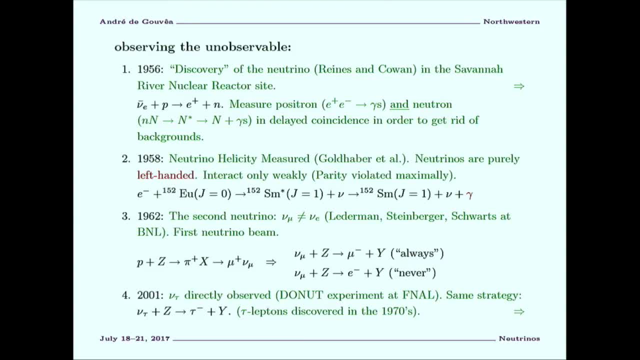 in front of the beam, all of the muons get absorbed And what you're left with are only the neutrinos. It's a really crappy beam. It's very, very big. It's a big beam like this, And you can't not have a very big beam. 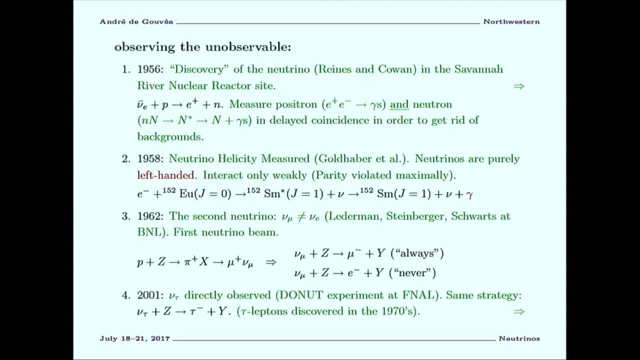 because you're basically taking a bunch of pions that go everywhere And you're just very, very quickly trying to aim them all going in the same direction And then you wait And, of course, when the pions decay, the muon and the neutrino. 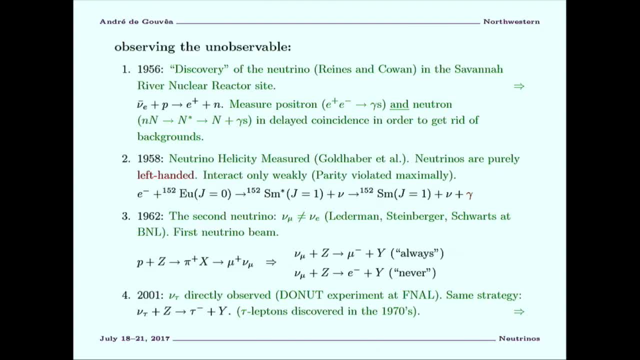 go all over the place, But it's a beam nonetheless. This is still how we make neutrino beams today. We haven't gotten any smarter. And the idea is very simple: If you take these neutrinos, you're going to get these neutrinos. 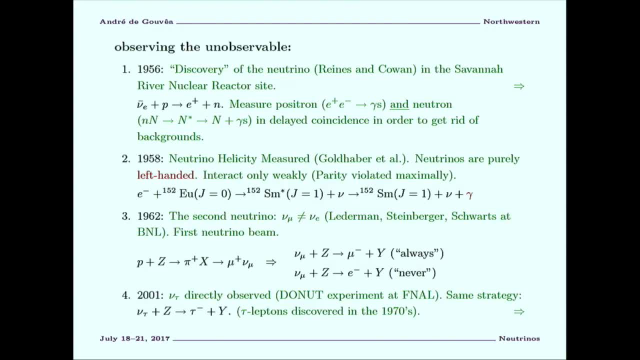 And if you believe in this muon number conservation law, these have to be muon neutrinos. So that means if you take these neutrinos and you make them hit something, they should only be able to produce muons And they should not know how to produce electrons. 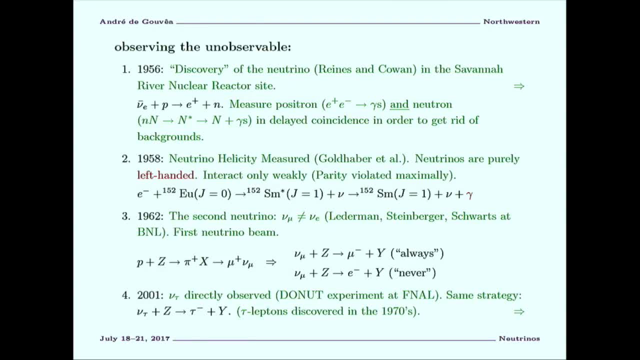 Because if this particle is a muon neutrino, this reaction goes. But this reaction is forbidden because it violates both electron number and muon number. So that's the experiment And that's what they confirmed. And just to keep in mind, if this neutrino 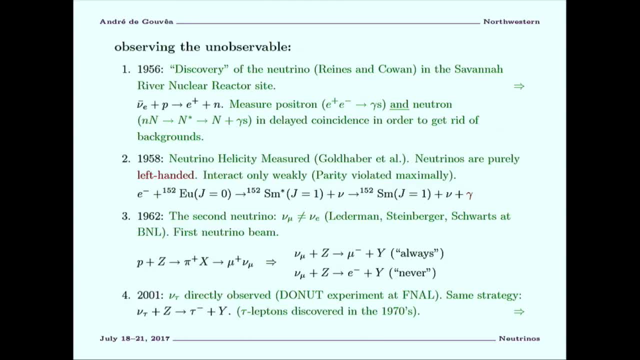 could do both things. it would probably make more electrons, because the electron is lighter, So there's more phase space for that. So they do the experiment And sure enough, this never happens, And this thing here always happens. What's also interesting about this? 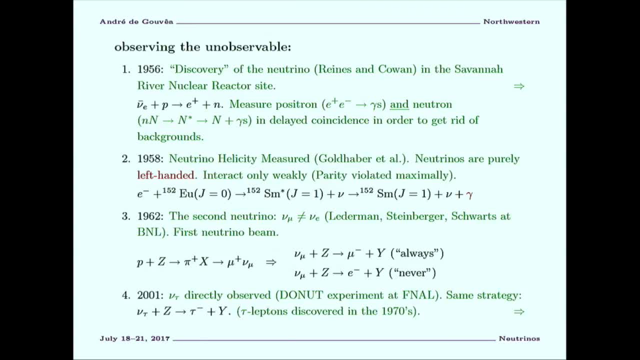 is that the neutrino experiments we do today are actually aimed at measuring exactly this thing. that never happens, But we know how to do it. But we know how to make it happen if we're very patient. So this is the experiment that established that there's 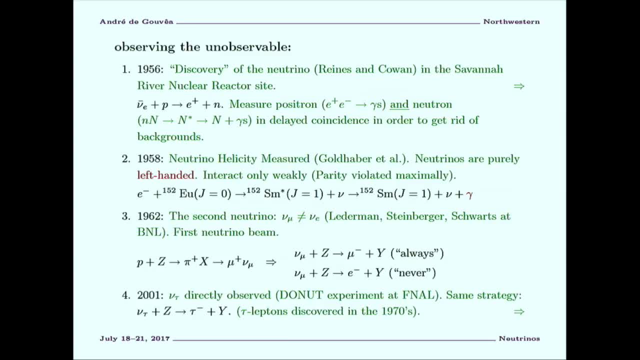 actually a second neutrino. Then, of course, in the 1970s, people found out that there's another particle called the tau, which is also like an electron and a muon, but it's even heavier. So it stands to reason that there's a third neutrino. 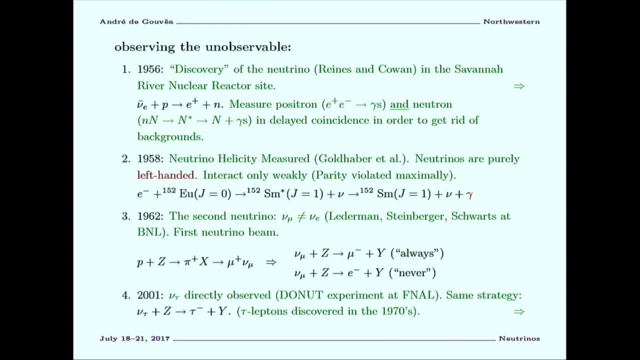 The presence of the third neutrino was established in lots of different ways, including at LEP from Z decays, But it took us a really long time to actually see the tau neutrino do something. So again, just like we wanted to see the muon neutrino do, 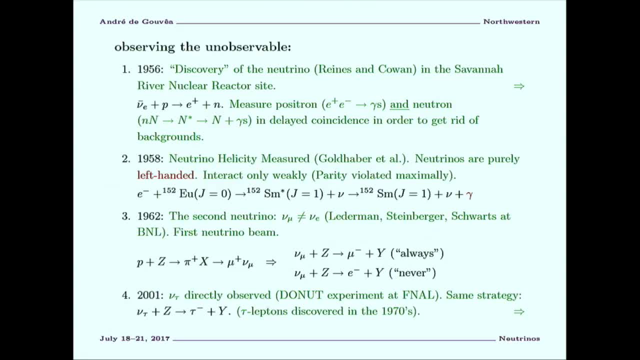 something, and we wanted to see the electron neutrino do something. we wanted to see the tau neutrino hit something and produce a tau. This experiment was successful only in the 21st century. So there's this thing called the DONUT experiment, which 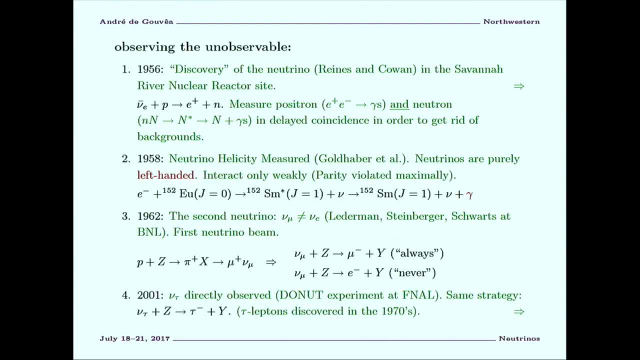 took place at Fermilab. This is a great experiment name. It stands for Direct Observation of New Tau, And this is done in 2001.. One thing which is fun to keep in mind: this is way after the top quark was discovered. 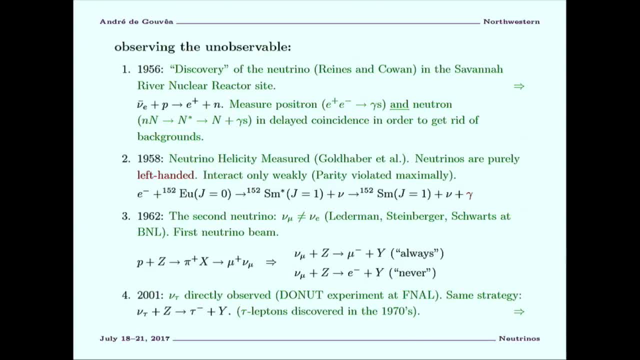 So again, if you're a skeptic, the tau neutrino was the last matter particle to be discovered in the Standard Model. by a lot I mean the tau. the top is in the mid 1990s. Let me show you how the tau neutrino is discovered. 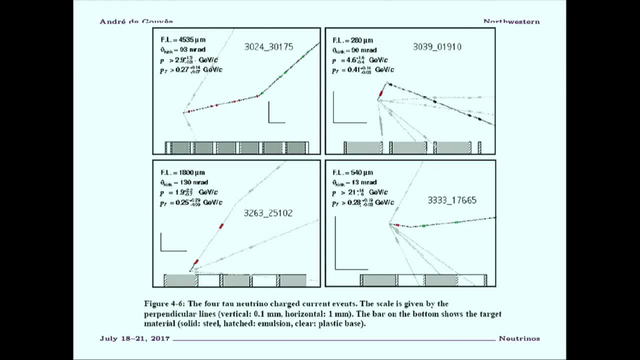 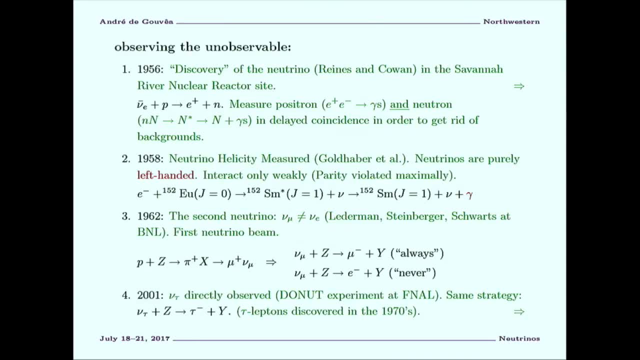 because it's kind of cool. So this is how you see the tau neutrino. What happens is you try to make a tau neutrino beam. You do it in exactly the same way that you produce this muon neutrino beam, except that the pion doesn't decay into tau neutrinos. 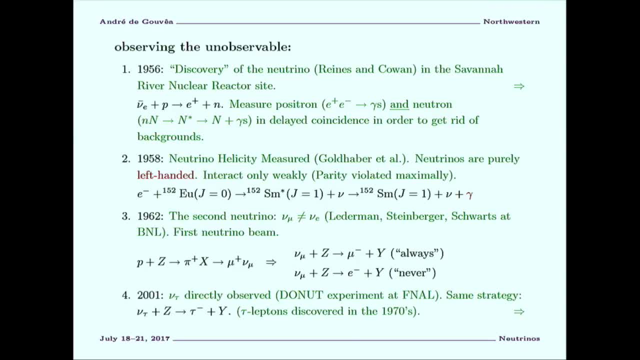 So you need a heavier meson for that. So you need a higher energy beam that produces a lot of d sub s's. These are C bar s bound states, which like to decay into taus and tau neutrinos. So if you have a high enough proton hitting a target, 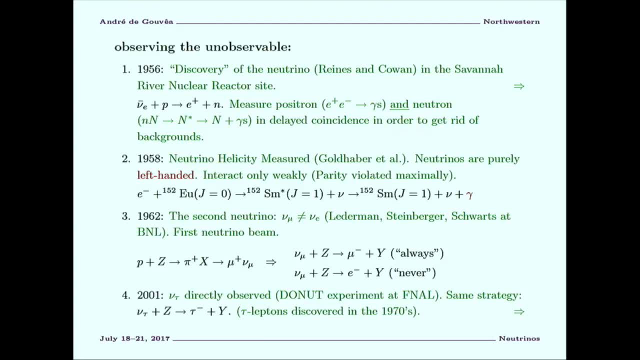 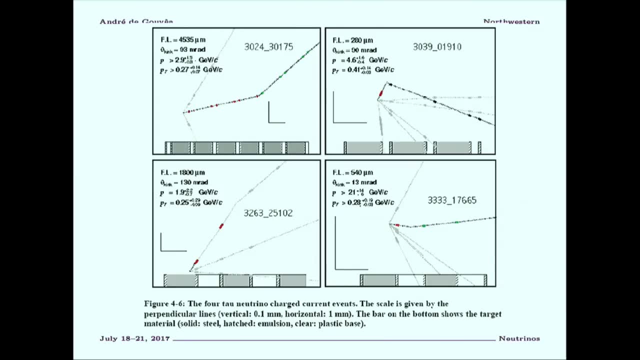 you produce these charmed and bottom mesons and these guys can decay into taus and then you get your tau neutrino beam. So the idea is, this neutrino's coming from over here. you don't see it, it hits something. 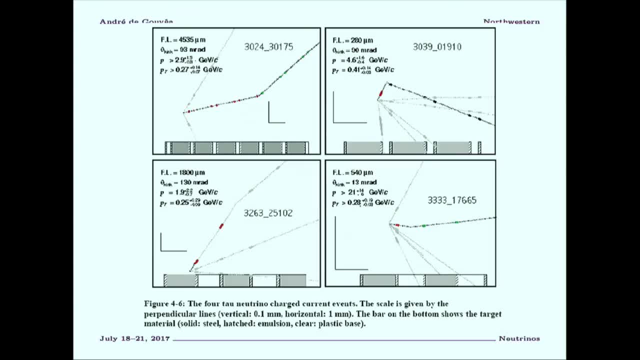 it produces a particle that travels a little bit and then it has a kink in it, and that's indicative of a tau decay. So the idea is that a tau was produced over here and then it decayed into a muon and two neutrinos. 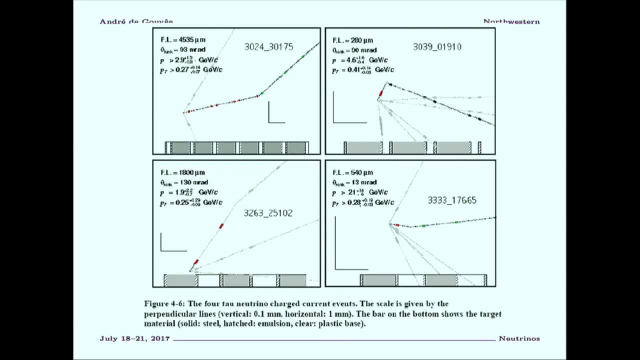 which is why you get this kinematical kink. This is a challenging experiment because this happens relatively quickly. I think the scale here is of order, a fraction of a millimeter. that's what's written down over here, And on top of that this has to be a neutrino detector. The cross sections are still very small, so that means you need a lot of mass. So you need a really dense detector with a lot of mass in it, Which makes measurements really hard. because if your detector's really dense and massive, that's great, because lots of neutrinos will hit it. 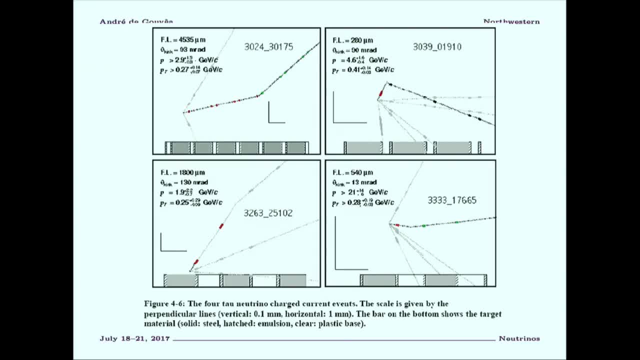 that's bad, because everything that gets produced will be absorbed by your detector. So that's why people were clever enough to have a technology where you actually could see the tau track that was produced inside of this thing, which I think was lead. Okay, so you have this lead emotion detector. 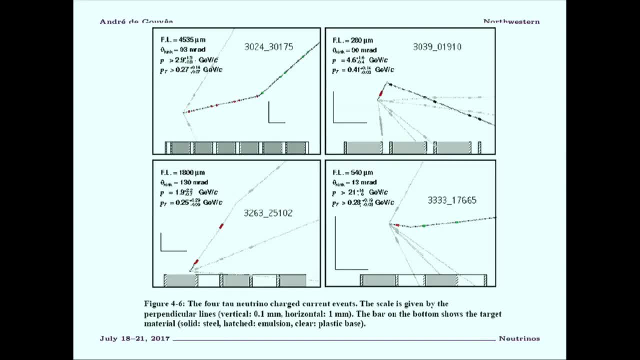 The lead gives you the target, the emotion gives you the ability to see these tracks And it's a very big detector. and this is a picture of almost all of the tau neutrinos we've ever seen. ever, really ever. The number of tau neutrinos we've ever seen is less than 10.. That's less than the sample of Higgs bosons that we've accumulated from the collider experiments. We don't know a lot about the tau neutrino if you don't believe in the standard model of weak interactions. We have not measured its properties at all. 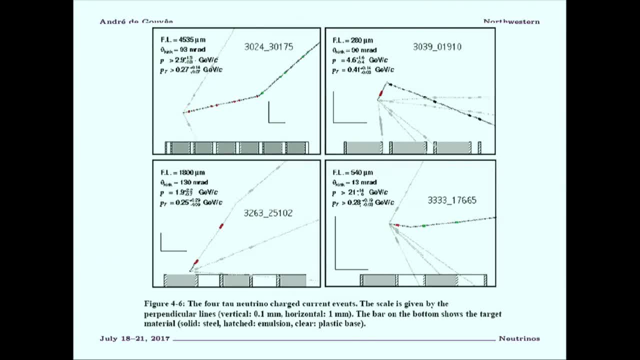 The final thing I'd like to mention about this experiment is that this experiment is crazy hard Because, remember, we're producing the tau neutrino beam, which is really hard to do. and it's really inefficient Because every time you produce a d sub s meson, you produce a gazillion pions which are happy. 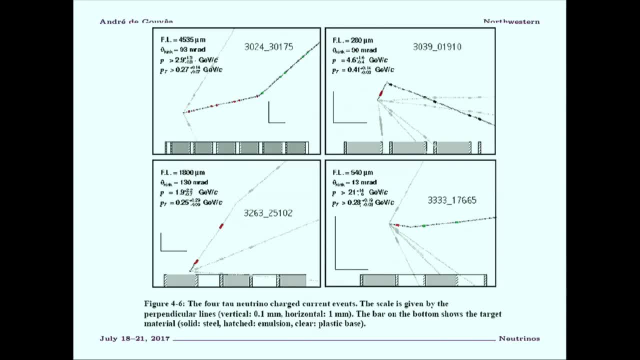 to decay into muon neutrinos and kaons, which also decay into muons and electron neutrinos. So when they do the experiment and they show us these really, really nice results, they actually see. and, by the way, to make it worse, this is not a real time experiment. 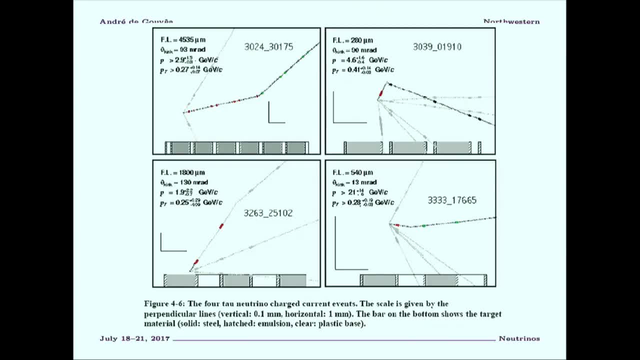 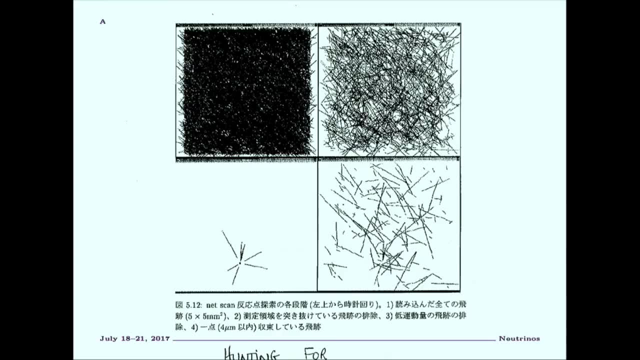 This is an old fashioned experiment where the tracks are left in place and you have to go look for them later. So their sample, already a little bit cleaned up, looks like this. These are all the tracks that they have, And out of this mess you have to figure out that there's a tau decay in here. 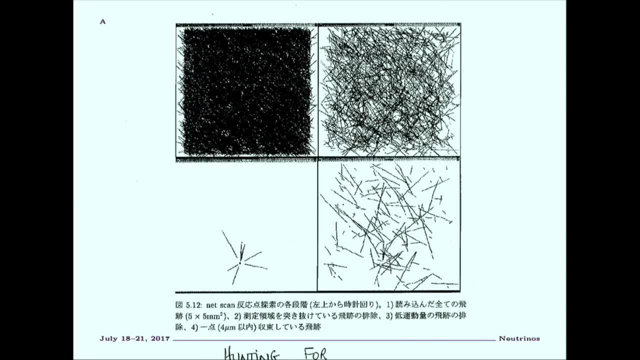 And they tell us that they know how to do it And we believe them And that's why we know the tau neutrino was discovered. All tau neutrino observations, by the way, that were done and were identified as tau neutrinos come from these types of experiments. 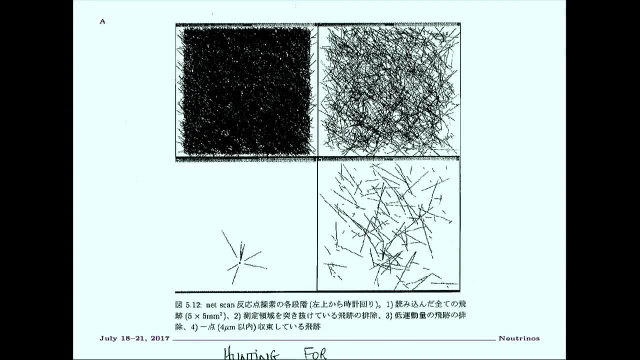 The other evidence that we have for tau neutrinos is indirect, by looking at neutral current events in large atmospheric neutrino detectors and inferring from the absence of muon neutrinos that the tau neutrinos are the thing that are doing something. OK. 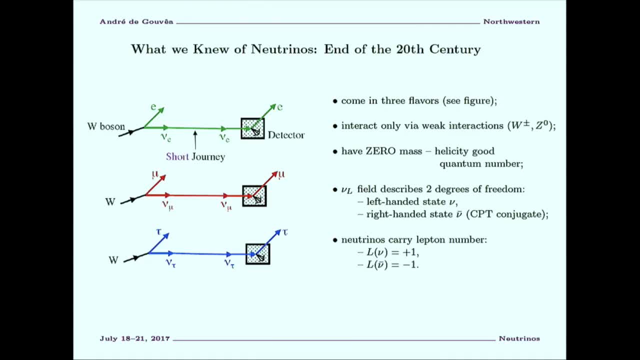 So good. I think I made good progress. So let me summarize the story so far. So if you pick a standard model textbook from the 1980s or the 1990s, it will have a really tiny chapter on neutrinos. 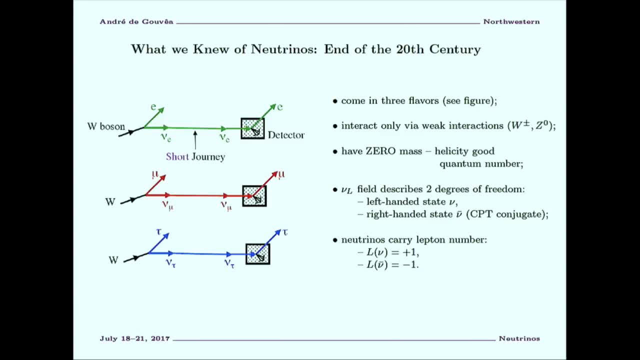 And that's what that chapter will say. if it's a long one, This is what we know about neutrinos. There are three flavors of neutrinos: an electron neutrino, a muon neutrino and a tau neutrino, And they're defined according to what's the charge. lepton that talks to it via charge-current-week. 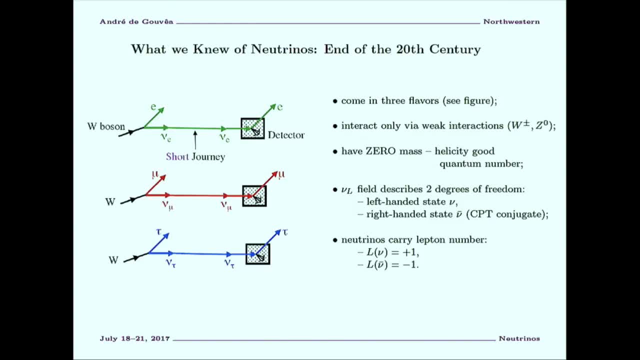 interaction. So the new E always comes in with an electron and every time it hits something, it only knows how to produce electrons. There's a new mu and then there's a new tau. They only have weak interaction, so they only talk to the W and the Z. 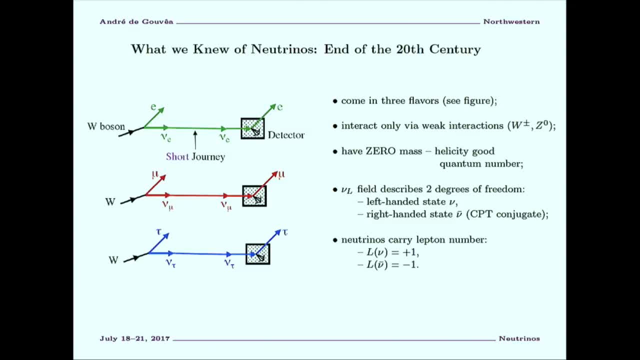 We have no evidence that that statement is incorrect As far as we could measure. until very recently, the neutrinos were supposed to have no mass, And this is very. if this had been true, it would still be quite interesting. So the neutrino was the only massless fermion that we knew about. 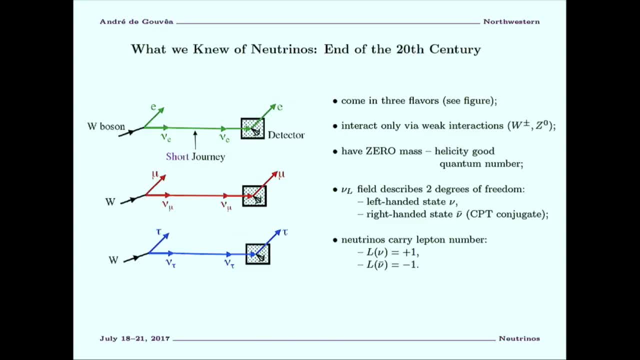 And of course we were wrong, so we don't know about that either. But massless fermions are very interesting And you all know about biofermions. So a massless neutrino is the poster child of biofermions, especially because it's only 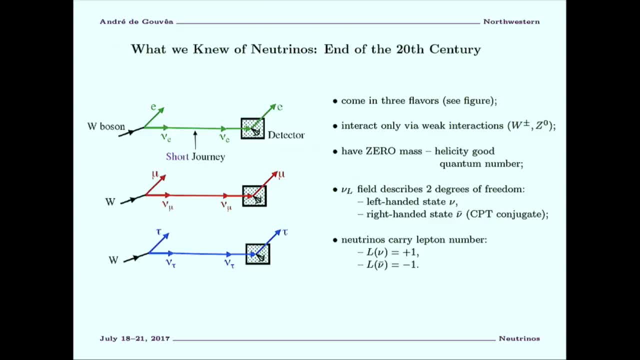 produced by weak interactions, And the weak interactions are maximally parity-violating, which means that every time you do an experiment with neutrinos, the neutrinos are always left-handed. So that's interesting. Every time we do an experiment with anti-neutrinos, the anti-neutrinos are always right-handed. 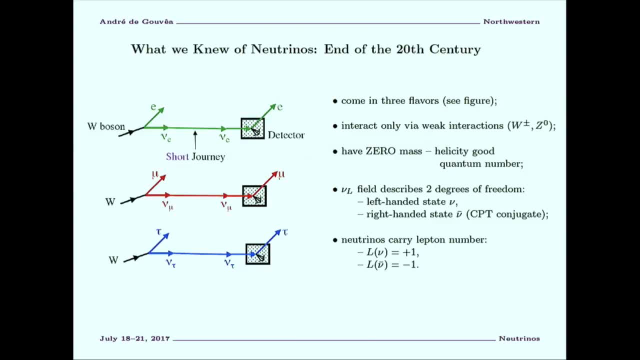 We have never seen that not be true, And that's interesting. So that means we can classify the neutrinos by their handedness. That's what's written over here. And then there's this thing which I just said: The neutrinos are a great biofield. 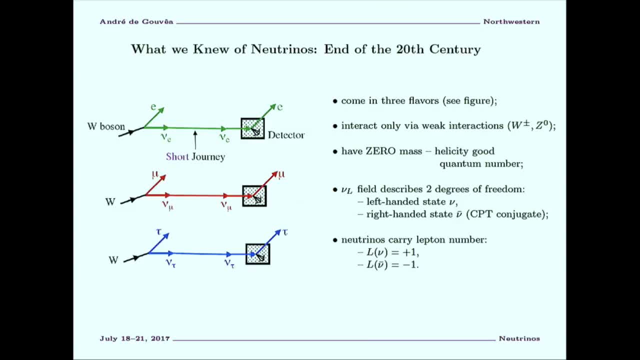 As far as we know, we only need two degrees of freedom to describe a massless neutrino: the left-handed guy and the right-handed guy. And that's exactly right. And that's exactly what a biofermion contains. And this is important because we have to check if that statement is actually true or not. 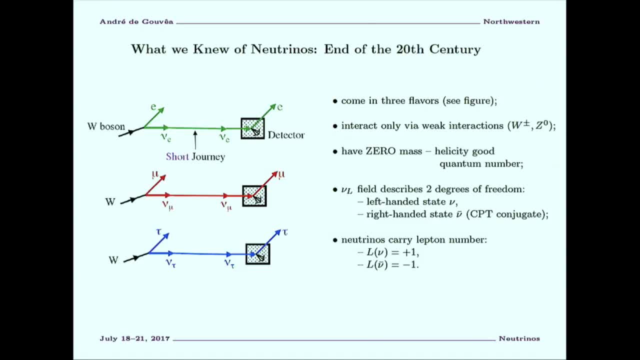 Finally, there's, on top of this flavor conservation law. there's another conservation law called overall lepton number conservation, which is, if you do an experiment and you count how many leptons go in, the number of leptons that go out is the same. 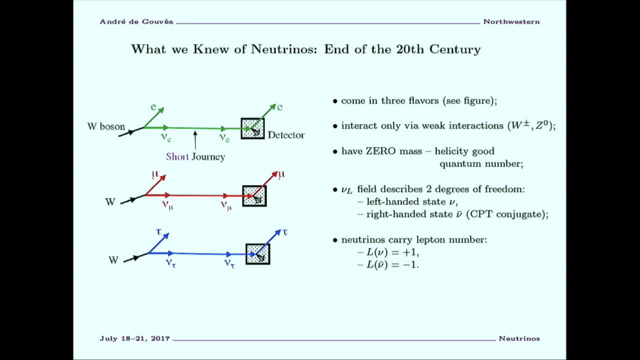 And it's in this sense that we can define a neutrino versus an anti-neutrino. And again, as far as we know, we can't define a neutrino versus an anti-neutrino. And again, as far as we know, we can't define a neutrino versus an anti-neutrino. 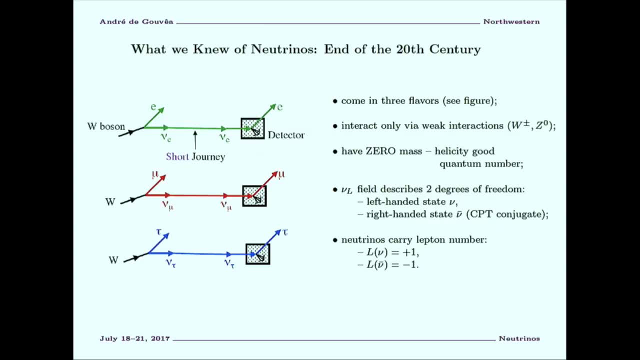 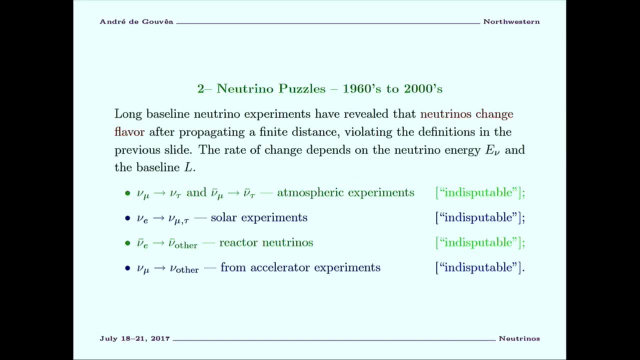 This is an absolute, true statement about nature. OK, So now the next step is for me to tell you why a lot of the information here is wrong, And this has to do with stuff that started happening in the 1960s, And I'll start telling you this story. 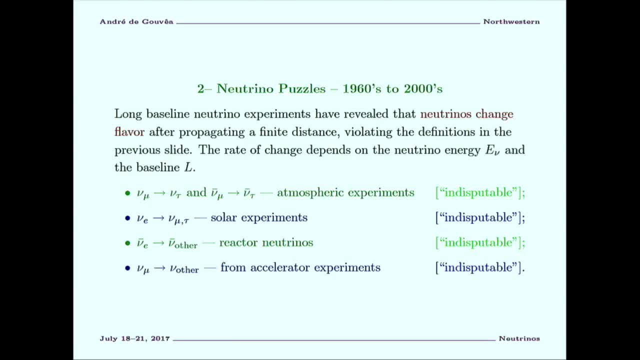 And I have 15 minutes more, unless I don't understand the oh. half an hour more. Oh, I have a lot of time, So you're in trouble. OK, But we have lunch at some point, Although I should ask you a question. 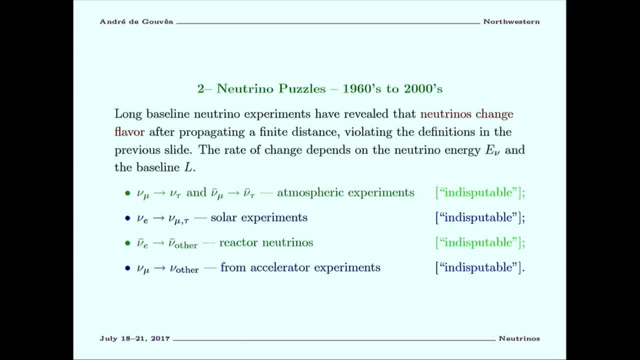 OK, But we have lunch at some point, Although I should ask you a question. Yes, do people have any questions? Yeah, Yeah, For that neutrino experiment. how do they distinguish the lines? Which lines were the real signal from the? 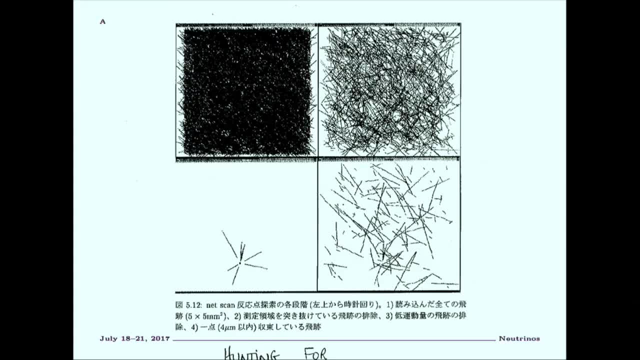 Oh here. So all the lines are signal. They're all due to other neutrinos that are going through the detector as well, And they just have a very, very good reconstruction algorithms. That means that they are really good at reconstructing the line. 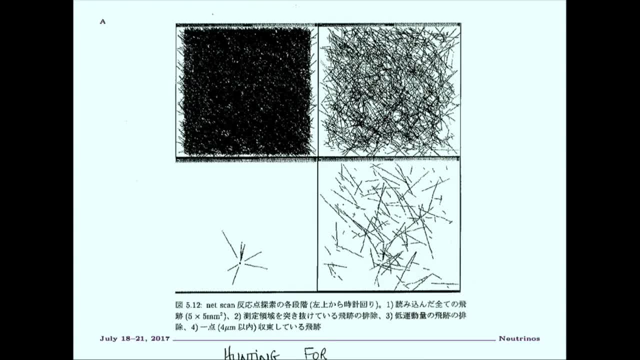 and then getting rid of it, And there's more things you can do. What they really look for are muons. So this is all about muons And, for example, in more modern detectors, what they will do is they will have a muon. 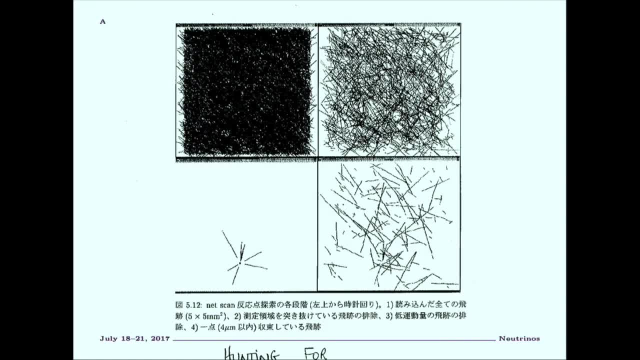 detector in the back. And then they will say: do I get a muon in my muon detector? If that's true, let me follow it back through this emotion detector and reconstruct that, And that will tell me which are the tracks I care about. 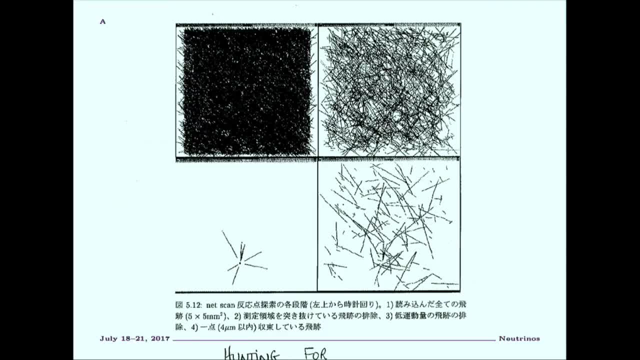 And that helps a lot. And then, of course, you have all these continuous tracks. You throw those out. Those are other weird stuff that's going on, And eventually they have this algorithm to solve this. There's a technological problem, which is: how do you do this in practice? 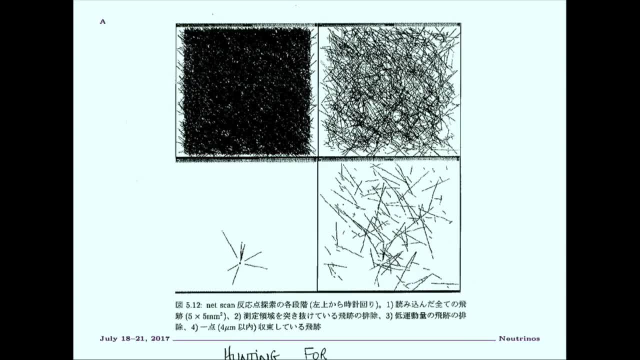 One way to do it is you hire a bunch of people and you make them do it for you, And that's how you did it until very recently. The big technological change was to teach the computer to do it efficiently and fast, And so effectively, efficiently and quickly. 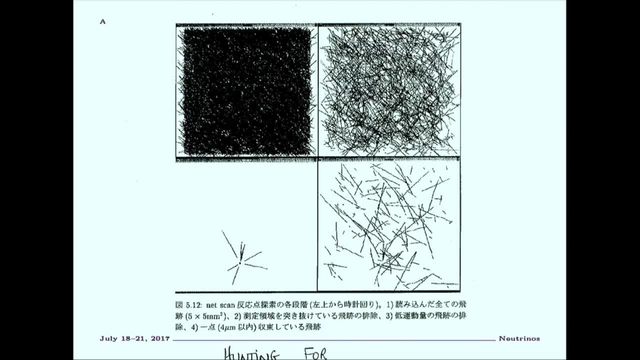 And they've developed it. They've developed it. They've developed these automated emotion scanning techniques that allow these experiments to actually exist in an even worse environment than this one. But yeah, it's an engineering marvel that this experiment works at all, And it works. 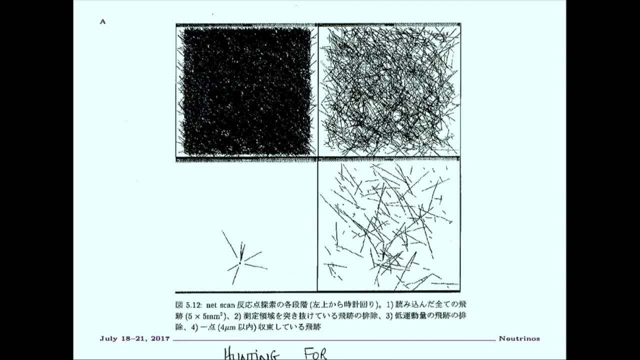 And I think people are convinced of that, And we don't have any new experiments that are out there that use this kind of technology, But people always wonder about whether we could do that, And in particular every time we talk about detecting TAUs. 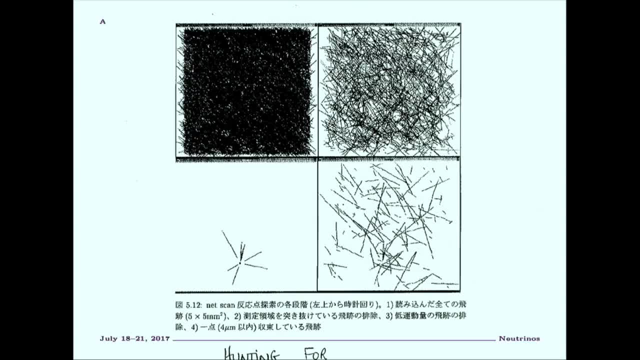 It's a big challenge because the TAU is a very annoying particle to detect in a neutrino experiment, because it doesn't look special. So you produce a TAU. it decays really quickly either into muon or an electron. 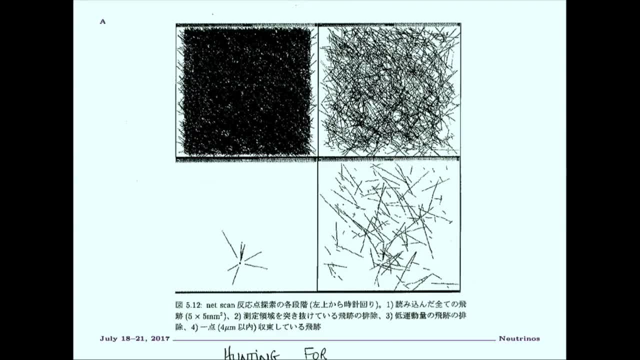 That's boring because the muon and the electron neutrino do this by themselves. They don't need a TAU in the middle Or they decay into pions and such, Which is good, because that's different. But that looks a lot like a neutral current process. 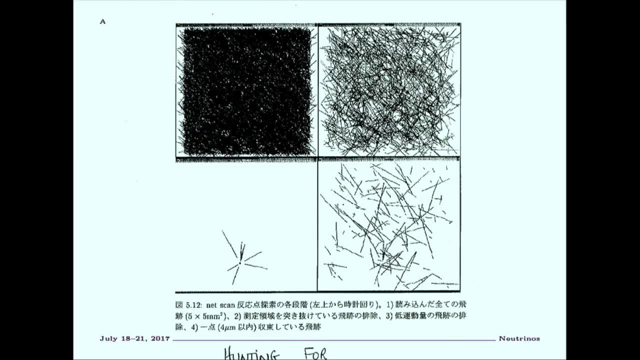 Where a neutrino does this. A neutrino comes in, hits a nucleus and emits a bunch of pions. So we don't have any good way of distinguishing other known phenomena from TAUs, except for the fact that this TAU lives a little bit and then decays. 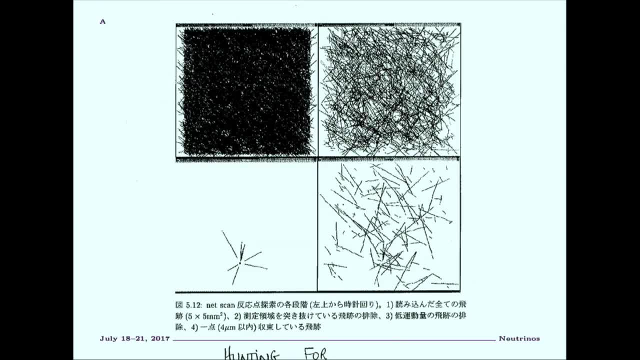 So you get this kink, But the kink is too small for you to resolve with other types of experiments, And the other issue you can do is you can try to do it kinematically, in a statistical basis, And the idea is the following: 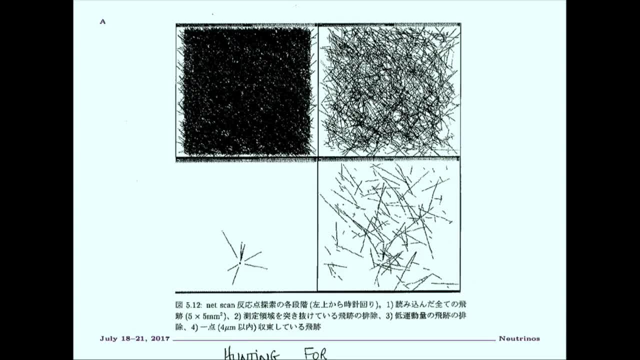 People try this: The NOMAD experiment at CERN, when they were looking for neutrino oscillations at much higher delta m squares. The idea is the TAU neutrino would come in, It produces a TAU And then the TAU decays to a muon. 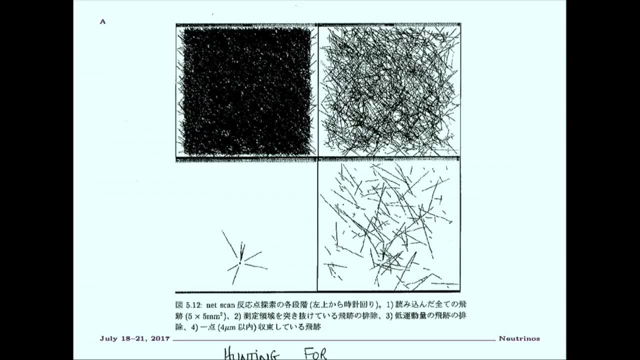 Now the way that could look different from a muon neutrino coming in and producing a muon is that if you follow this TAU path, the transverse momentum of the muon can be much bigger Because you're producing a TAU and the muon can get a big kick in the perpendicular direction. 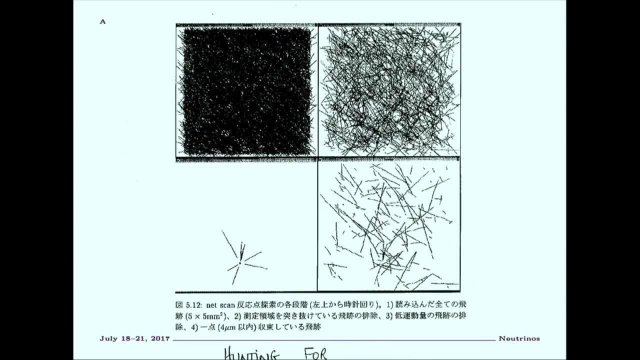 And you can't do that just by producing a muon because of energy momentum conservation. So by looking for high PT events you could get a sample which would have been enriched by the TAU neutrinos. They didn't see anything, by the way. 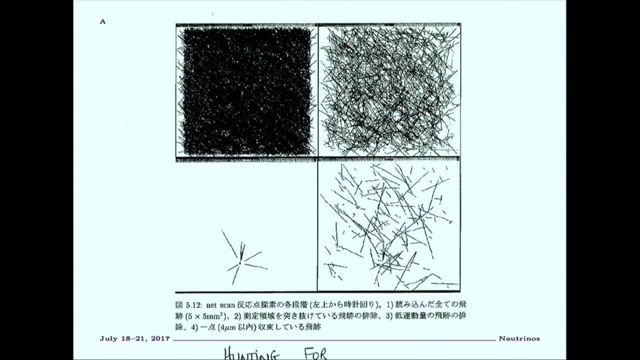 But that was the plan for that experiment. So statistically there's some good ideas. If you care about hydronic TAU decays. the TAU really likes to decay into row mesons because of this thing called the vector meson dominance. 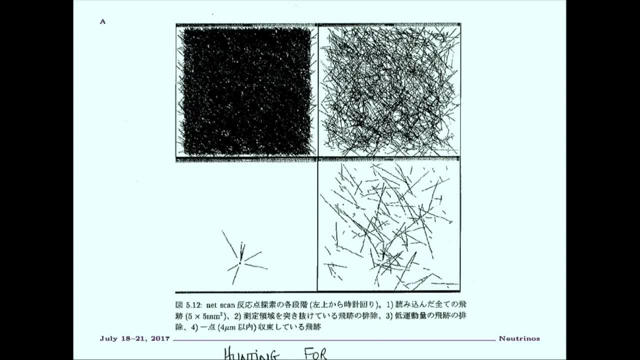 And you can see that. So that's one other handle you have. If for some reason you get an enrichment of row mesons in your neutral current sample, that might be a signature that you have more TAUs there than you have other kinds of neutrinos. 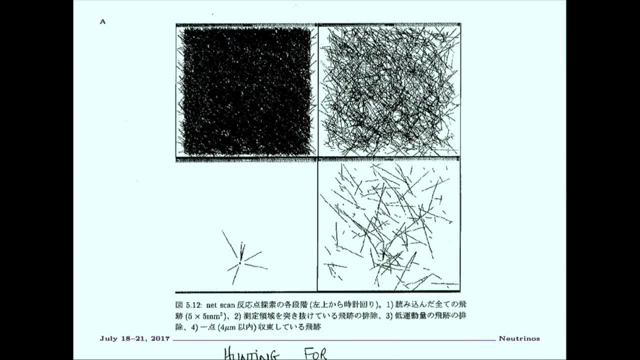 and so on, But it's still a challenge. We're not good at detecting TAUs. We're really good at collider experiments, or we're pretty good at collider experiments, But that's a totally different world. Collider experiments are really nice and you can see these beautiful they're called. 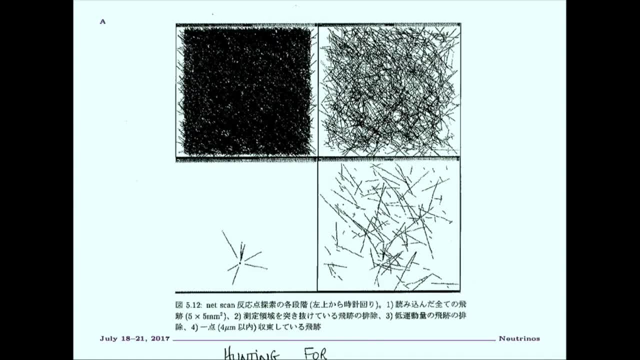 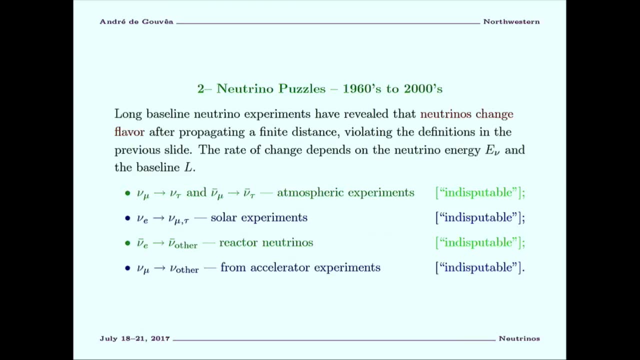 the TAU jets. They look exactly like a TAU is supposed to look, as opposed to a pion or something that hadronizes in some messy way. So other questions, OK. So let me start telling you about neutrino puzzles. 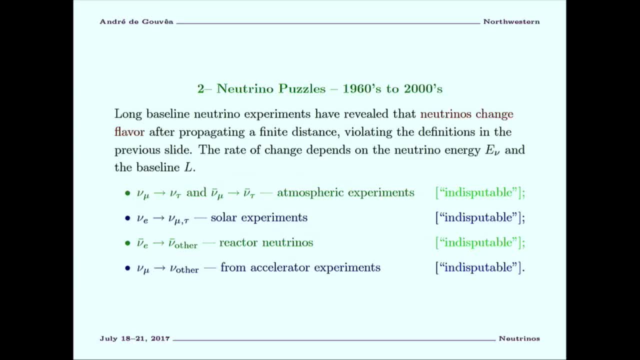 And that's the story which changed everything. And the idea is that people have figured out by doing experiments that if you produce a neutrino and you wait long enough before you detect it, it can actually change flavor and flight. That's what we figured out by doing experiments. 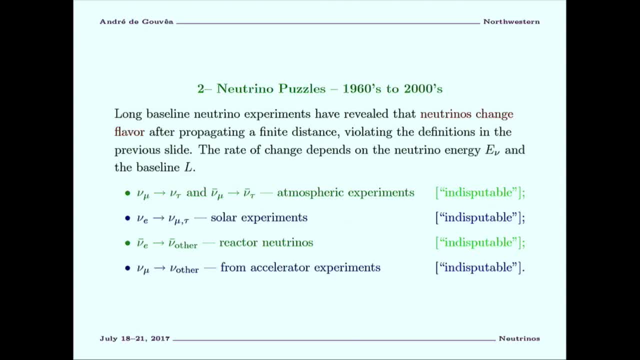 And the evidence for this is absolutely overwhelming. We have done experiments with different neutrino sources and we've done experiments with different neutrino energies and we've done experiments with different. We actually don't wait time, We just let the neutrinos travel a really long distance. 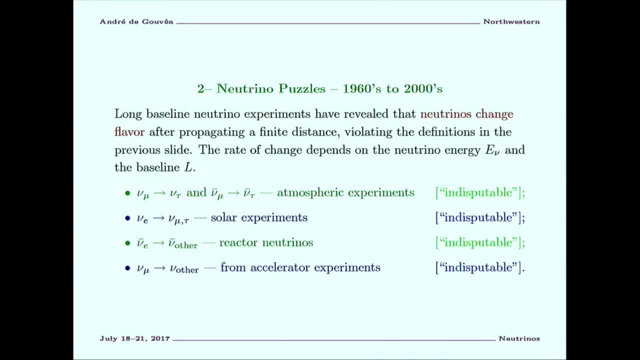 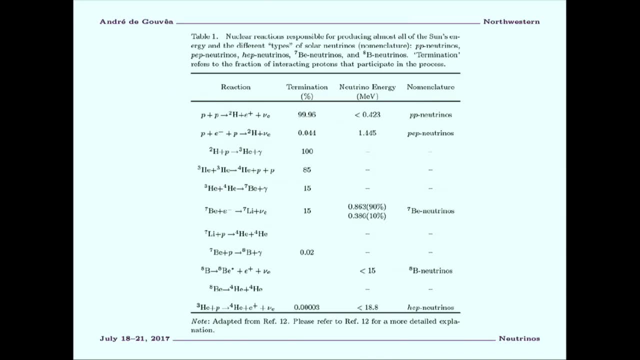 So this also changes the function of distance. So the evidence for this is really strong and that's what changed the way that we understand neutrinos, And I want to start telling you about this by talking about the solar neutrino problem. It's a very old problem. 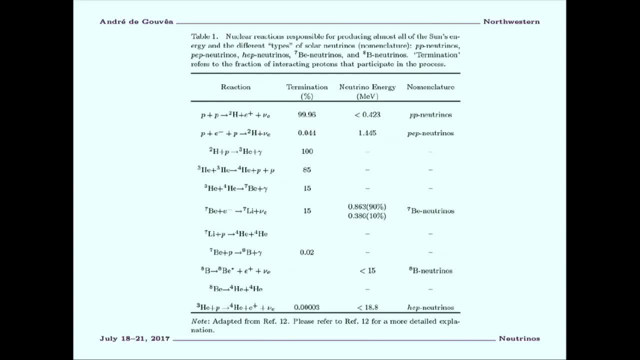 It's very important to remember that the Institute played a huge role in understanding solar neutrinos. This is the work of John Bacall, who was a big nuclear theorist, was done almost all of it here, And he was somebody who set out to try to understand how the sun works. 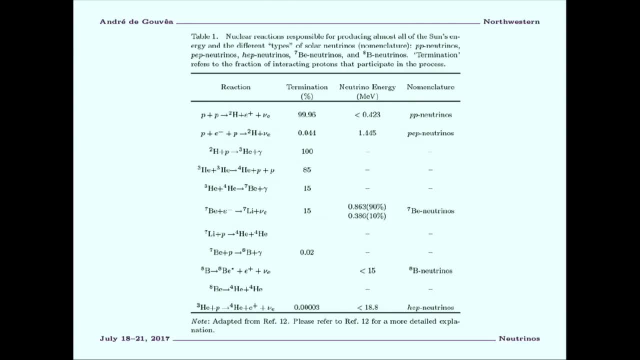 And the sun works, as you know, by nuclear reactions, So there's a lot of temperature pressure and so on, And people figured out that this is what's going on in the sun all of the time. And this is what you learn in grade school, or whenever it is. you learn about this, hopefully. 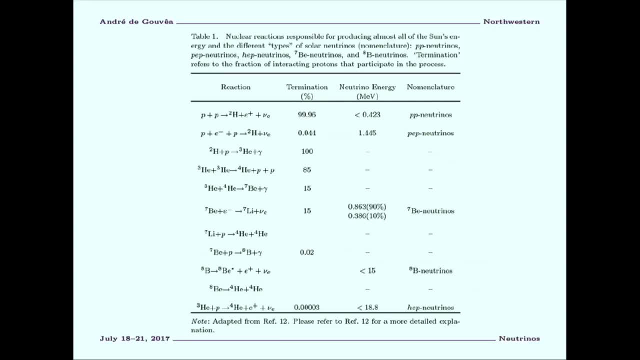 high school. So the sun shines by proton fusion. So there's enough protons there and enough heat to make two protons ultimately combine into helium-4.. So you're taking two protons. 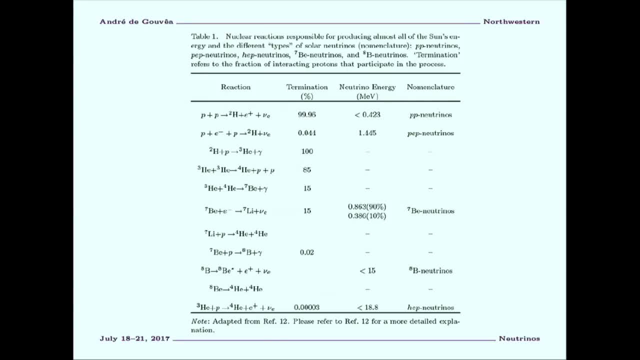 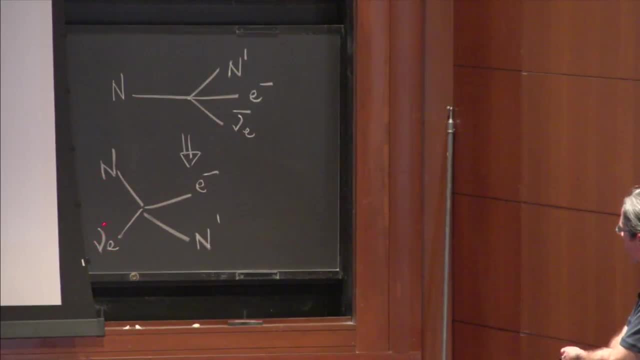 You want to look for an electron neutrino hitting a nucleus and producing an electron. Your signature is an electron- And of course, you want to do this with a material that doesn't undergo beta decay by itself- And again, this will become important later. 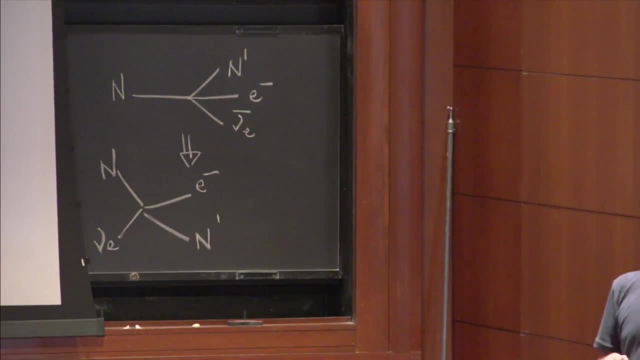 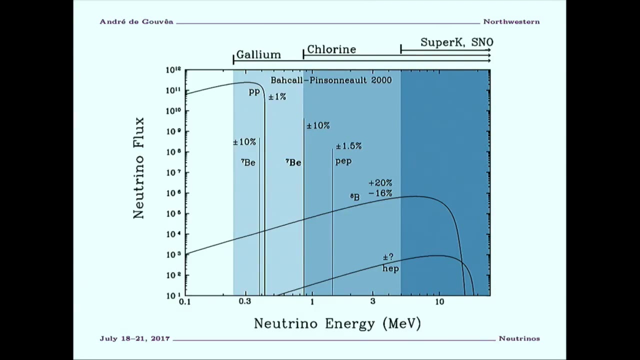 because if this undergoes beta decay by itself, you're in trouble because you have all these beta decays happening inside of your experiment at the same time, And this is what people set out to do. And actually the first experiment, the first two experiments, 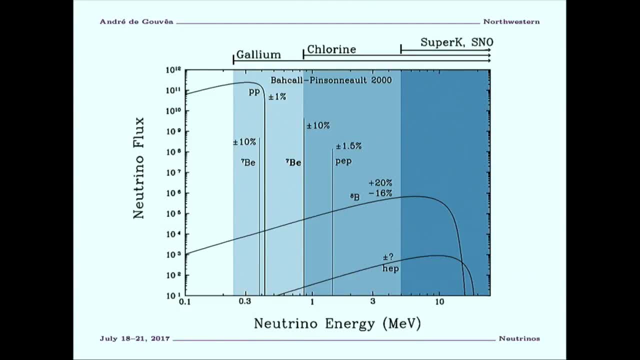 this is this chlorine experiment. They decided to do something different, which is, instead of looking for the electron, you looked for the nucleus that you're producing. So the idea for the experiment is very simple: You take a lot of chlorine, you put it deep underground when you're very far away. 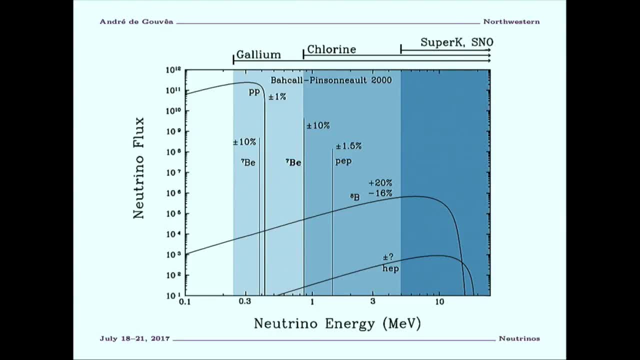 from cosmic rays and other radiation and stuff. and then you wait for a solar neutrino to come in and convert a chlorine nucleus into argon. it turns out Argon is great because it's a noble gas. That means that if you produce argon, 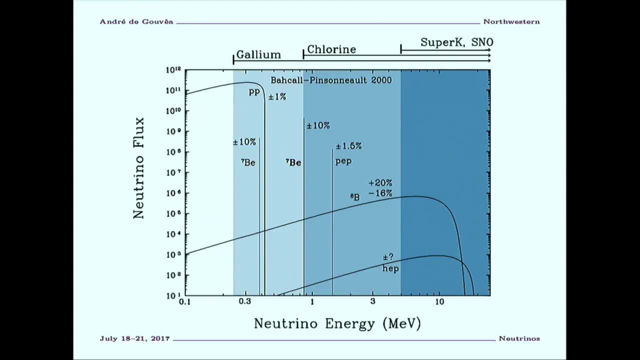 out of your big chlorine tank. it's just going to sit there, And then you wait a long time for this to happen enough, and then you take your big vat of chlorine and then you look at it and then you see how much argon you have produced. 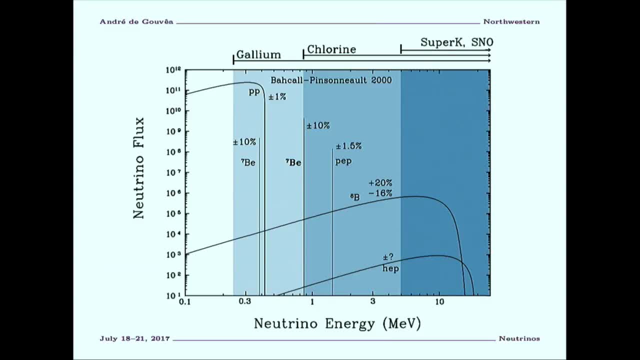 That's the plan. It's a totally crazy plan because the amount of chlorine that you need is gigantic. That's where we get into this era of experiments that have masses measured in kilotons. Okay, so it's a big, big vat. 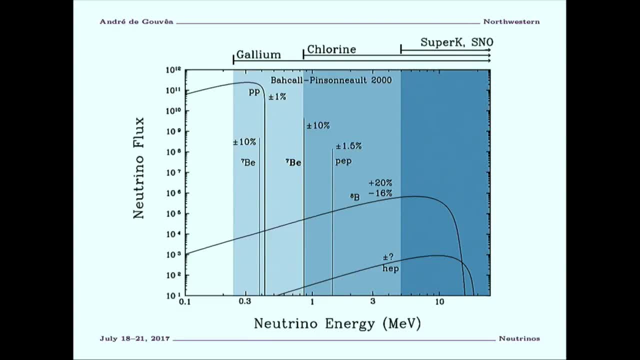 of chlorine which was taken to a gold mine in Homestake, South Dakota, And the signal that you're looking for is really small. Again, what they would do is that they would expose the chlorine for about a month. they would take it out. 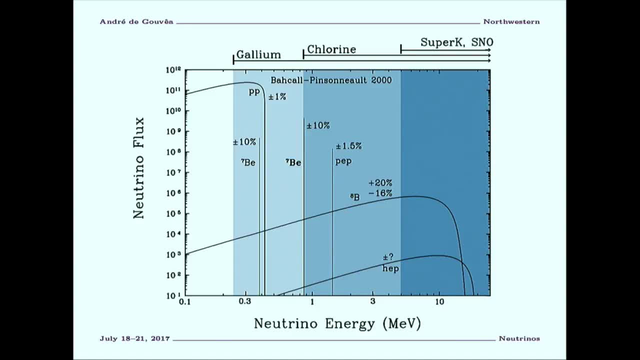 and they would look for something like tens of argon atoms inside of this big vat of chlorine. That's the experiment. It's a very difficult experiment. It involves a lot of chemistry, which makes it very, very hard, And somehow people did it. 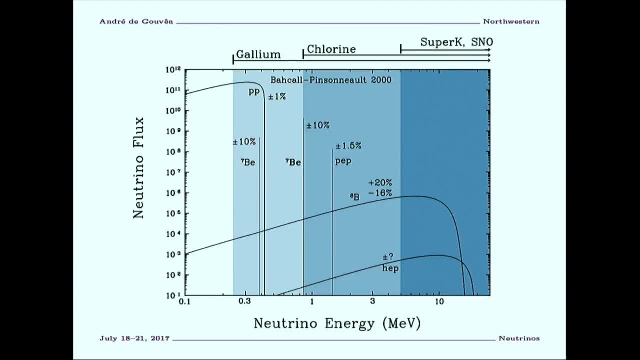 So they actually managed to do the experiment and they managed to see these argon atoms and they've established that they can see neutrinos coming from the sun. That's a Nobel Prize-winning experiment, by the way. just for seeing the neutrinos coming from the sun. 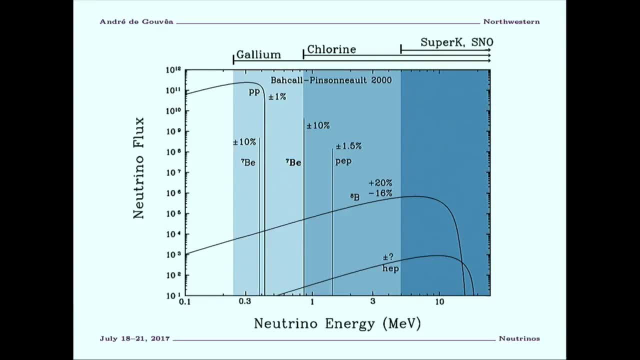 to Ray Davis. This is the chlorine experiment, And this experiment was a great success, except for the fact that we knew how many neutrinos we were supposed to get And they were off by about a factor of three. So they saw a factor of three less neutrinos. 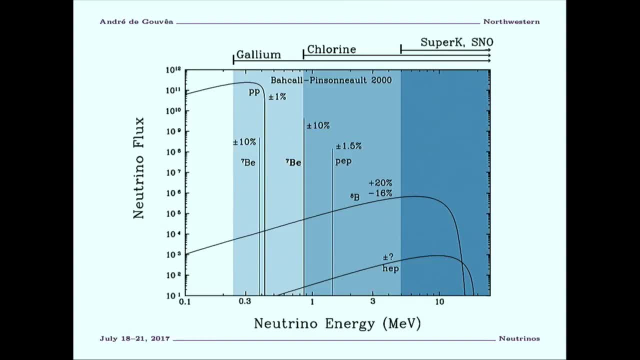 coming from the sun than they expected. This is in the 1960s And, of course, when this result came out- and I don't know, because it wasn't there, but I can predict that what happened was people said: great. 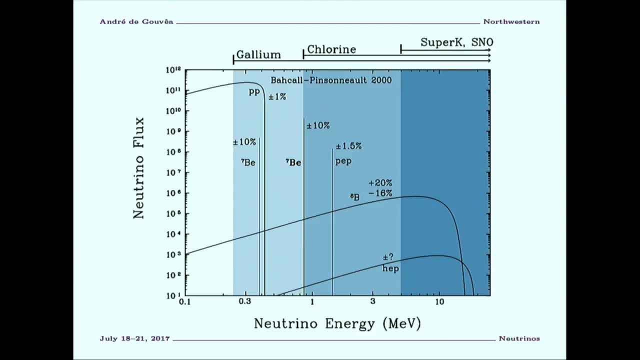 we know neutrinos are coming from the sun. this is a great measurement. It's off by a factor of three, but who cares? I mean, it's a really hard calculation because you have to understand how the sun works in detail. 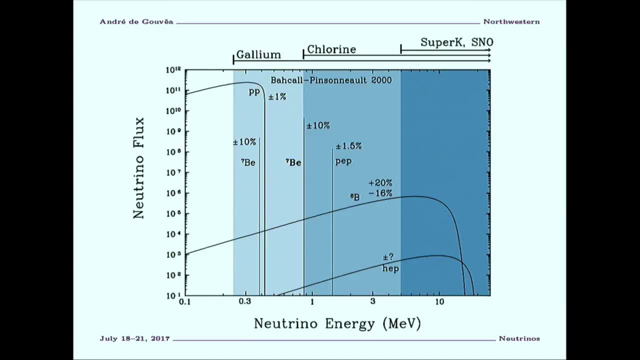 and you're doing this crazy experiment where you're counting atoms in this gigantic vat of chlorine. By the way, chlorine is like cleaning fluid, It's not very sophisticated. So the fact that you're off by a factor of three- ah, factor of three, that's not so bad. 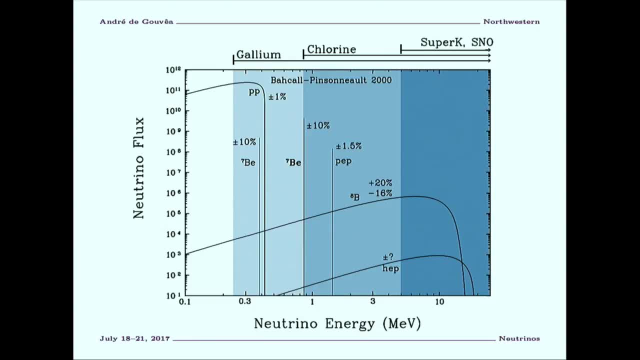 This is in the 1960s. The experiment continued for many, many decades. I mean the experiment stopped running in the early 2000s And they confirmed this factor of three and the calculations were refined. There's a lot of criticism of how the calculations were done. 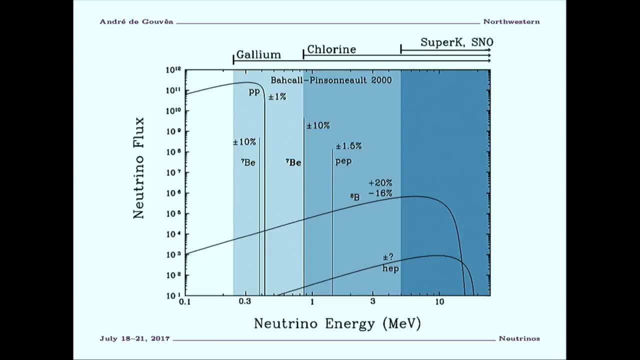 Maybe these models for the sun were just wrong in some interesting way, and so on. So in order to resolve that, people built a different kind of experiment. These are gallium experiments. It's exactly the same idea: a large volume of gallium. 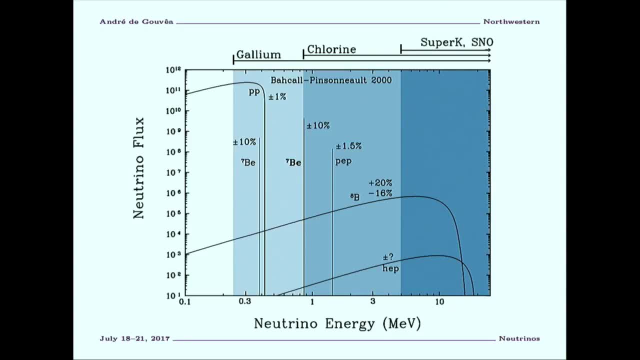 that's converting into germanium. And then there's some clever technique of identifying how much germanium you've produced, And the idea is: oh, I should have said this: the argon that you produce is radioactive. That's good, because you can see. 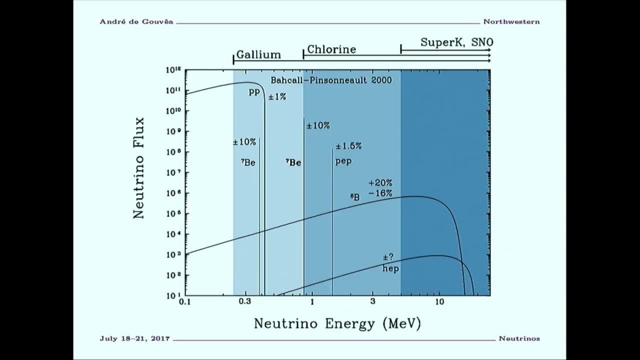 the radioactivity coming from that. The same is true of the germanium that you produce. That's kind of how you see these atoms. So this gallium experiment was also done. And the nice thing about the gallium experiment, which I didn't explain. 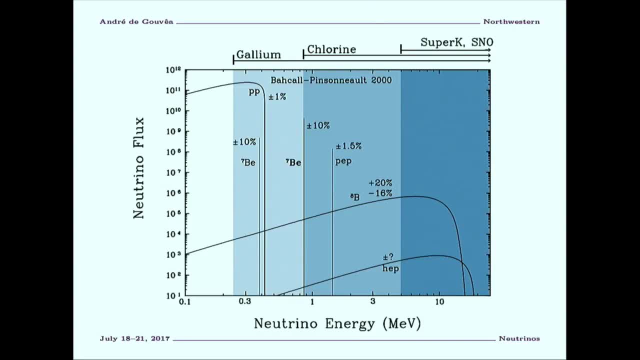 so these lines here show the threshold of the experiment. In the case of the chlorine experiment, if the neutrino has less energy than that, then the reaction doesn't go. It's not kinematically allowed With the gallium experiments, it's the same. 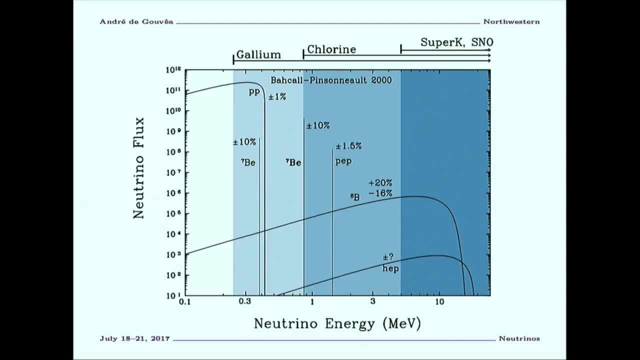 It has a threshold, but the threshold is a lot smaller. And this was very important because with the gallium experiments you could see this gigantic PP neutrino flux. So that's why these experiments were built for was to check whether the result 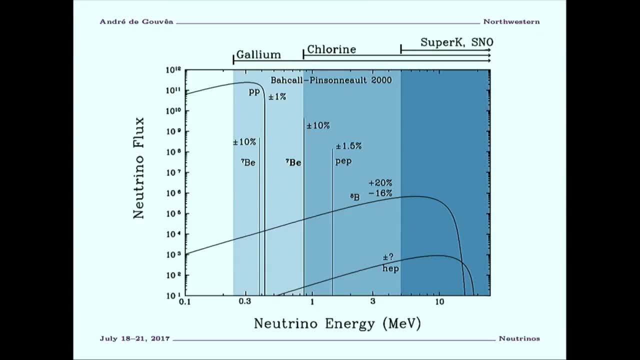 of the chlorine experiment was correct And they were also sensitive to the PP neutrinos. and they were sensitive to the PP neutrinos. Sure enough, when they do these experiments, they also see fewer neutrinos than they anticipate by a factor of two. 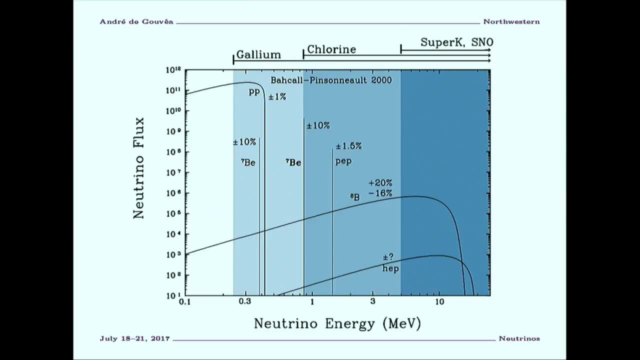 Finally, at around the same time that the gallium experiments were coming on, we had these really big water tanks that were built underground to look for proton decay And somebody figured out: hey, we can do solar neutrinos with that. It has a much higher threshold. 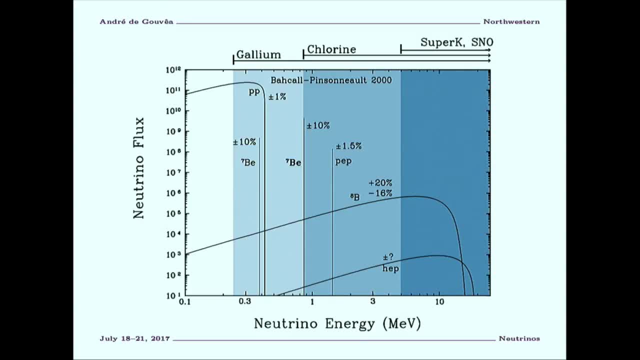 It works on water, And what you're basically seeing is electrons scattering on the electrons in the medium, And you can convince yourself of why that's true. First of all, electron neutrinos- don't know how to do charge current scattering off of protons. 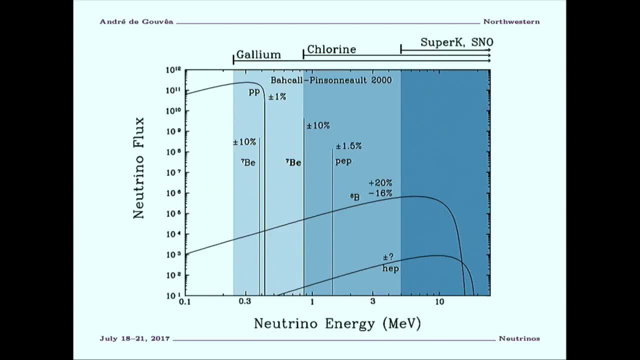 It just doesn't work. at low energies It's not possible. So if you don't believe me, just try. You'll see that you violate lepton number if you try to do that, Or you have to produce a delta plus plus resonance. 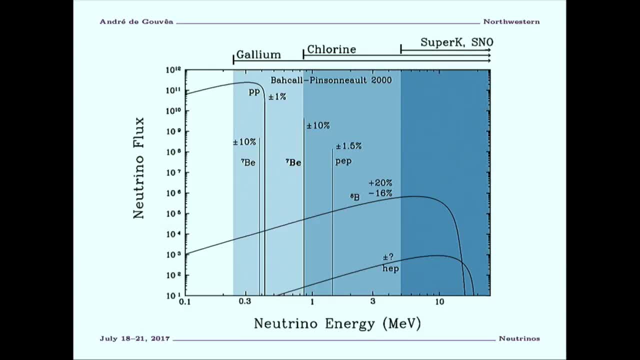 which takes a lot of energy. so you can't do that. And electron neutrinos can't really interact with oxygen either, because the oxygen is a very, very tightly bound nucleus. It's a doubly magic nucleus, if you remember what that means. 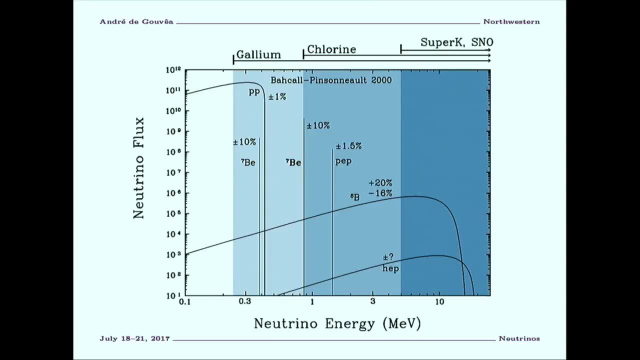 If you don't know what that means, you should look it up. But oxygen is doubly magic, So they have to talk to the electrons. And again, this large water. Cherenkov experiments also see a big depletion of the flux, So don't look at the last part of the plot. 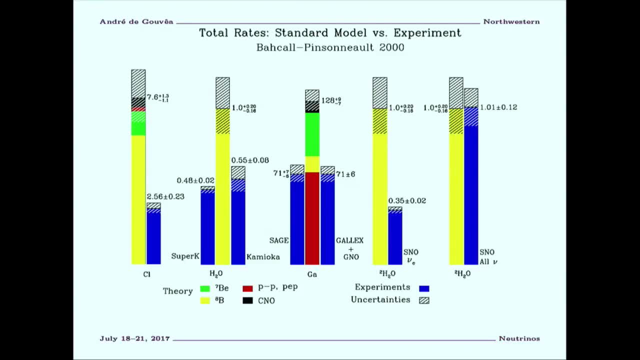 This is a colorful plot and all you want to take from this is the blue lines are the measurements of the neutrino flux in some weird units. In case you like ancient history, these were measured in a SNUs. These are solar neutrino units. 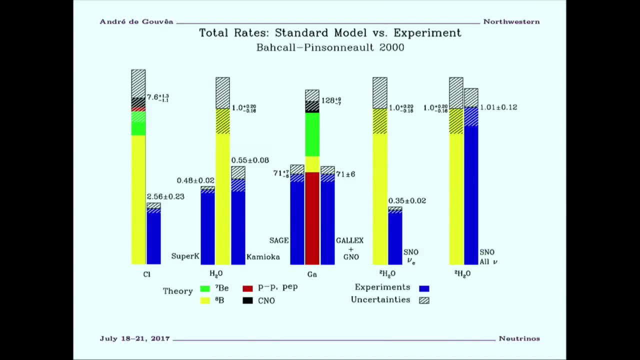 So the flux for the chlorine experiment was 7.6 SNUs- This is true, by the way, I'm not making this up- And the measurement is 2.56, same units. So this is the chlorine experiment, This is the water experiments. 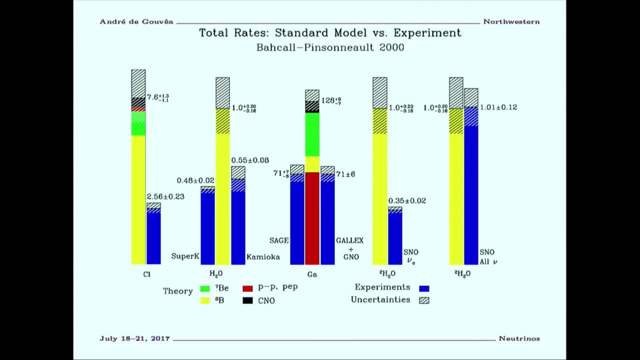 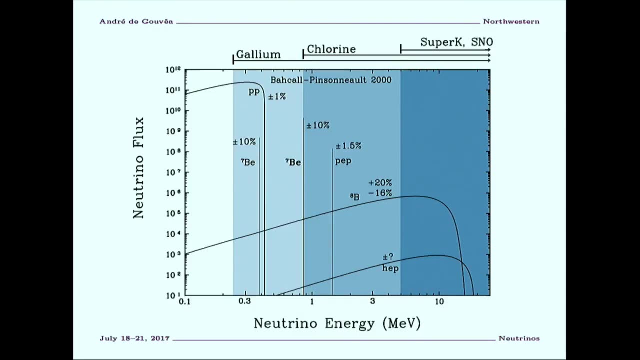 They expected this much and they got half. These are the gallium experiments. They expected this much and they also got half. What the colors here indicate is where the neutrinos are coming from that contribute to this particular flux. So the boron-8 neutrinos. are these neutrinos over here? 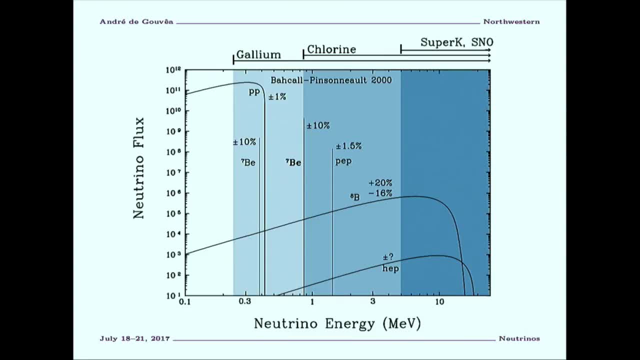 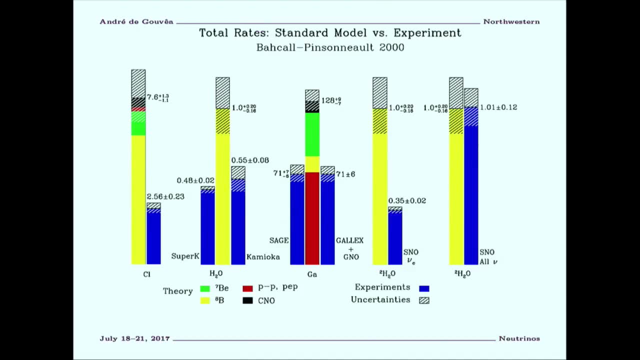 from boron-8 decays. The PP neutrinos are these guys, And then you have these lines which are mostly beryllium-7.. So you notice that all of these experiments see a big depletion of the number of neutrinos. 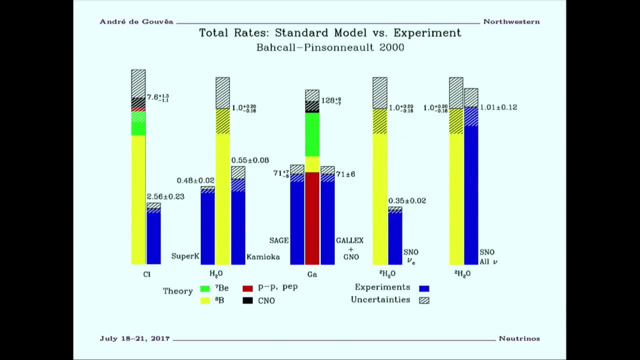 that you expect, And in order to resolve this problem, we had to build a new experiment that made measurements that look like this, And I'm not going to talk about this today, but I'll start talking about this tomorrow. This is a snow experiment. 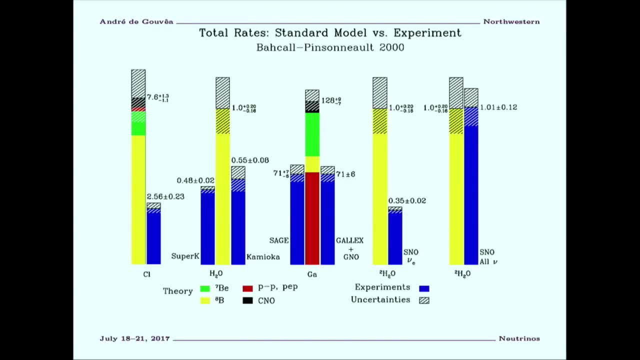 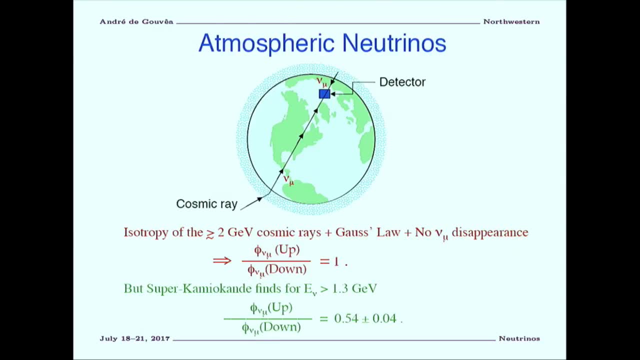 that actually solved the problem for us. But this is where we were at the end of the 1990s And I'm not going to talk about the snow experiment now. but since I'm here, I'm trying to do some time management here. 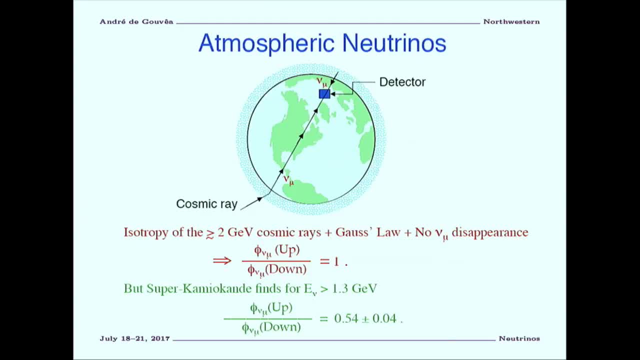 The other puzzle that people ran into was with neutrinos produced in the atmosphere. This is important because we still care about these neutrinos today, And the idea is very simple: They're cosmic rays hitting the atmosphere all the time. People learned that more than 100 years ago. 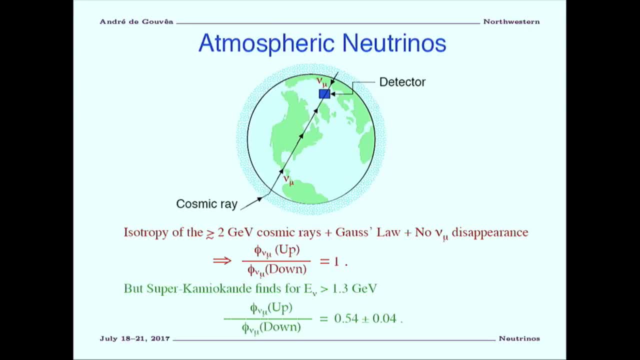 And these cosmic rays. when they hit the atmosphere they produce particles, mostly pions, Pions and kaons. a little bit of charm. People do research on that. But if you produce a lot of pions then the pions will decay. 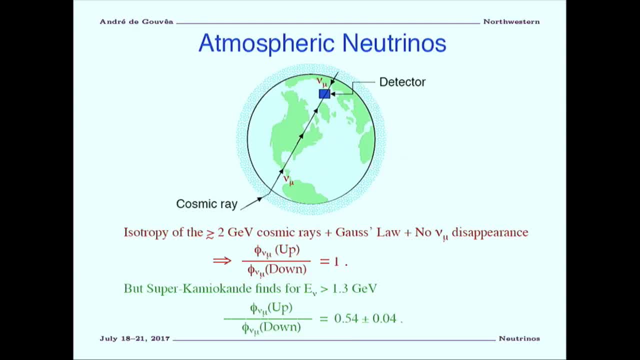 and the pions decay mostly into muon neutrinos. That's what we care about Now. the muons that are also produced in pion decay will also decay some of the time And they decay into again muon antineutrinos. 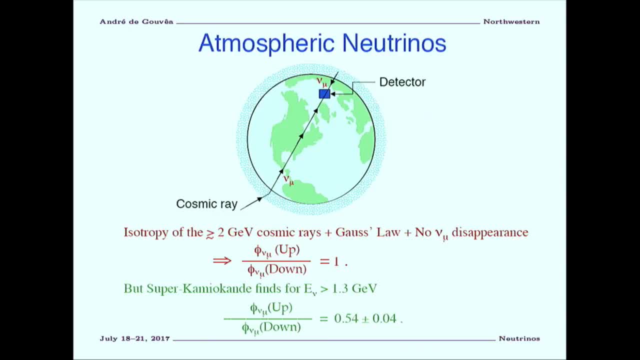 electron, neutrinos and electrons. So you have a flux of neutrinos coming all the time bombarding the Earth. So that's the atmospheric neutrinos, And they have lots of nice properties. One really nice property is the following: That's what's depicted here in this picture. 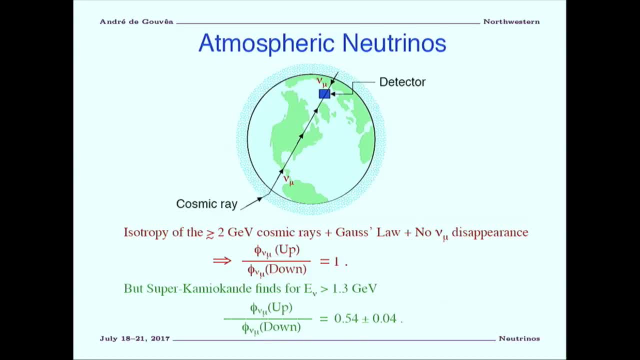 If you put a detector underground, we should be so lucky we could go this deep. But if you put a detector underground and you ask how many muon neutrinos do you get from some solid angle on top of you, And then you compare with how many neutrinos you get. 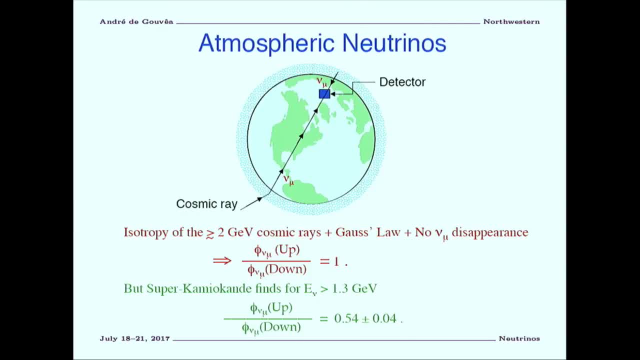 from the same solid angle in the opposite direction. So you look at the neutrinos coming from above and you look at the neutrinos coming from below. You can convince yourself very quickly, using the fact that we live in three dimensions, that the number of neutrinos that come from below 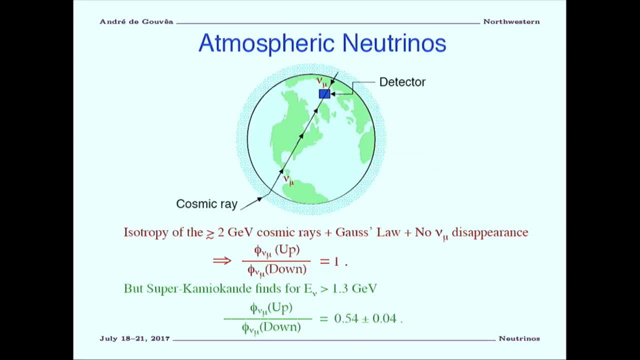 in the same solid angle is the same as the number of neutrinos that you should get from above. That's a very, very simple prediction that you can make. that only depends on geometry And it only depends on the fact that the number of neutrinos- again 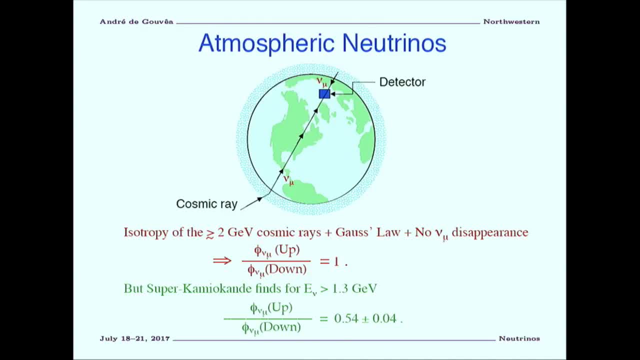 that gets absorbed by the Earth is ridiculously small, So you can neglect that. So if you believe in those two things, which only rely on geometry and the weak interactions being very weak, then you expect the number of neutrinos that come from above to be exactly the same as the number of neutrinos. 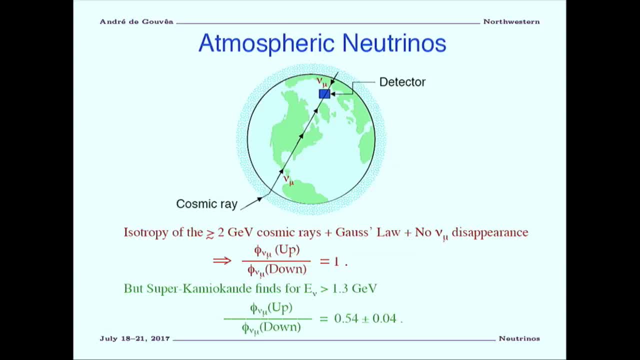 that comes from below. That's a very, very simple prediction. So you wanted to measure one, And one manifestation of this experiment is the Super-Kamiokande experiment. They measured this ratio and they got it right. It's actually about a half. 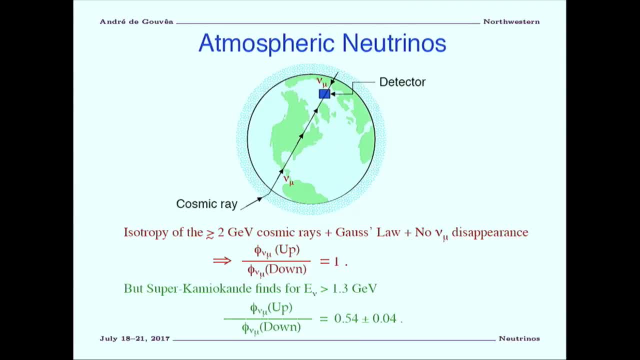 with a very small error bar. So they find out that the number of neutrinos coming from below is actually about a half of the number of neutrinos that are coming from above. Now, from a historical point of view, it's interesting to think about these experiments. 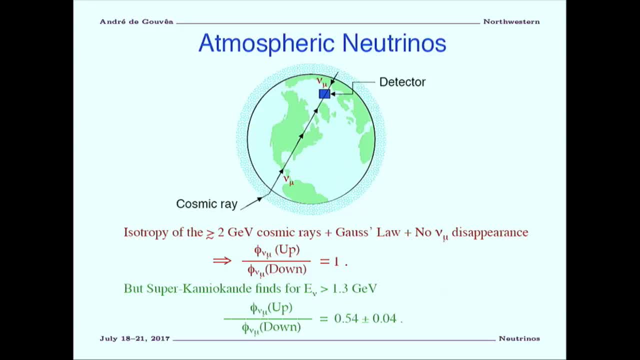 And, like I said, the first generation of this in Japan is the Kamiokande experiment. There was also an experiment in the US called the IMB experiment, And these were not. these were not neutrino experiments, These were proton decay experiments. 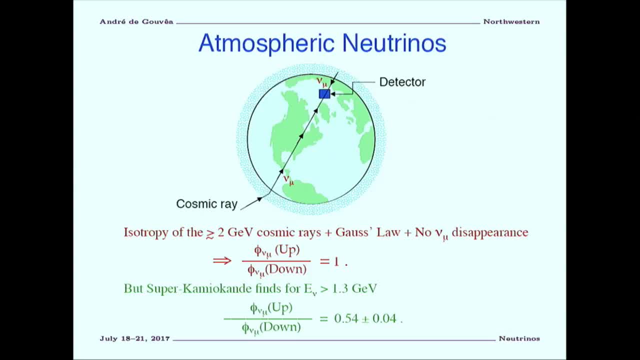 Okay, and if you don't know this, I'm sure you've heard about Super-Kamiokande And you might have asked yourself: what does this mean? And you probably said, oh, I don't know what it means because I don't know Japanese, for example.